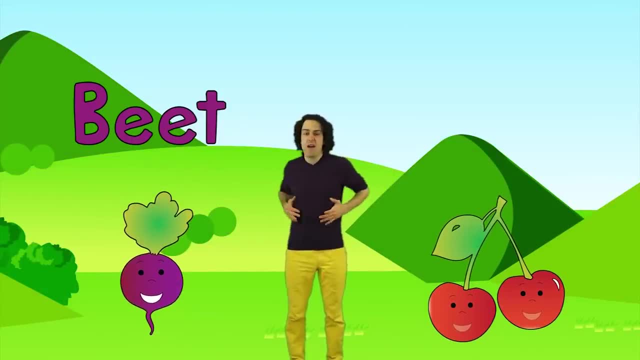 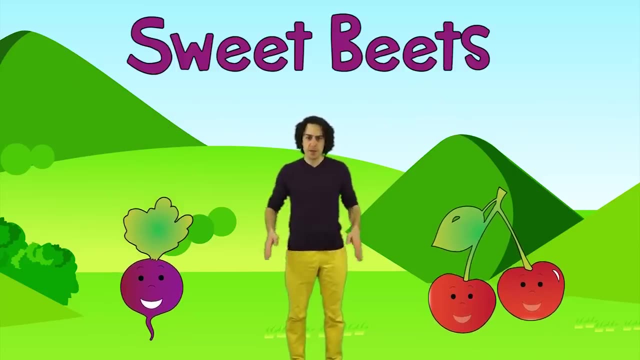 You made it Great. I'm here having lunch with my friend Beat and my other friend, Cherryes. Beat and Cherryes and I are going to play a song called sweet elementary beats. All That's all about playing the rhythm. We're going to play most of the rhythm on our legs like this: 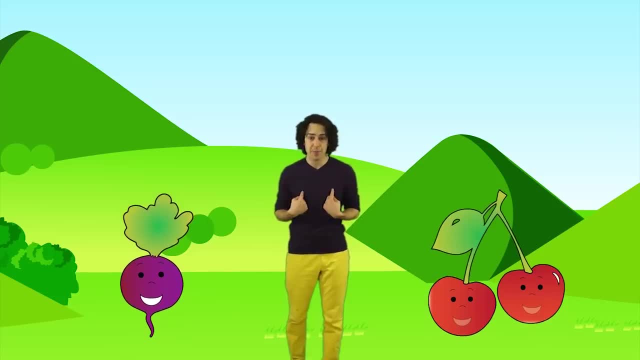 Now, this song is a call and response, which means I'm going to say something and then Beat and Cherry and you guys are going to repeat after me. Why don't we try a quick warm-up? So listen first and then you try it. 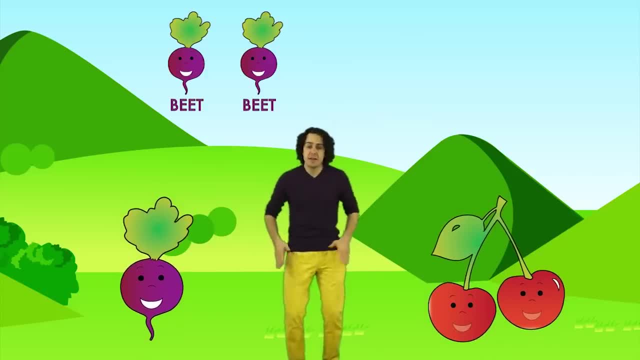 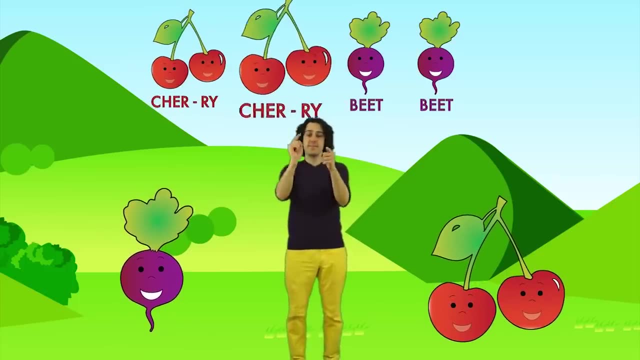 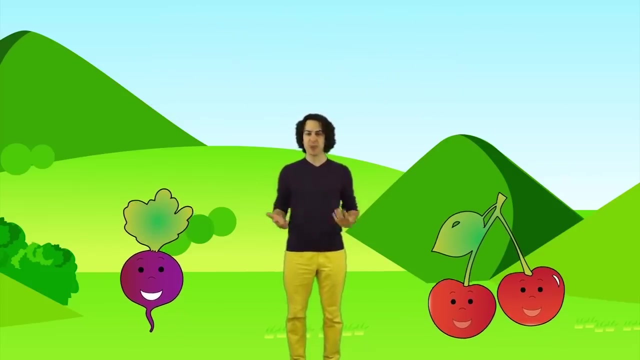 Here we go: Beat beat Cherry, beat, Beat beat, Cherry beat, Cherry Cherry, beat beat Cherry, Cherry, beat beat. Hey, that was pretty good, Nice job. So without further ado, let's play Sweet Beats. 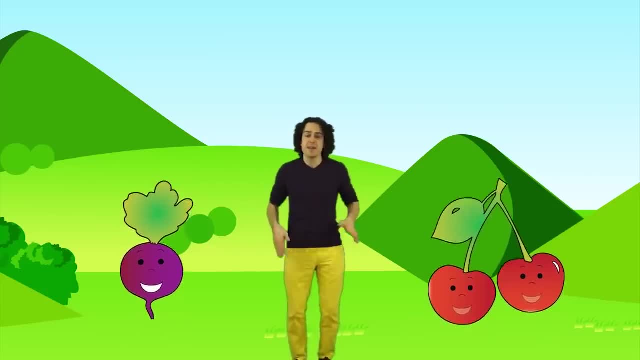 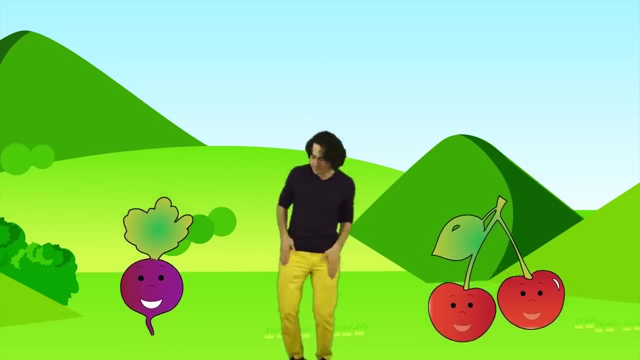 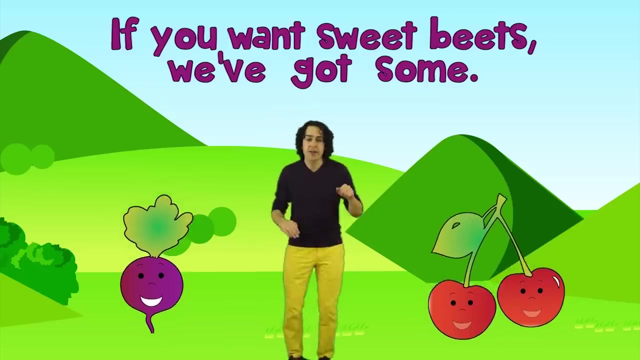 So let's tap on our legs. This is how we keep the beat nice and steady. That's it. You can play with two hands, or you can try going back and forth between your hands. So the song goes like this: If you want sweet beats, we've got some. 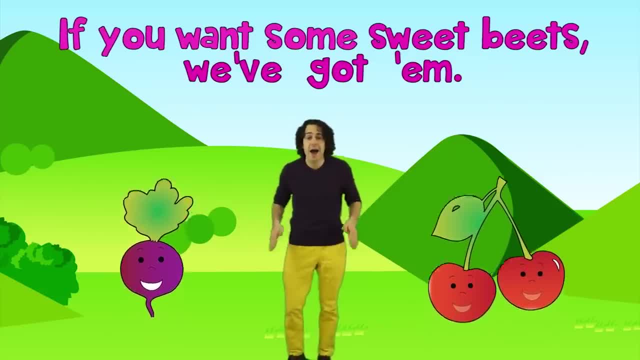 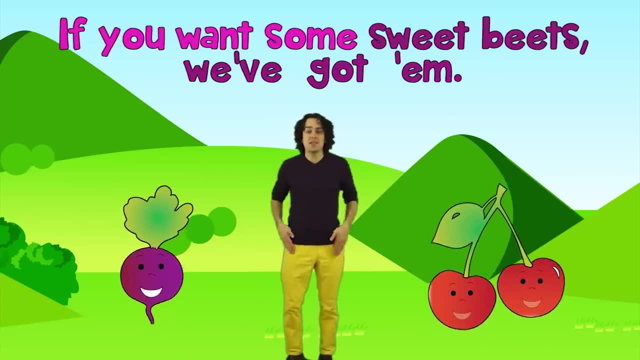 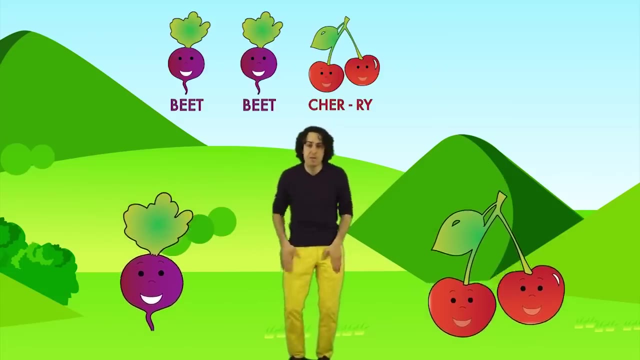 If you want some sweet beats, we've got them. If you want sweet beats, we've got some. If you want some sweet beats, we've got them. Repeat after me, Here we go: Sweet Beats, Sweet Beats, Sweet Beats. 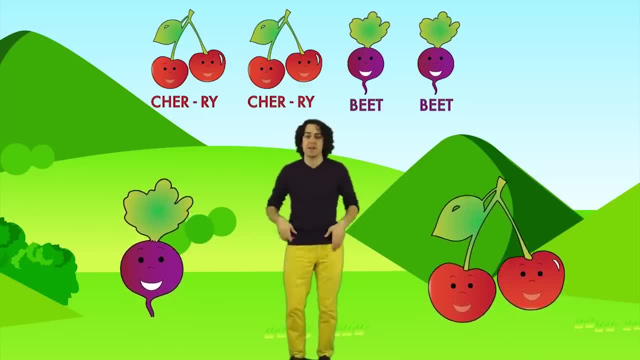 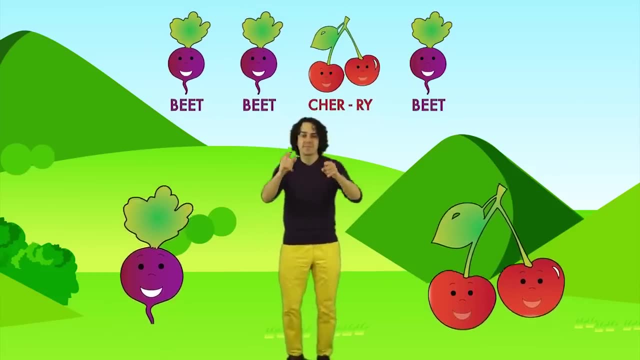 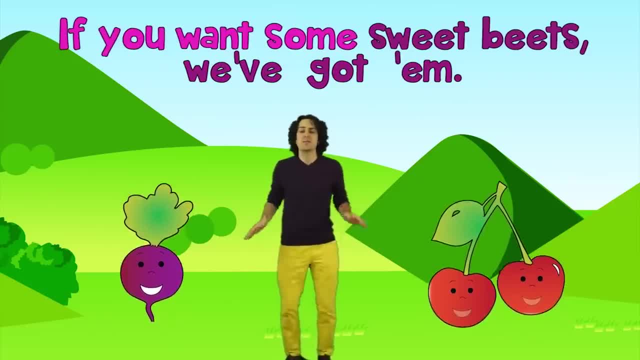 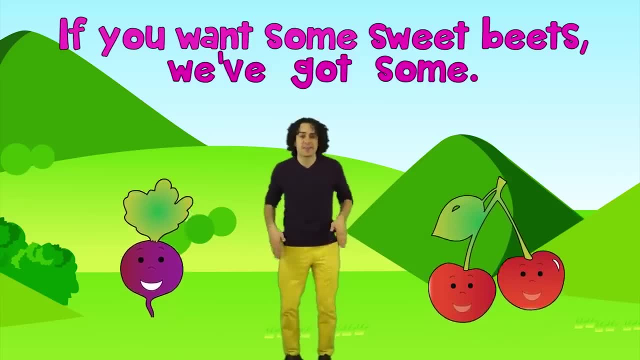 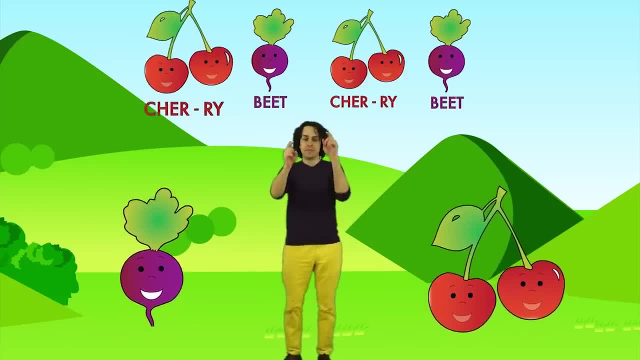 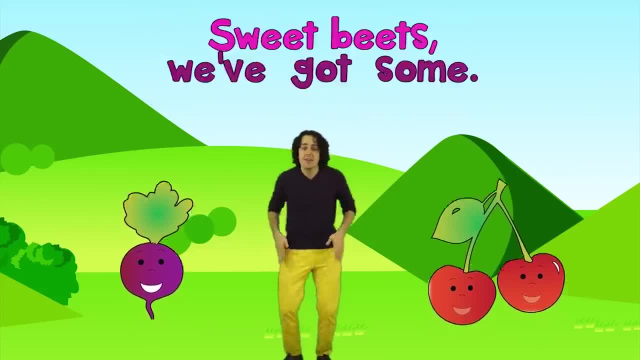 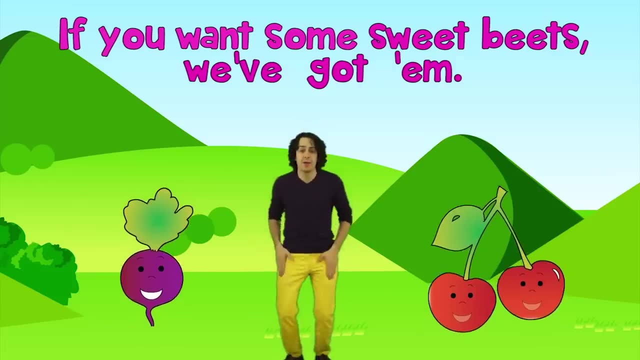 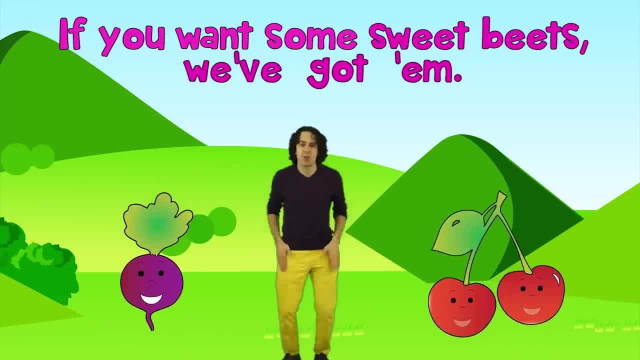 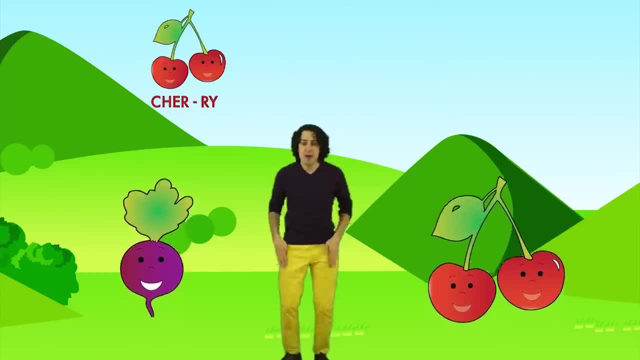 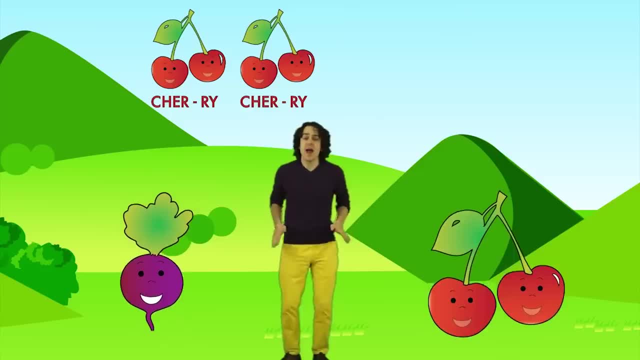 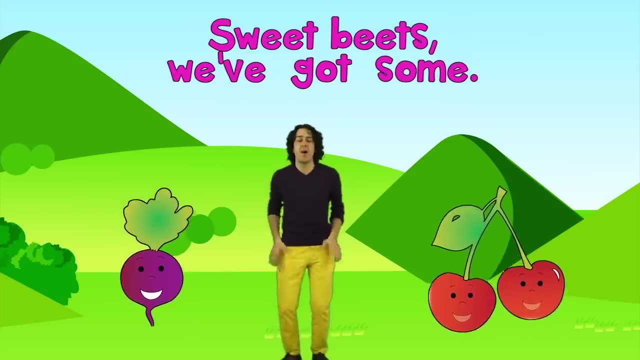 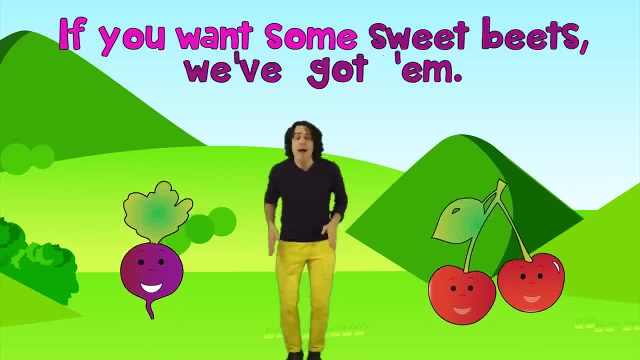 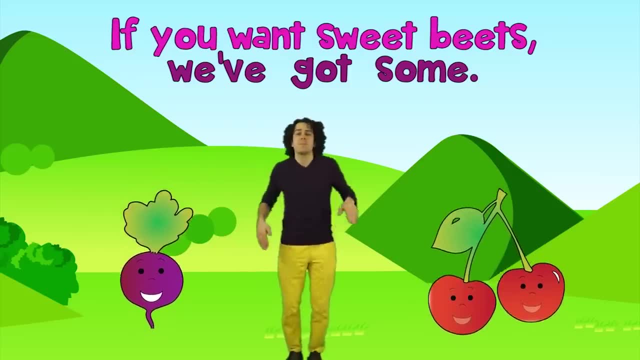 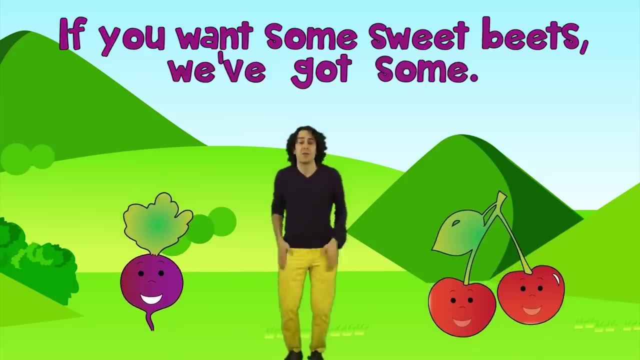 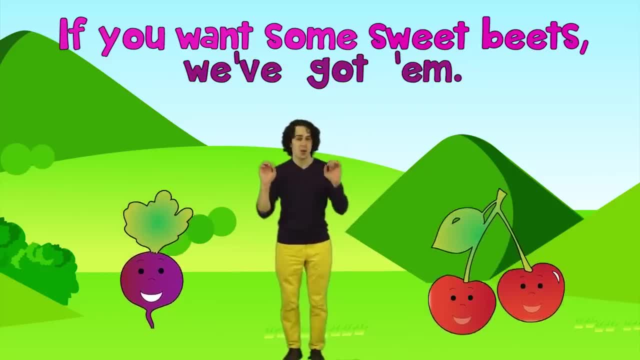 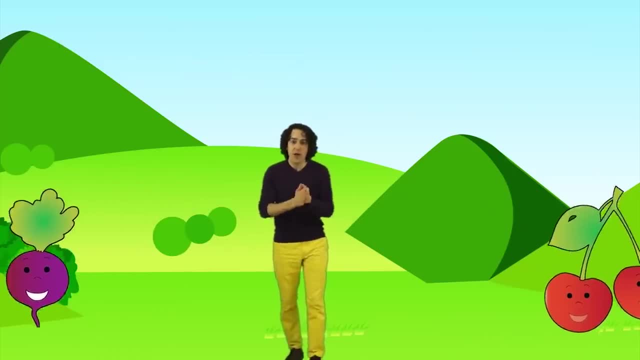 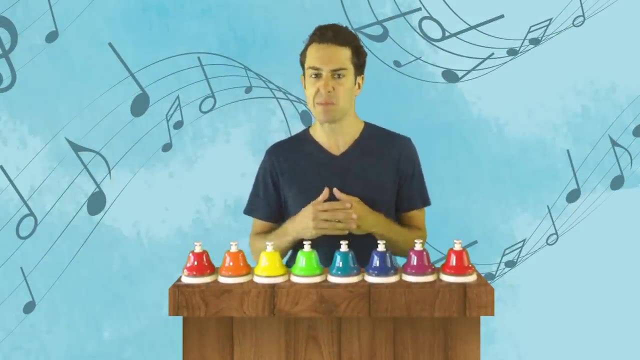 And if you want some sweet beats, we've got them. Hey, Nice job, Great job following along. That was a lot of fun. Hello again, and nice work with sweet beats. Sweet beats is all about rhythm, which is musical timing. 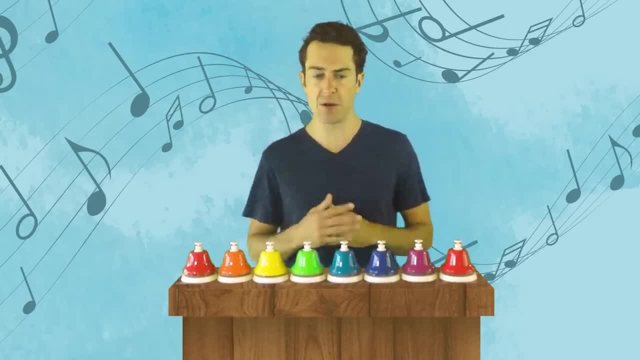 but in the next video we're going to talk all about pitch, which is how low or how high we sing different musical notes. To do this, we're going to meet eight different notes and eight different hand signs for each note. Getting the hang of these hand signs might take you a little while if you've never seen them before. 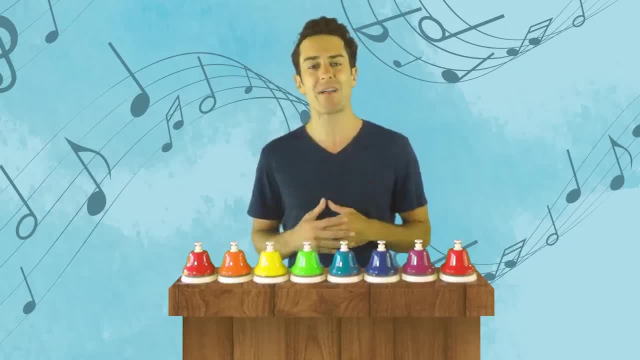 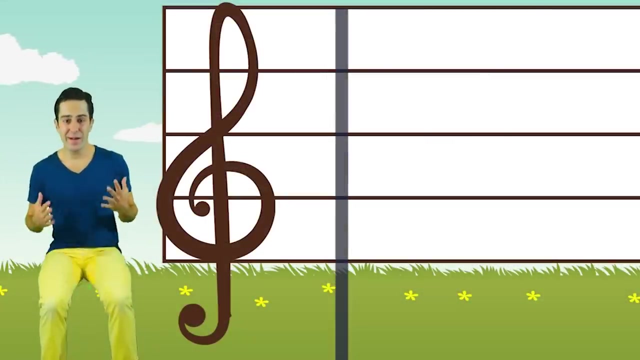 and we do go into a lot of detail inside of the Prodigy's Playground about the hand signs. For now, though, try singing and hand signing with these two hand signs. Short and sweet episodes of PSP Melodies. Hey everyone, and welcome to the very first episode of PSP Melodies. 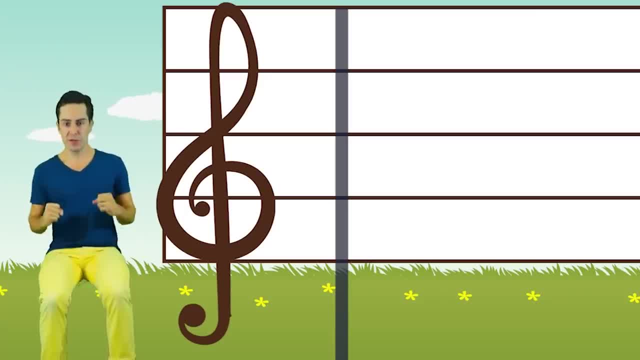 Today we're going to be singing the C major scale, going up using the solfege hand signs. We'll start out nice and slow and then we'll speed up as we go through it And when the music hits the line over here, that's when you're going to sing and hand sign. 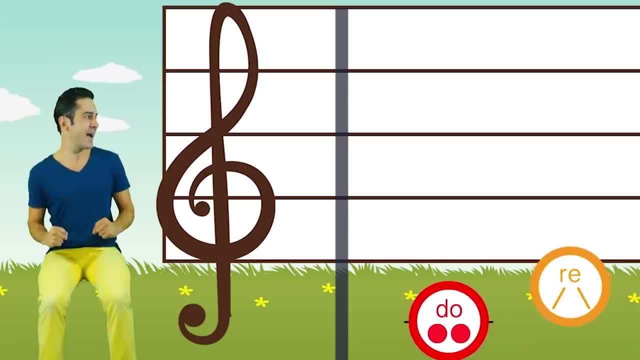 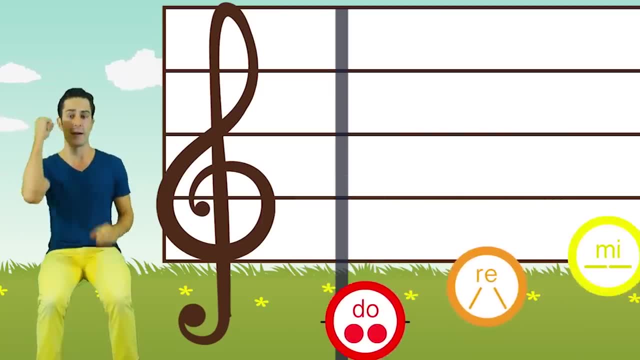 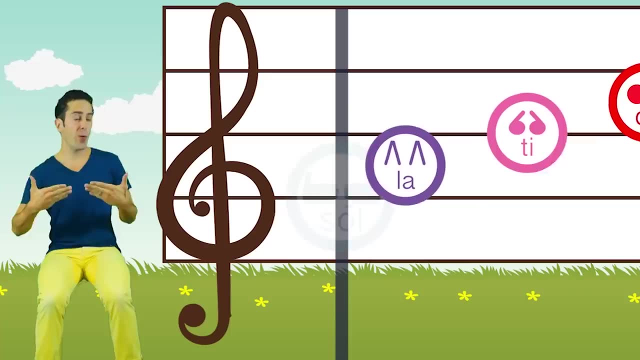 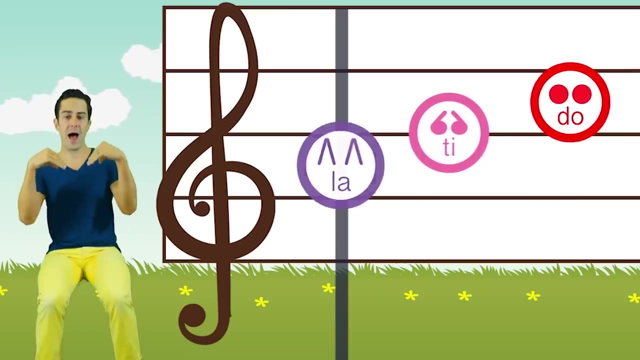 So let's start out down here with: Do Ready set. go Re mi fa You sing it Re mi fa Listen. we'll go. Sol la ti do You sing. Sol la ti do Listen faster. 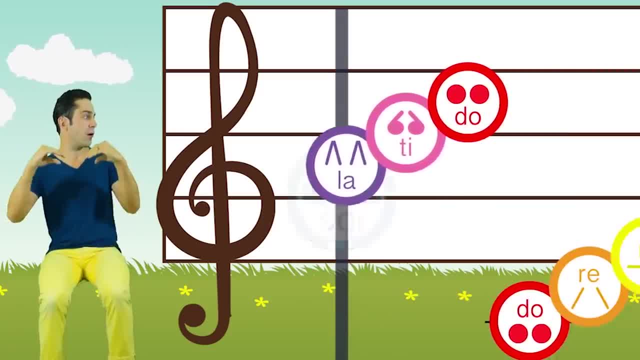 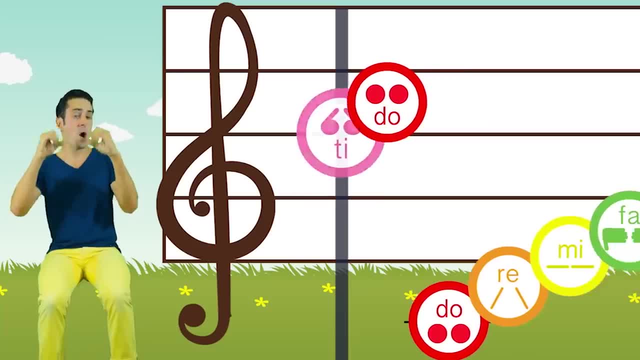 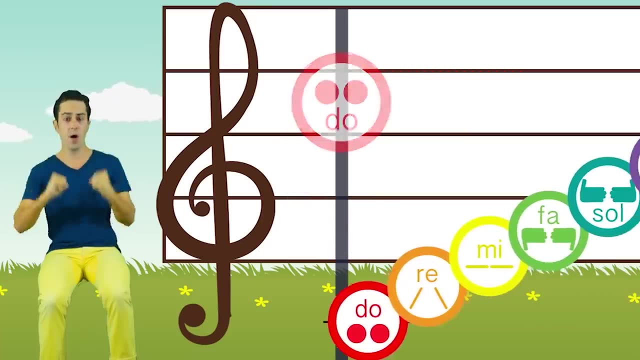 Do re mi fa Sol la ti do You sing All together. Do re mi fa sol la ti do. Do re mi fa sol la ti do. 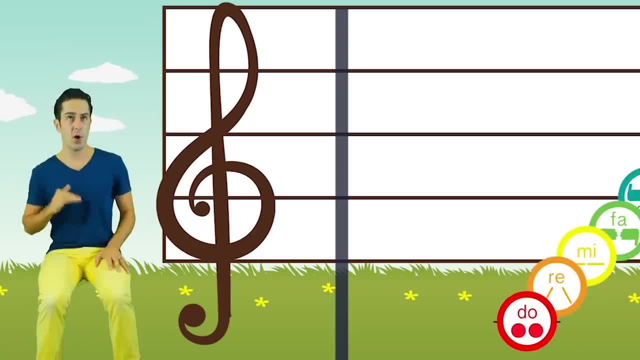 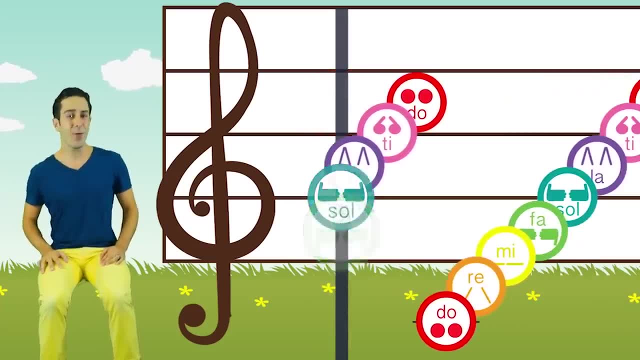 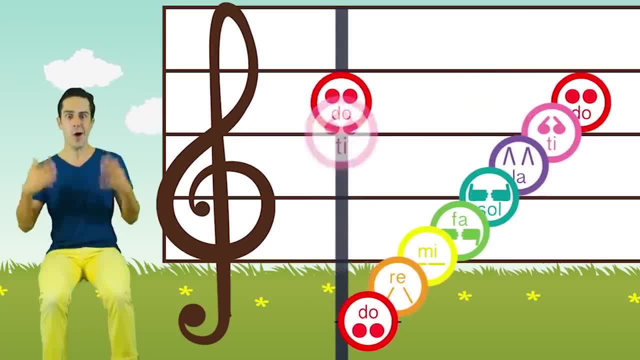 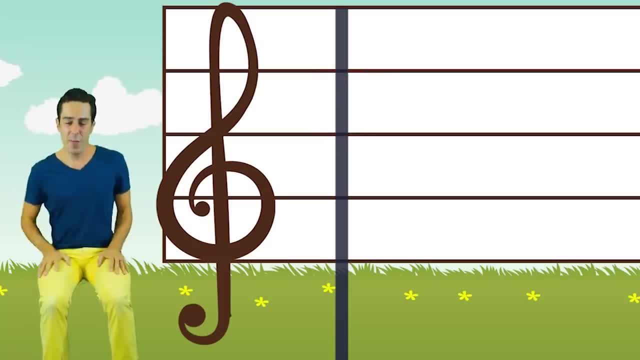 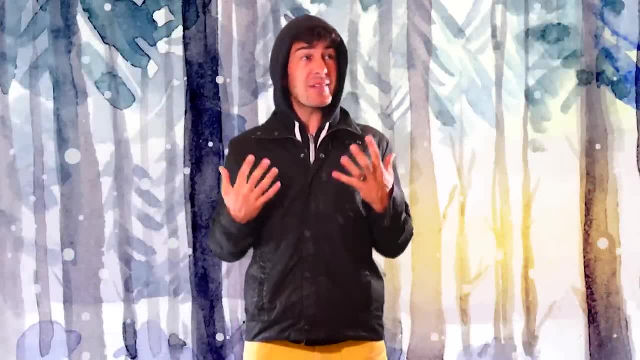 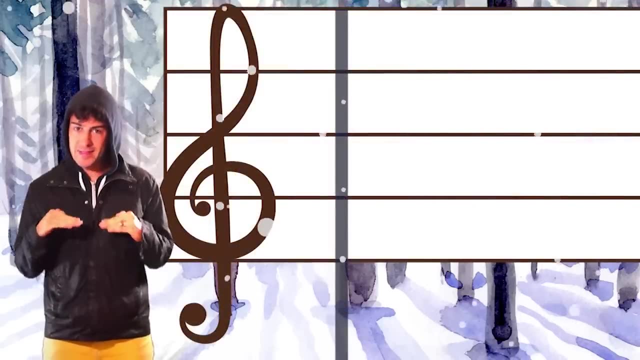 Hey everyone and welcome to a very snowy episode of PSP Melodies. My name is Mr Rob and today, as always, we're going to be singing and hand signing with the solfege syllables. The music is going to scroll this way and hit the blue line. 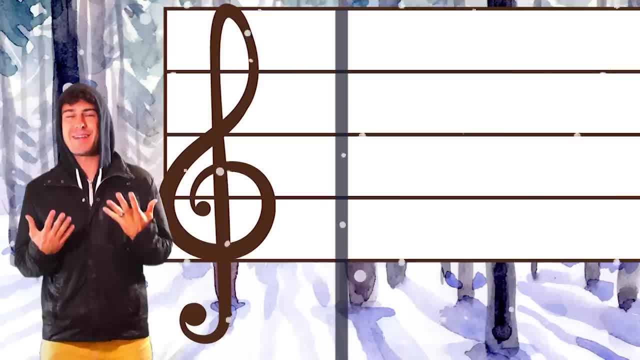 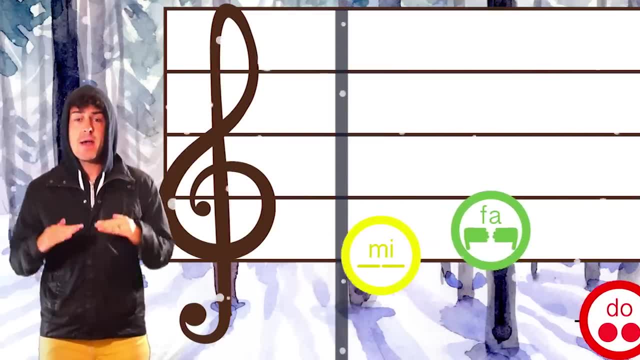 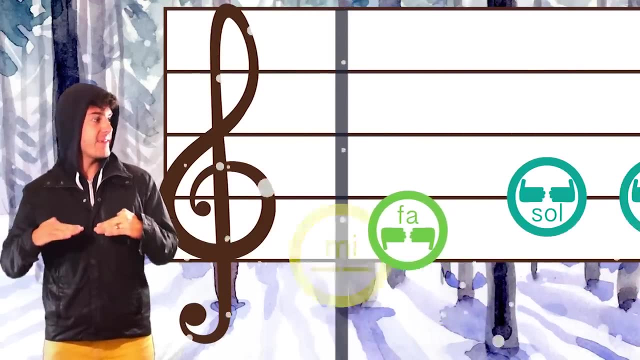 And when the circle is right on top of the blue line. that's when we're going to sing and hand sign. Let's start out with Do Ready, Do re mi fa. You sing Re mi fa. Then we sing. 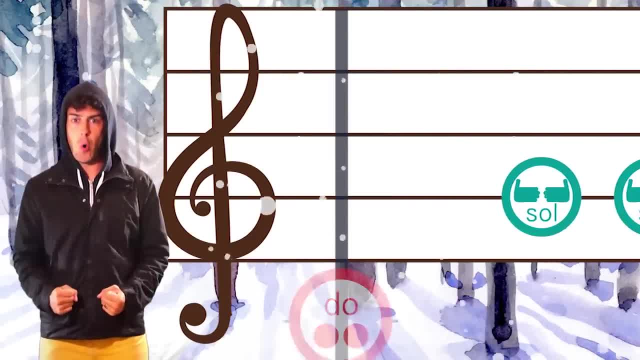 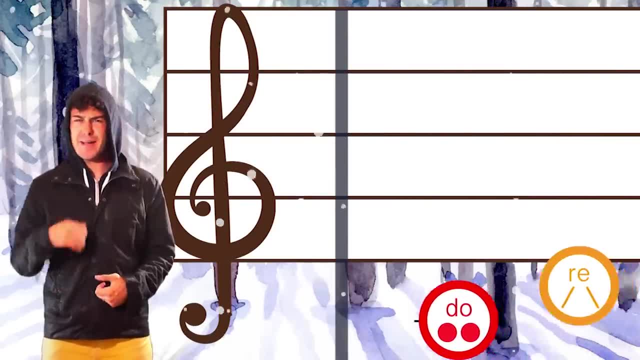 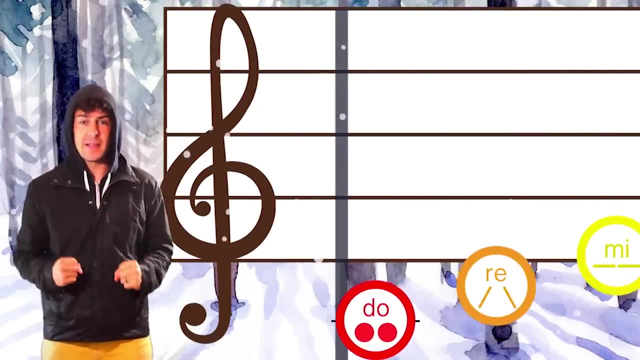 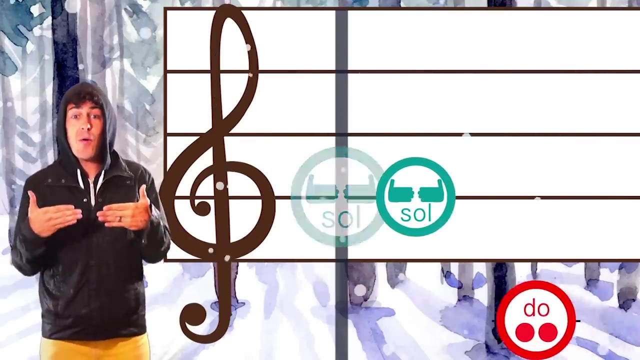 Sol, sol, Down to do. You try it Ready, Go Down to do. Hey, back to the beginning. Let's try. Do re mi fa. You sing it, Do re mi fa. Then off to sol, sol do. 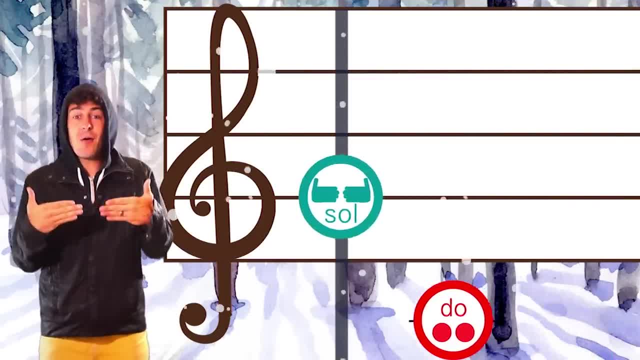 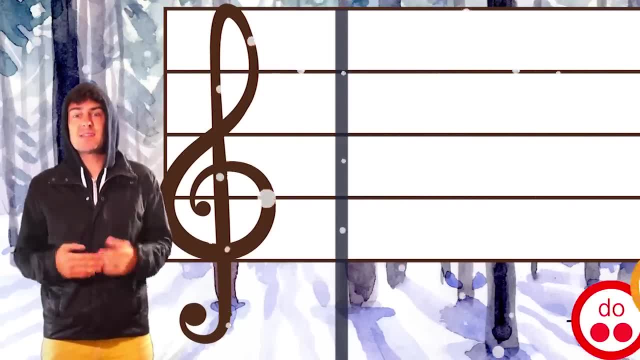 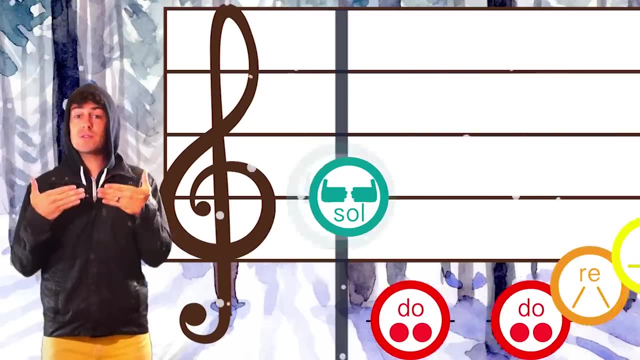 Nice and loud: Sol sol do. Hey, nice job with today's melody. Sounds nice and slow. Let's try it a little bit faster. Ready set. Do re mi fa. Sol sol do. 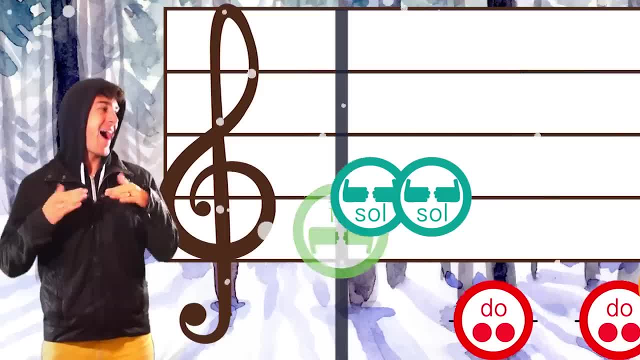 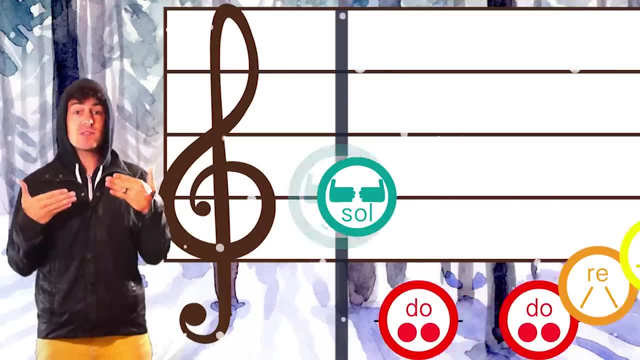 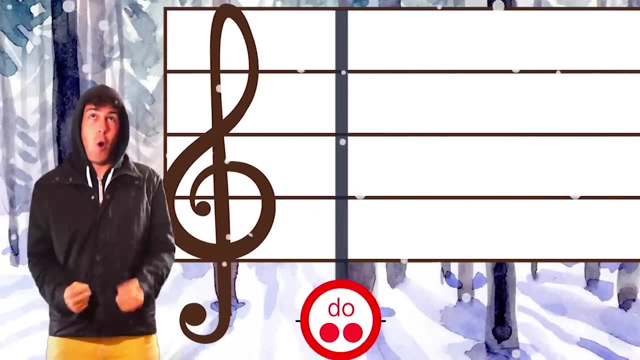 You do it All together. Do re mi fa Sol sol do Nice and loud. Do re mi fa Sol sol do. Hey, nice job. We're going to try it even faster, okay. 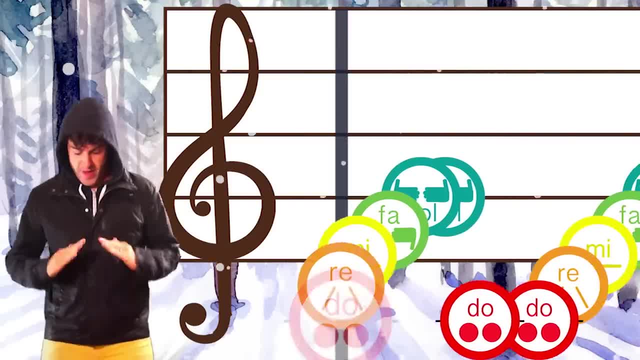 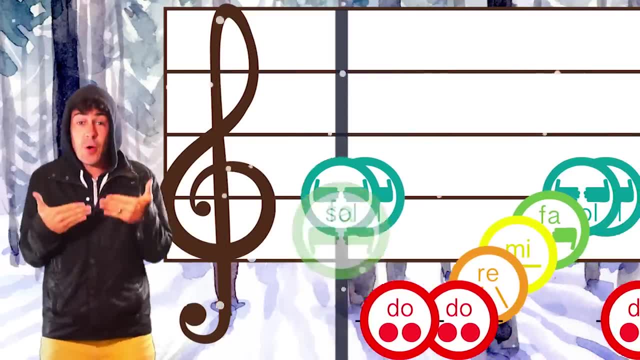 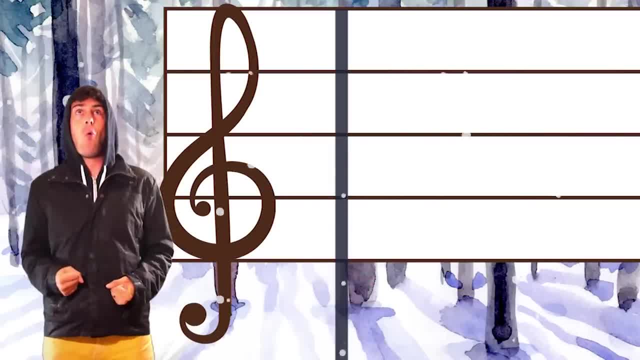 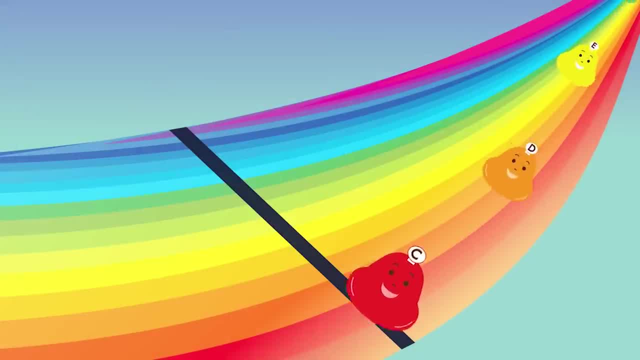 Do re mi fa, Sol, sol do. Hey, give yourself a huge round of applause. Nice job with today's episode of PSP Melodies. Thanks so much for hanging out today, and until the next episode I will. 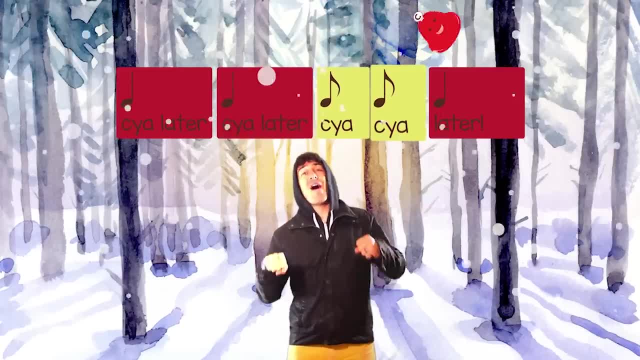 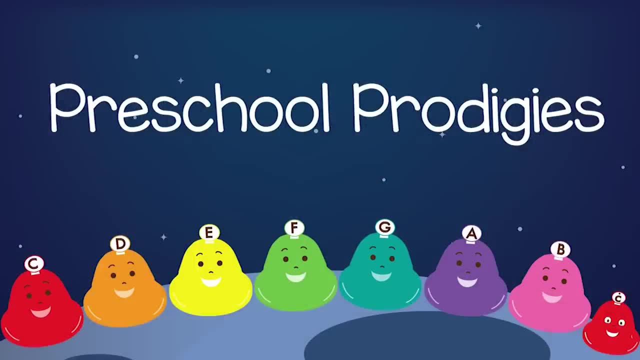 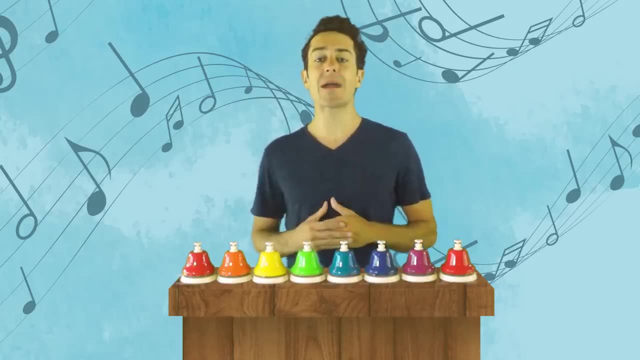 See ya later. see ya later. see ya, see ya later. Nice work. with those two episodes of PSP Melodies, everyone. Now we're going to keep practicing with our hand signs in this little game of What Song Is It? In this next video we'll sing and hand sign with some popular kids' songs and you'll have to figure out what song we are singing and hand signing. 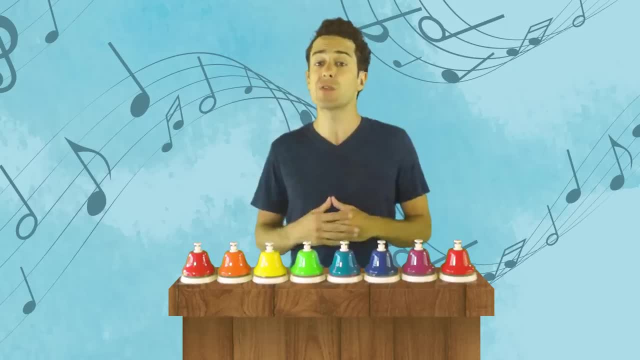 Some of the songs do move a little bit slower than you might be used to hearing them, but that will help you sing and hand sign with more accuracy. Inside the Prodigy's Playground we have faster versions and more advanced versions of all the songs that we're going to complete in this next lesson. 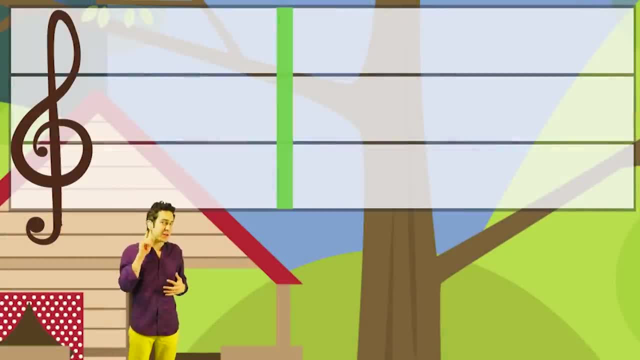 So this is going to be our first song. We're going to sing and sign. You're going to listen and tell me what song it is. When the music comes this way and hits the line, that's when we're going to sing. 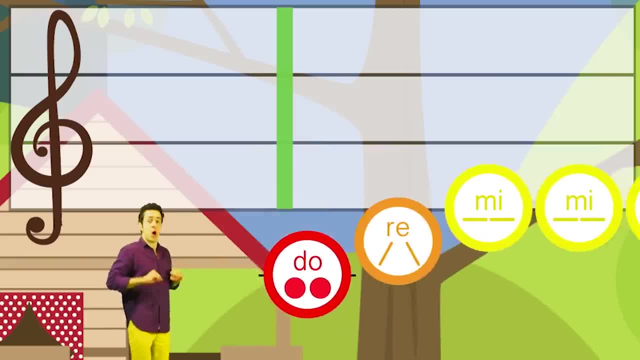 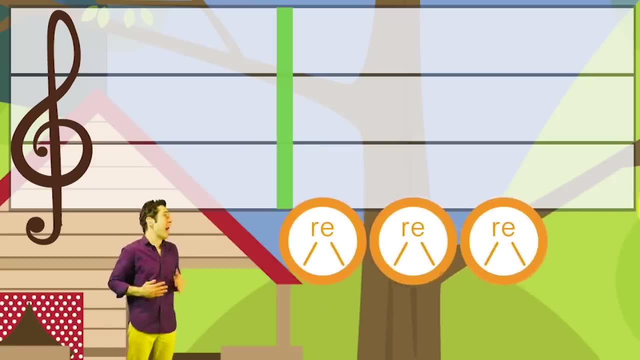 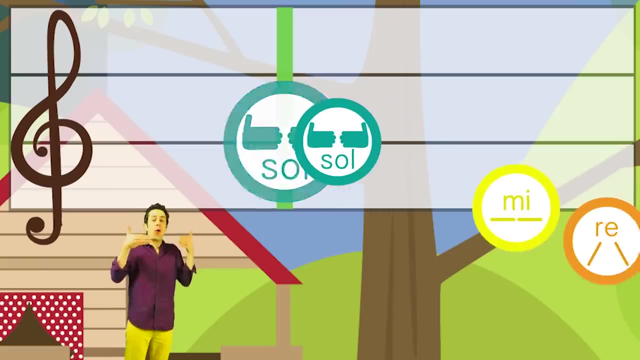 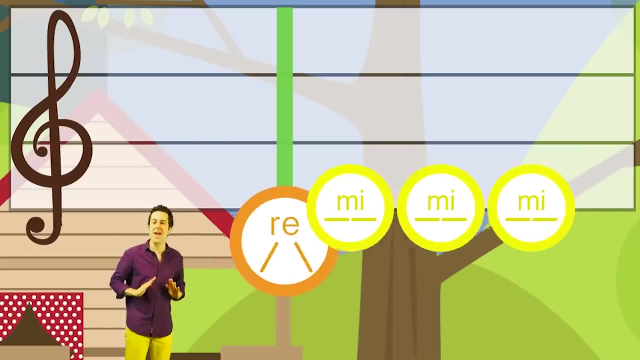 Here we go. Mi re do re, mi, mi mi. What song is that? Re re re, Keep on going, Mi sol sol. What song is it? Mi re do re, mi, mi, mi. 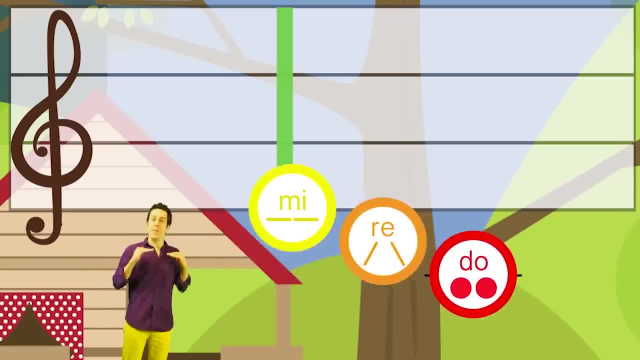 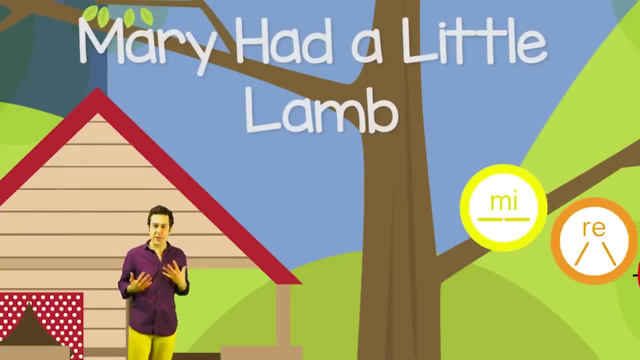 Back to re, Re, re, mi re do. Do you know what song it was? Yeah, it was. Mary Had a Little Lamb. Did you hear it? It kind of went like this: Mary had a little lamb, And so on. 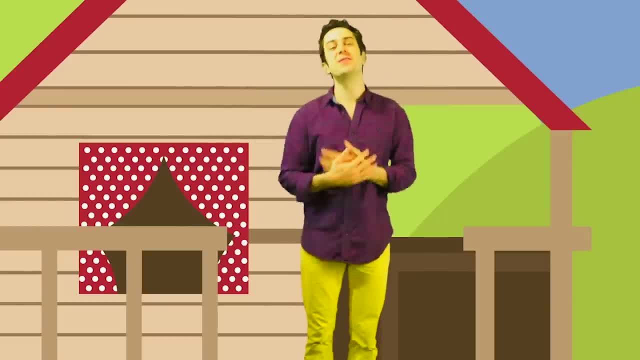 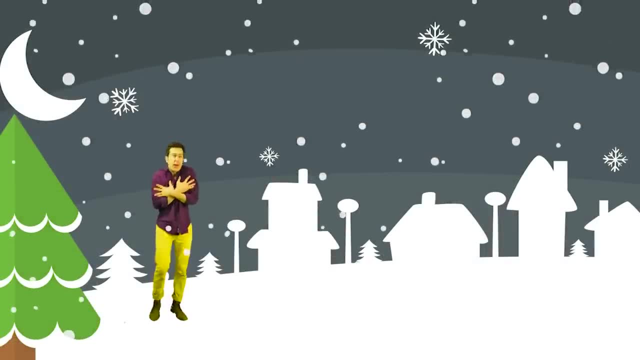 Nice job with that one, everybody. All right, we're going to jump into the next song. It's cold here. I wonder what song it's going to be. All right, are you ready? Here it comes, flat hands, one, two. 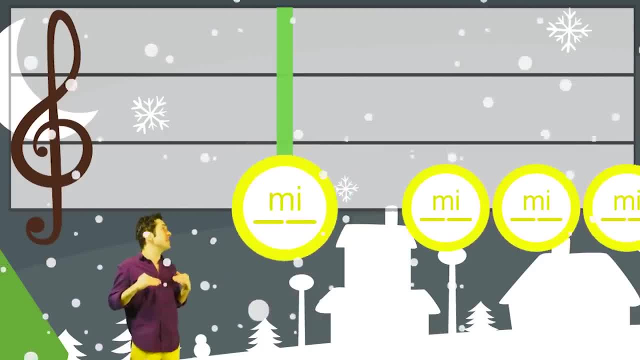 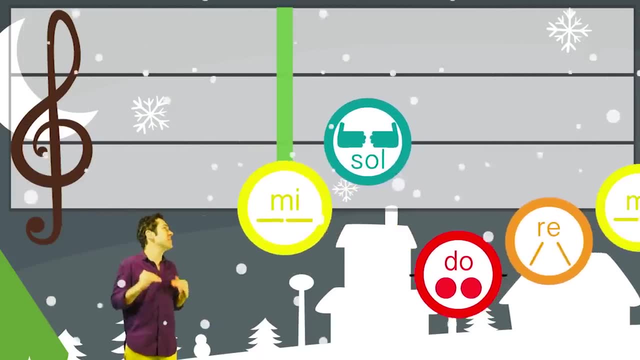 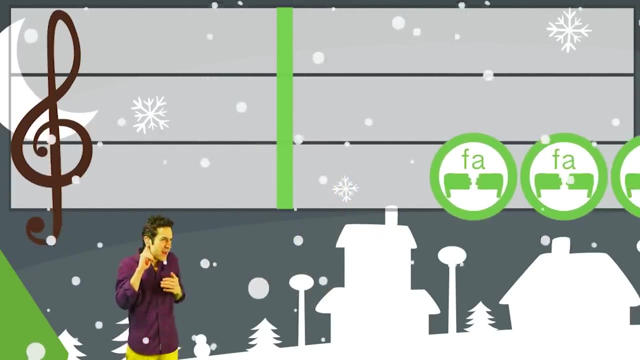 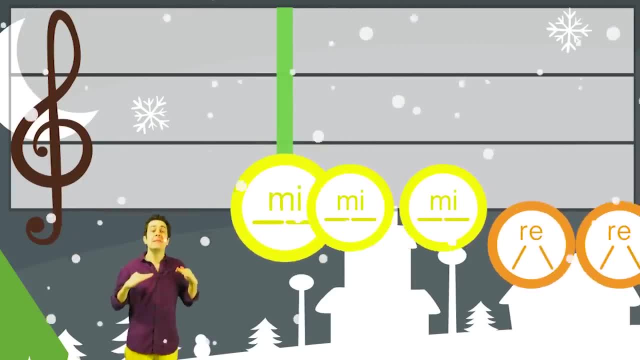 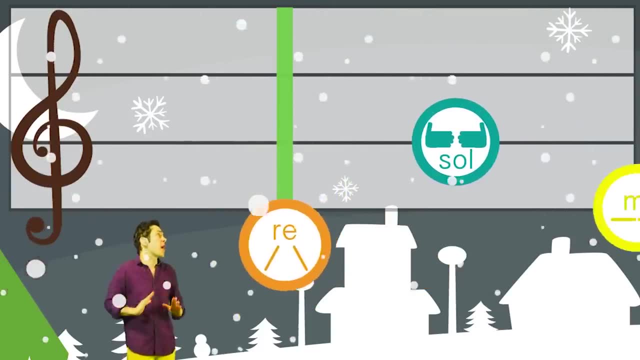 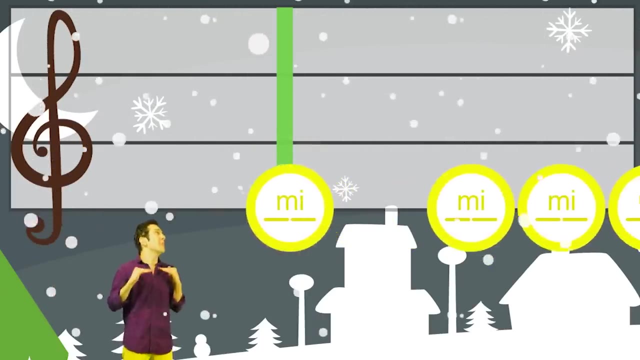 Fa fa mi mi mi mi, re, re, mi re. up to sol to sol, it's Jingle Bells, Mi mi mi, king, and sign mi mi mi, almost to the end. 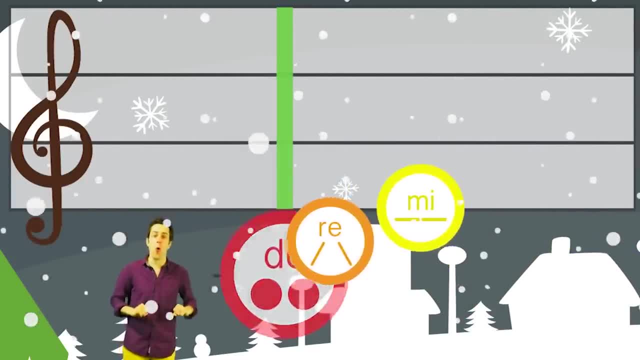 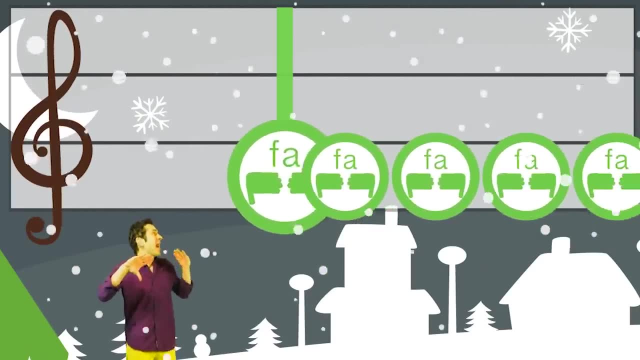 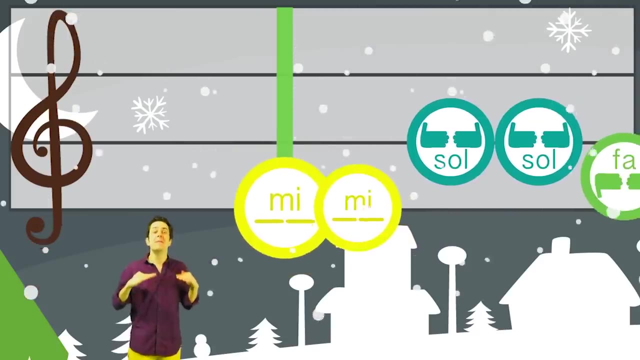 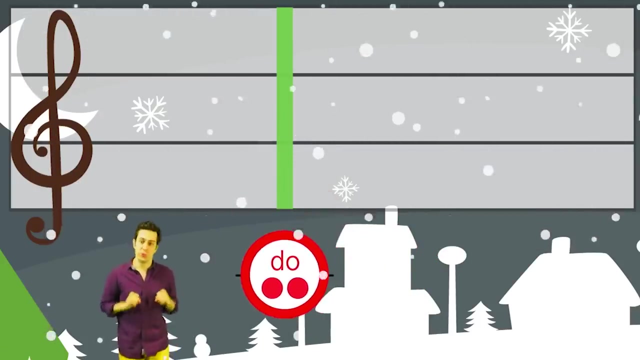 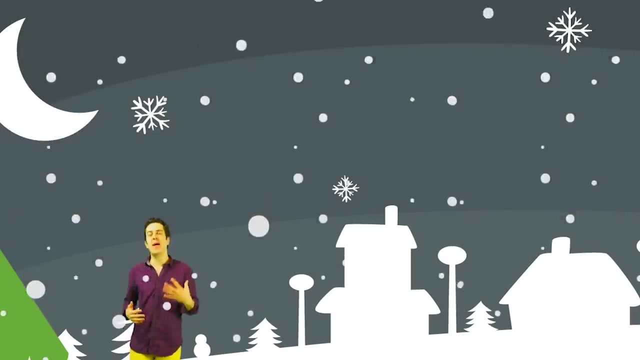 Mi sol do re mi. one more time with a thumbs down for fa Fa fa fa fa fa mi mi. mi sol sol fa re. do Nice job with Jingle Bells. everybody Great job singing and hand signing. 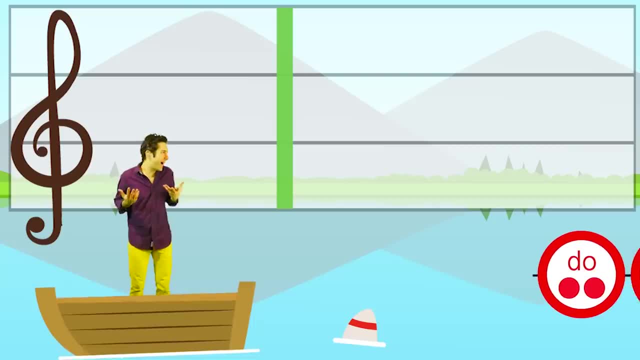 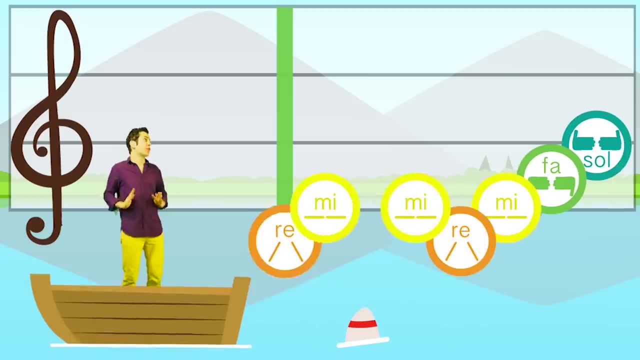 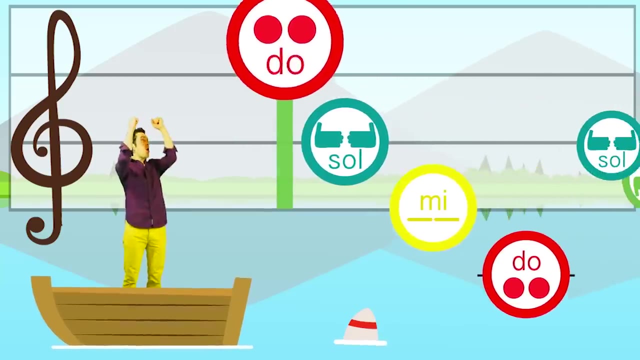 Alright, let's jump into the next song. I wonder what song this one's gonna be. Here it comes. Do do do re mi mi re mi fa sol. You got it. Do sol mi, do sol fa mi re do. 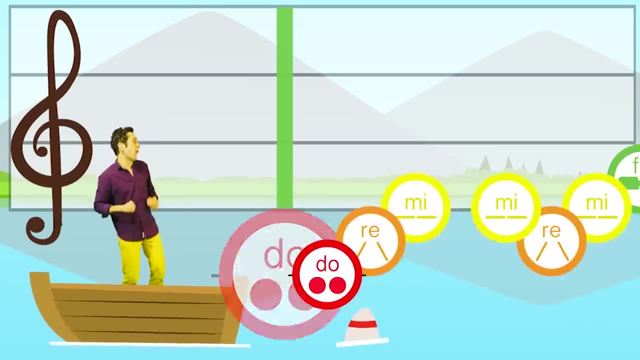 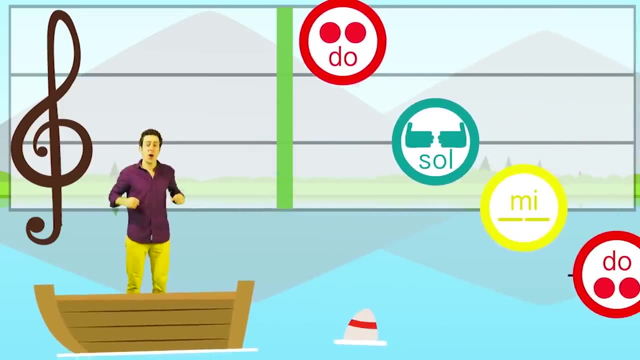 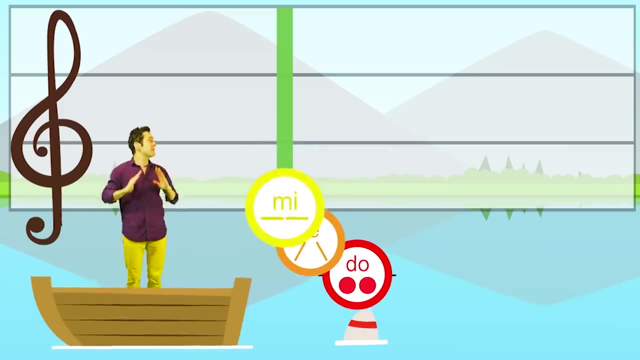 One more time: Do do do re mi mi re mi fa sol To do Do sol mi, do sol fa mi re do. Do you know what song it is? 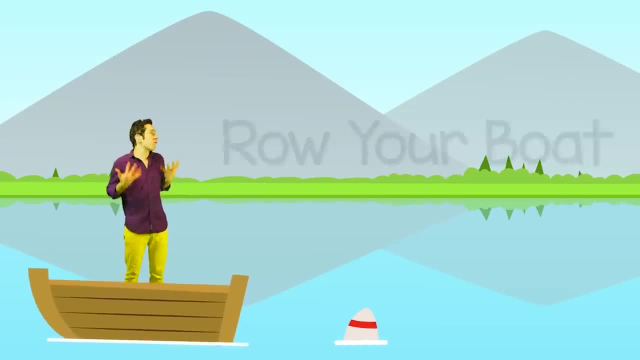 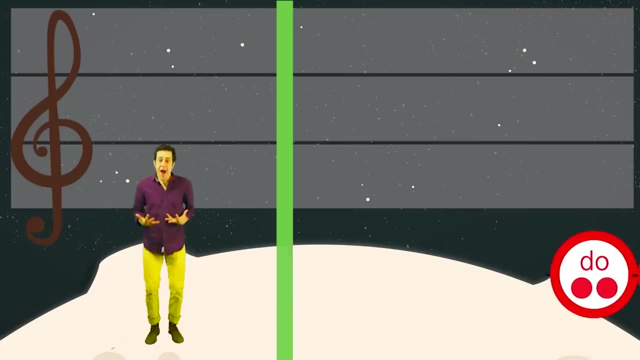 Yeah, you do. I mean, we're on a boat, It's gotta be Row, Row, Row Your Boat. Nice job with that one. We're gonna jump into the next song. Alright, let's jump into the next song. 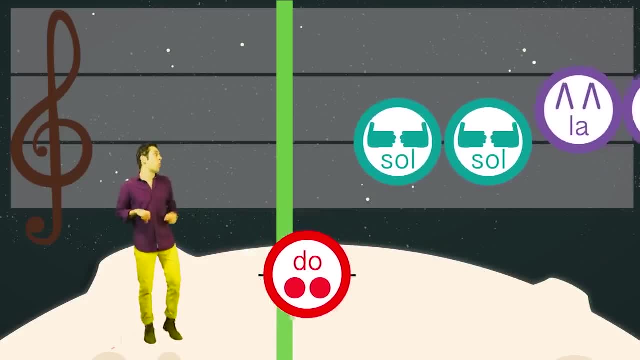 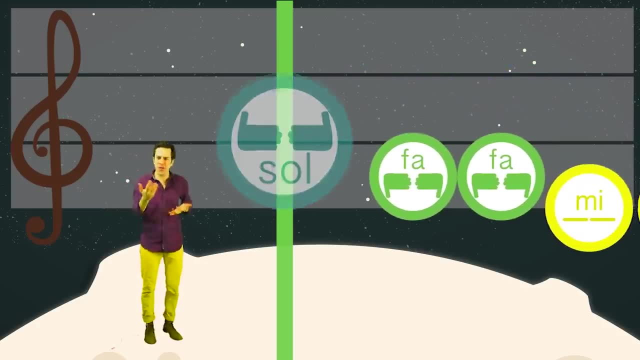 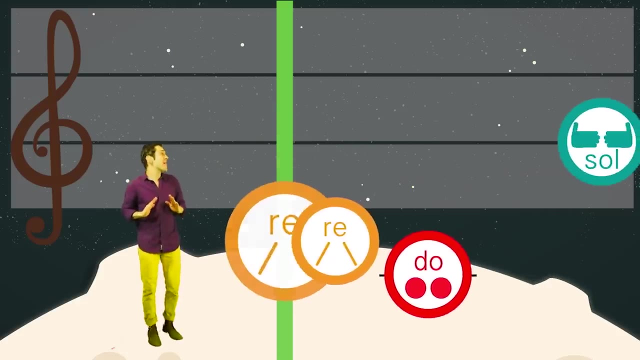 Here it comes, Ready set. we got Do do sol, sol la la sol. What song is it? Fa fa mi mi re re do. Yeah, it's Sol sol mi mi mi re re do. 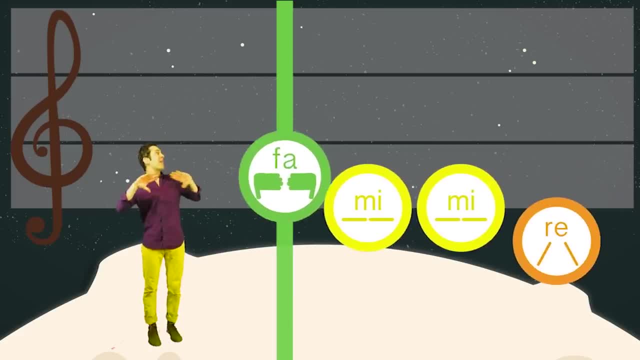 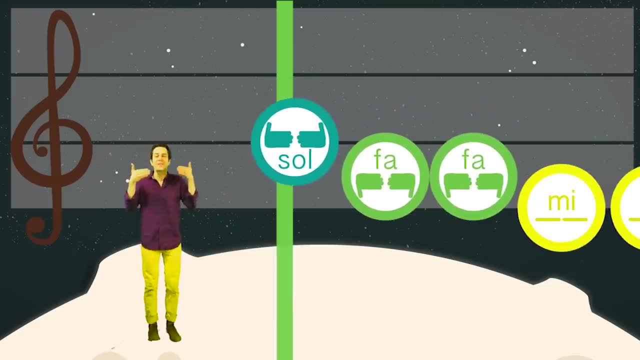 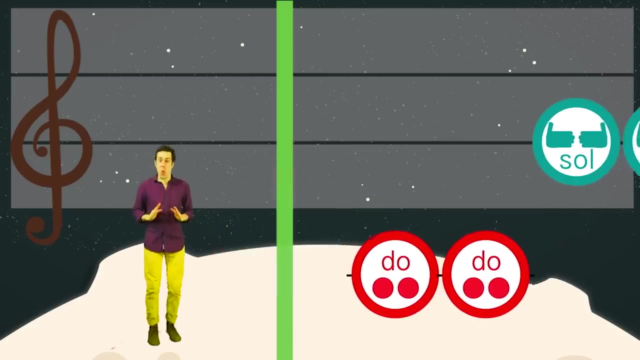 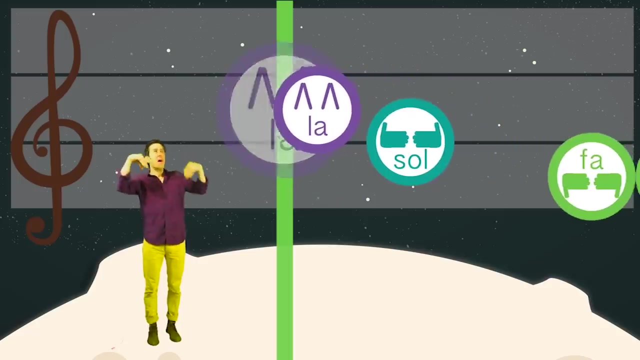 Sol, sol fa fa mi mi re do Again. Sol sol fa fa mi mi re do Whoops Fa to do, Do, do sol, sol to la, la, la to sol. 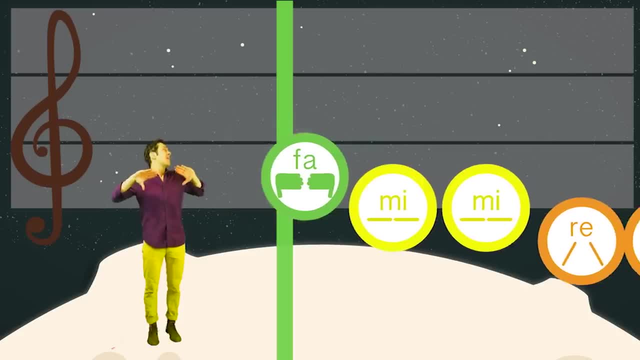 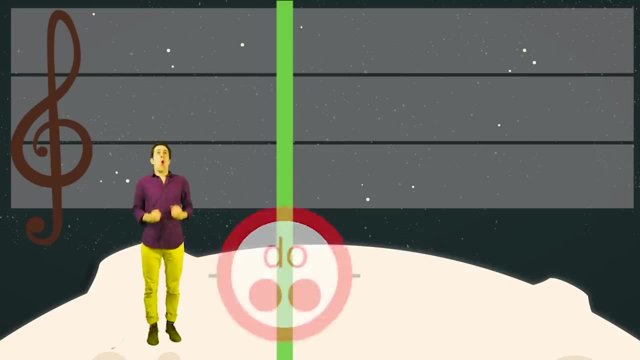 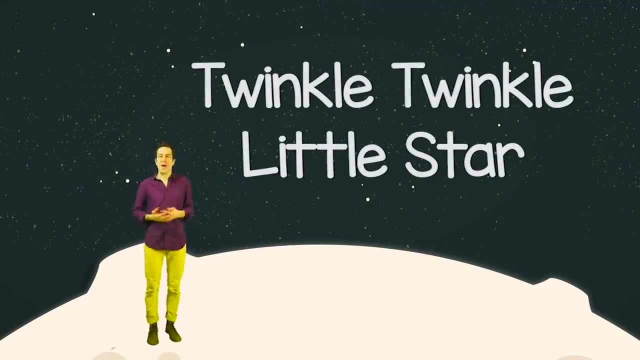 Sol back down to fa, Fa, fa, fa, flat hands, Mi mi re re do. What song was that one? Yeah, it's Twinkle, Twinkle Little Star. We're out here in space. 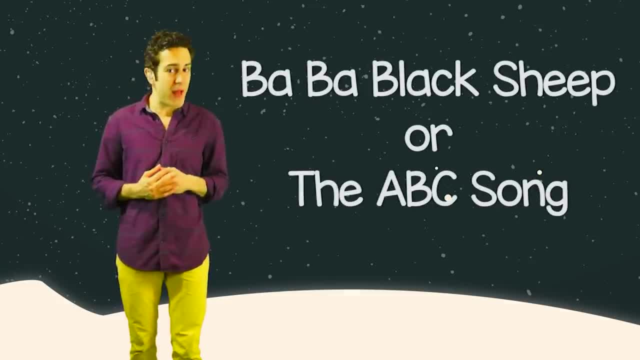 It had to be Twinkle Twinkle Little Star. If you thought it was Baa Baa Black Sheep or the ABC song, they actually have the same melody. It's sung to the same tune, So if you thought it was either of those, you were right. 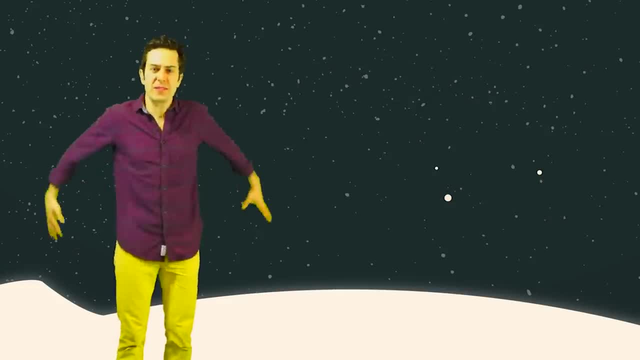 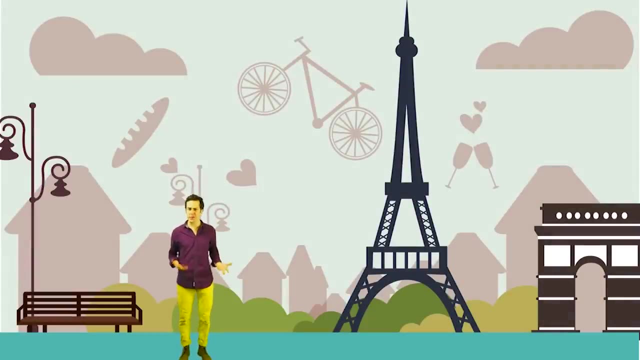 It's the same thing. All right, we're going to jump in and do one more today. Let's go Ready set. So we're here in Paris, France. Huh, I wonder what songs that we know that are in French. 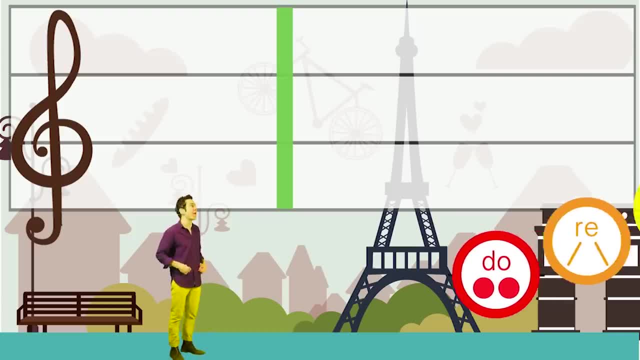 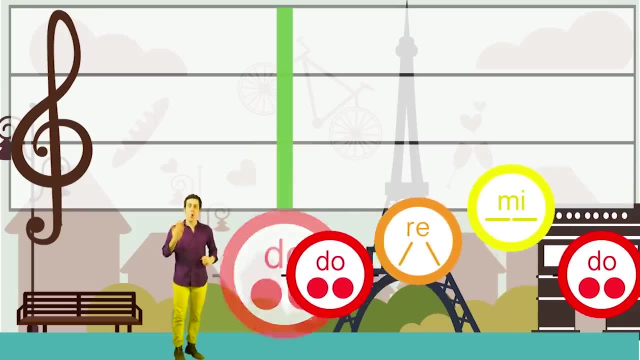 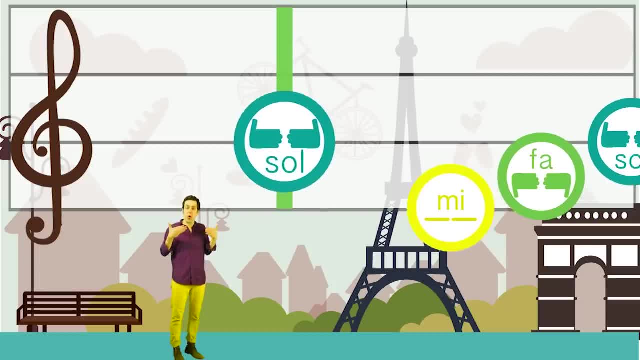 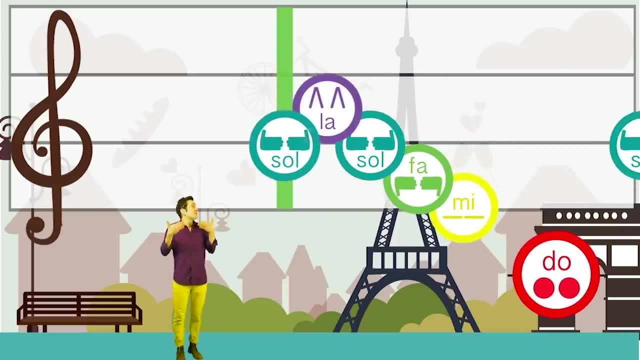 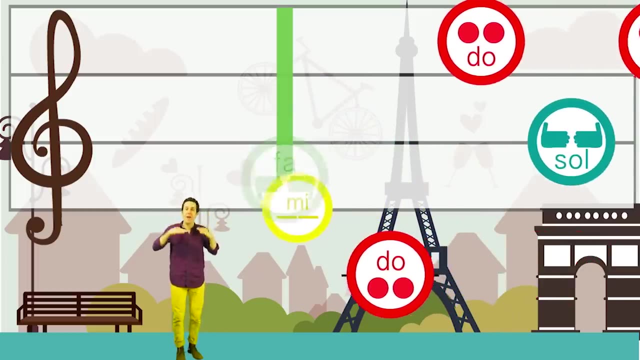 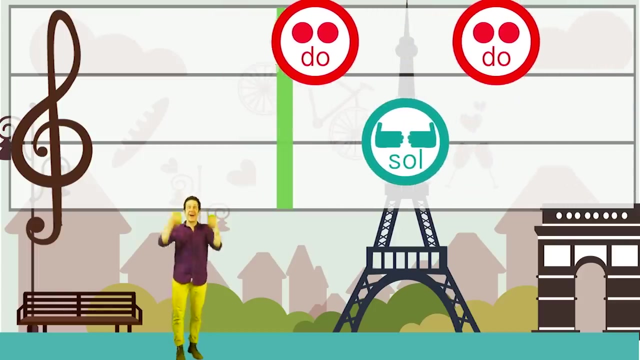 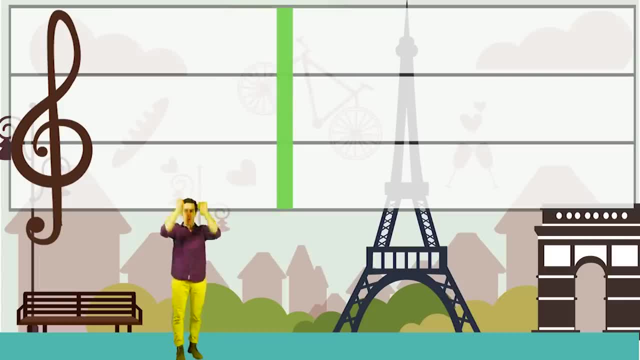 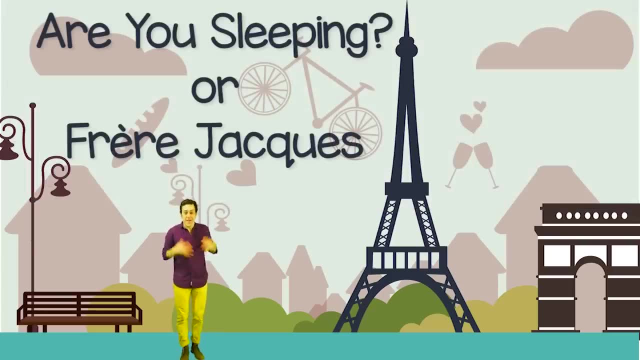 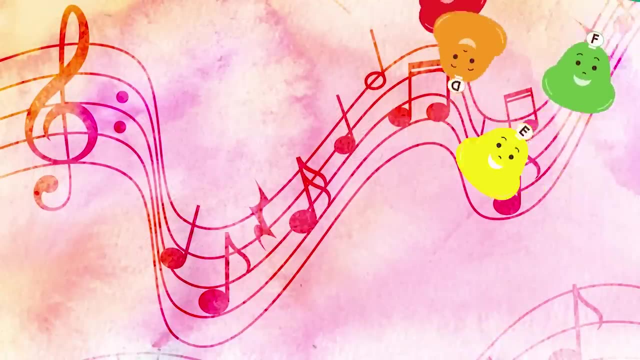 do sol do. What song was it? It was: Are You Sleeping or Frère Jacques? Hey, great job today. everybody Give yourself a huge round of applause. Nice job singing and hand signing all these famous melodies. Nice job, with What Song Is It? everyone? 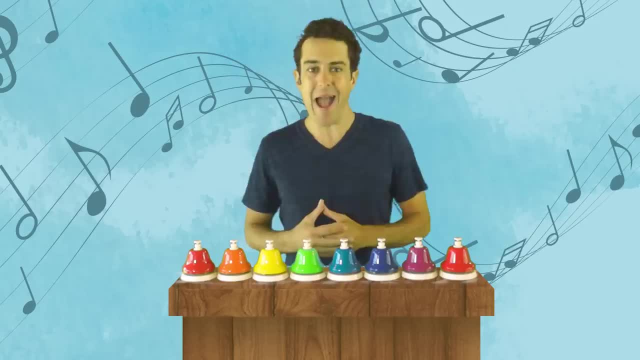 What Song Is? It is a little listening game that tests your musical ears, And in the next two videos we're going to do some more listening activities. Before we get to those activities, though, I wanted to really quickly talk to you about the Prodigy's Desk Bells. 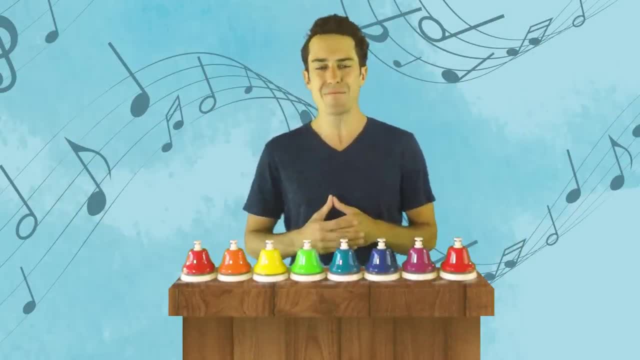 These bells are the backbone of our full-length program, the Prodigy's Playground, And for lots and lots of reasons, these bells are, hands down, the number one musical instrument for young children. They're colorful, they're super well-tuned. 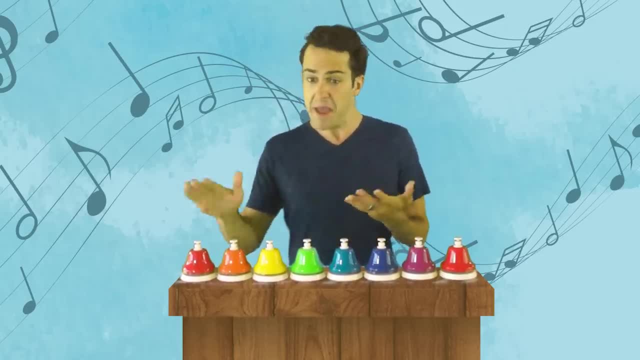 they're durable and they're really easy to play. All you have to do is hit it and it rings out and it sounds great. And because they are individual musical objects, they allow you to focus on one or two or three or whatever sort of select group of notes that you want to at a given time. 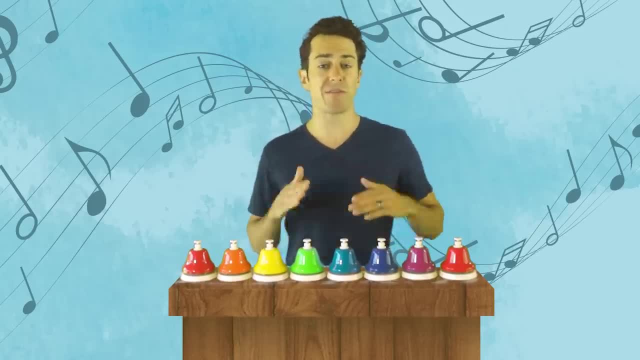 Now you probably don't have a set of bells yet, which is why we're doing a lot of tapping and clapping and singing and hand signing today, But I wanted to show you a short clip of an early bell lesson from the Prodigy's Playground. 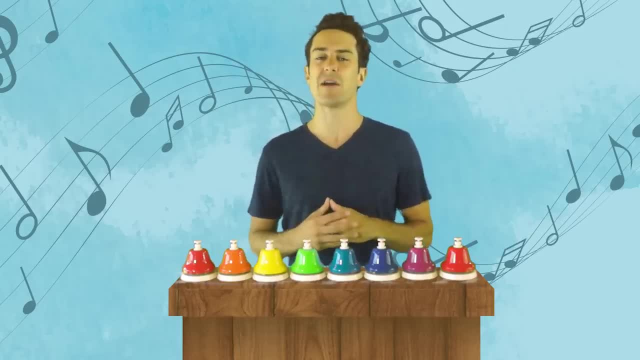 that will actually get you ready for the next two listening videos. And, of course, if you want to get a set, a set of bells of your very own, you can head over to Preschool Prodigy's dot com slash bells to order a set. 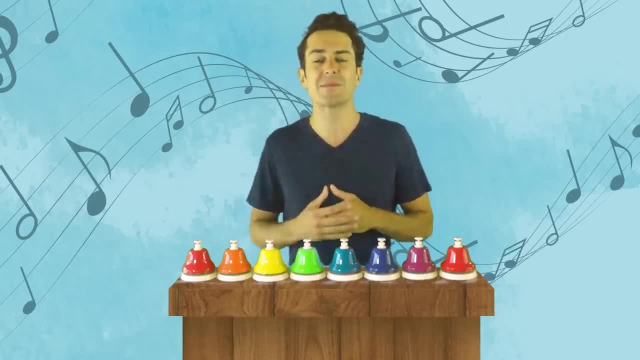 They're fully guaranteed by our team and they're easily one of the best investments that you can make for young kids playing music, All right, so let's check out a little bit of the Do Mi Sol slide before we get back to doing some listening activities. 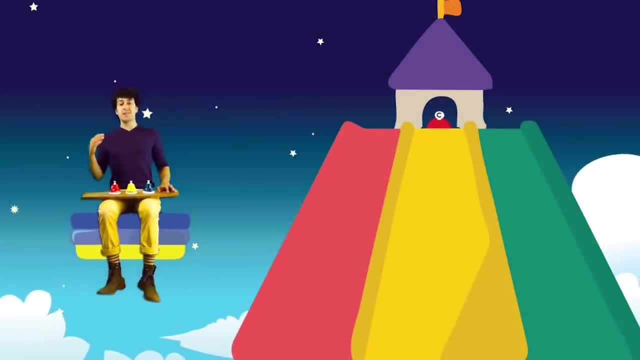 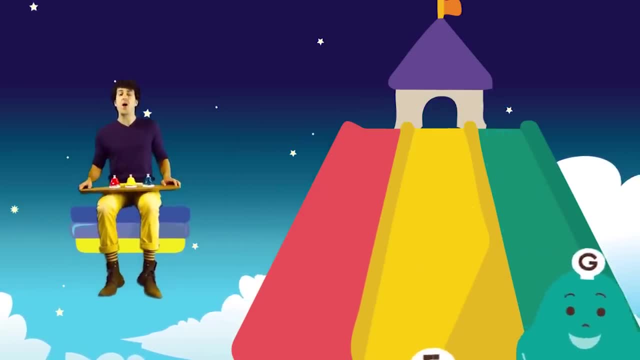 and the teal bell. Get all three of your bells out- red, yellow and teal- because today we're taking three musical notes and putting them together to make a chord. Can you say chord, Nice job. So a chord is a group of musical notes. 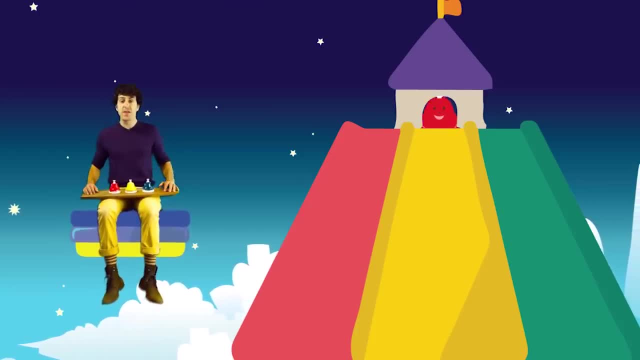 and most chords have three notes in them. We're gonna play this C chord. This is sort of our most important chord. It's like our home base chord. So this chord is based off the note C and it has the notes E and G in it. 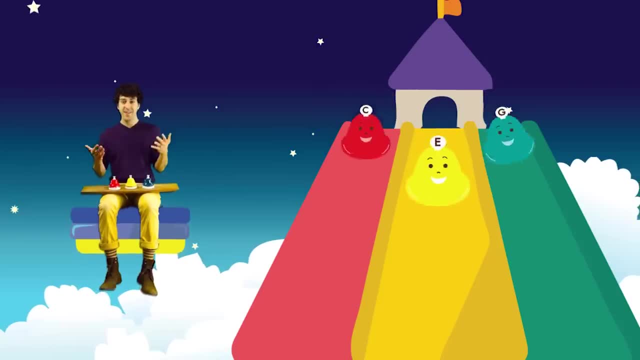 Can you play all three of yours together? Nice Well, today we're gonna play the notes separately, going up and down. We're gonna play the C, E, G, E and C. We're gonna sing a little song called Let Us Play. 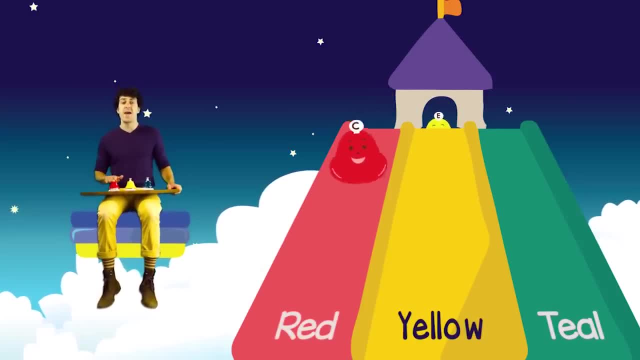 So follow along. It goes like this: Red, yellow, blue, red, yellow, blue, red, yellow, teal, teal. Sing and play. Ready set go Red, yellow and teal. Let's try it backwards from teal. 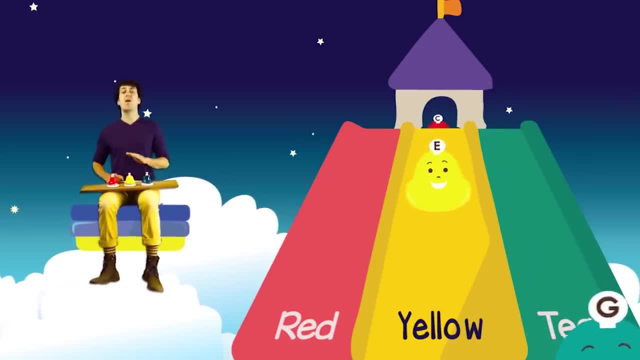 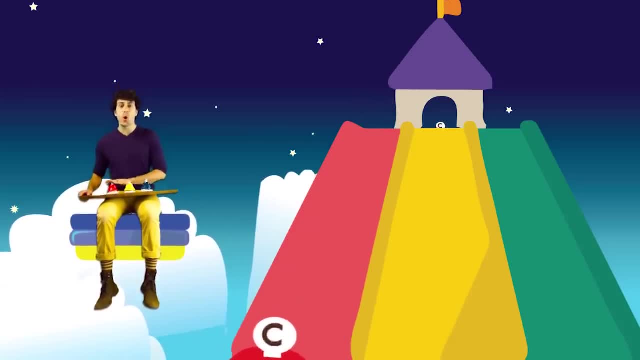 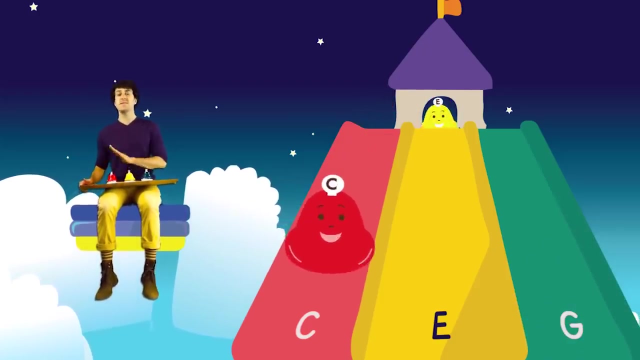 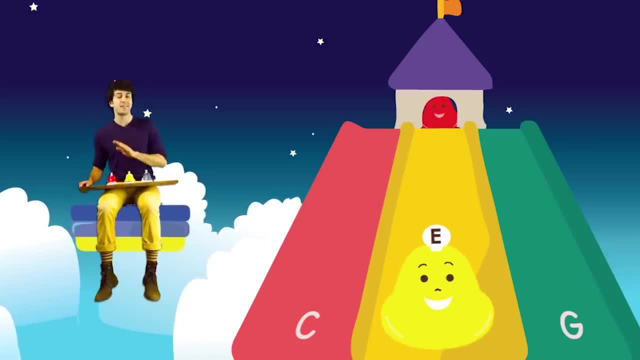 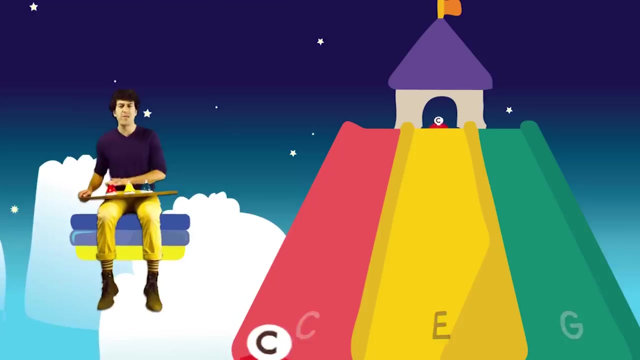 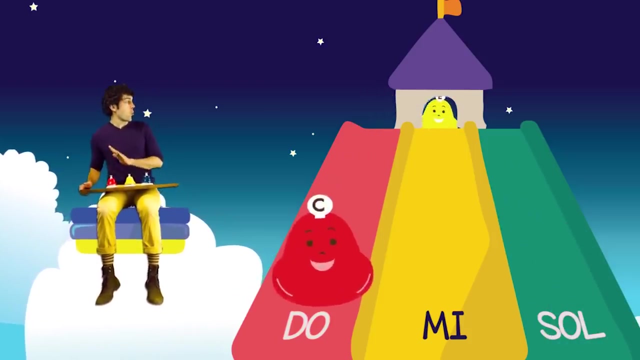 G, G, G, G, E and C. Nice job, fellas. One more time like that: G, E and C. We're going to use the solfegg syllables Do mi sol, Do mi sol. Nice job everybody. Do mi and sol. 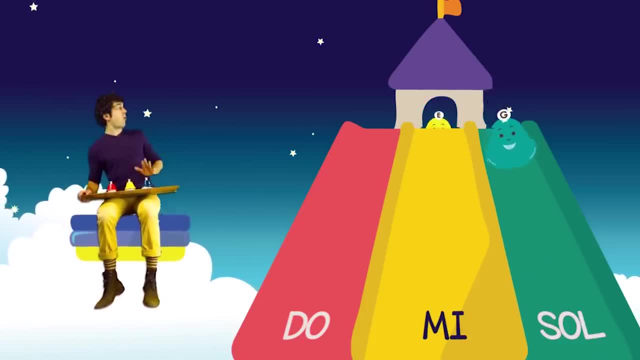 Let's try it a little backwards, starting from sol Sol mi do mi, sol, Sol mi do. One more time, Sol mi do. Let's add the words Let us play, Let us play. 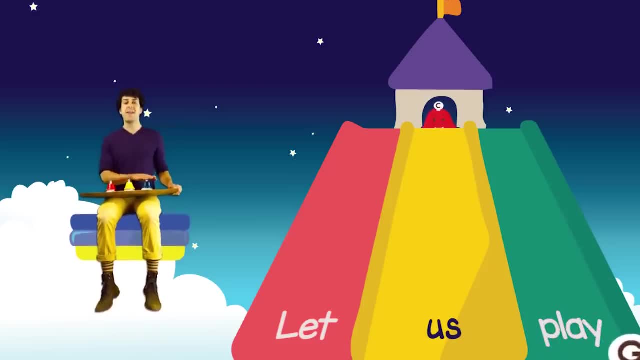 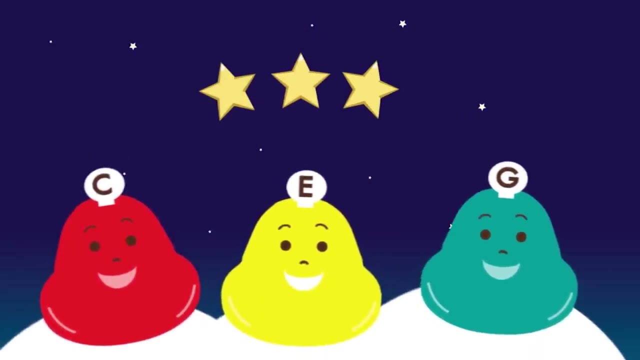 Let us play. Yeah, Let us play. Play Two more times. Let us play Very last one. Let us play. Go back to do for one more time. Do Hey, nice job, Nice job everybody. Give yourself a big round of applause. Nice job playing. do mi and. 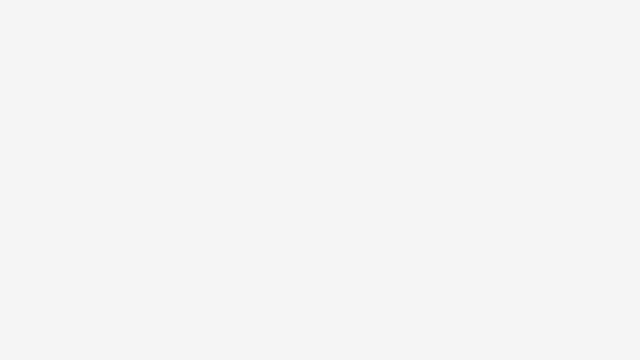 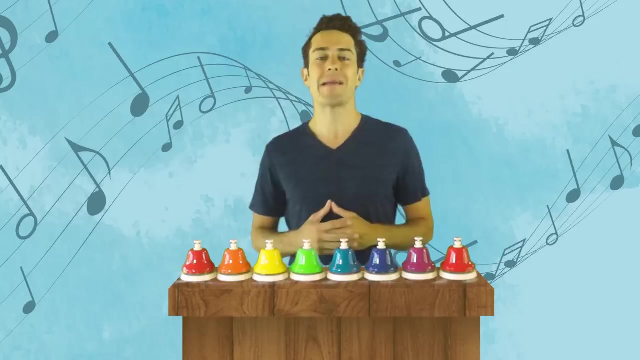 sol. So that was just a little clip of a bell lesson from the Prodigies Playground, just to kind of re-familiarize yourself or just to straight up introduce the idea of do mi and sol. In this next video we're going to do some chord watching and try to determine what kind 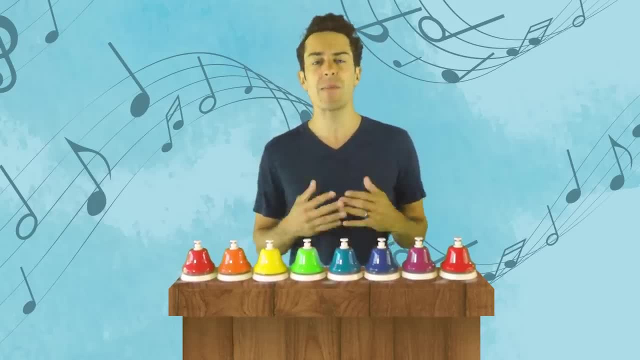 of musical group we are listening to. Inside the Playground we meet lots of chord players. We practice identifying these chords, lots of groups of musical notes, and we practice identifying these chords as a means of building up our musical ear and our sense of pitch. 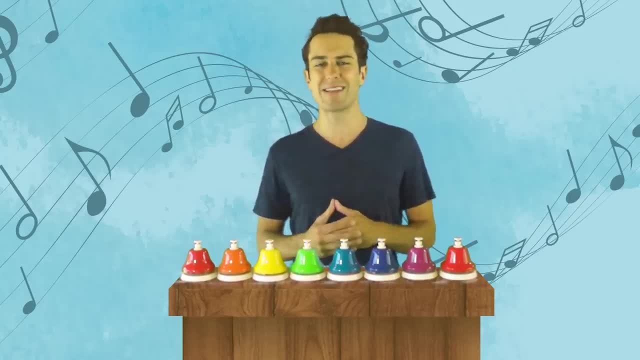 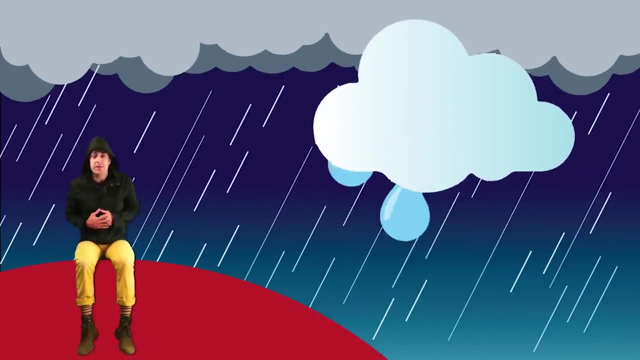 All right. Well, we'll talk a little bit more in the next video, but head over and I'll see you there. Hey everybody, and welcome to another Preschool Prodigies music lesson. Today we're out here in the rain doing some chord, watching Some people go out storm watching, looking for. 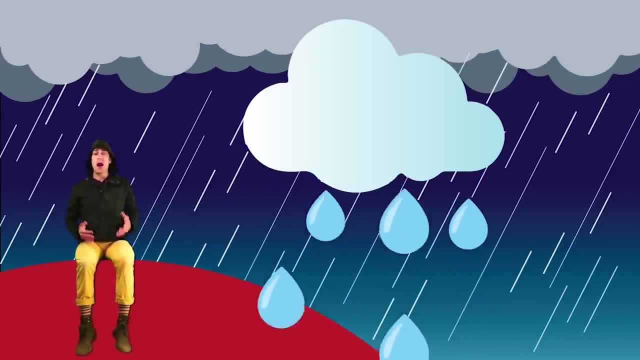 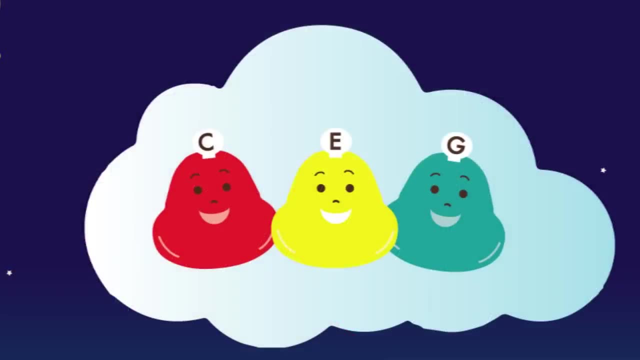 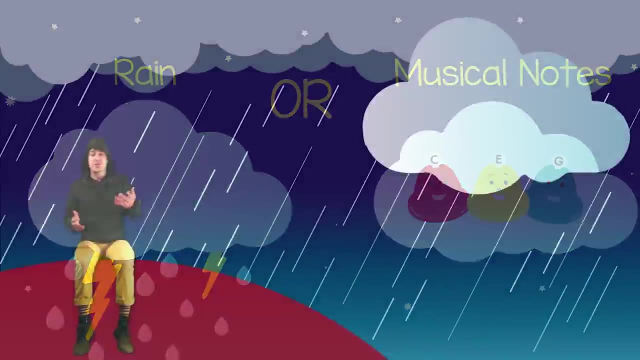 storms trying to take cool pictures of the lightning. But today we're out here in the rain. We're out chord watching. Well, a chord is a group of musical notes and we're looking to see if these clouds are either filled with rain or if they're filled with musical notes. 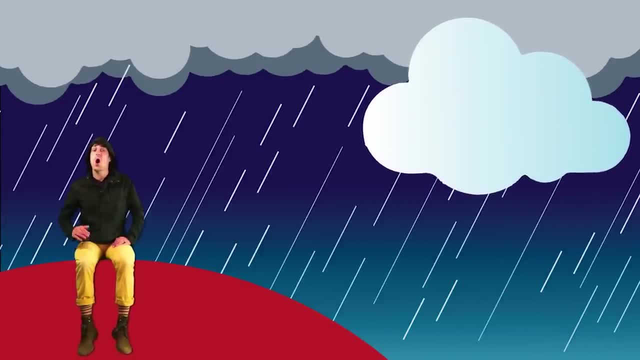 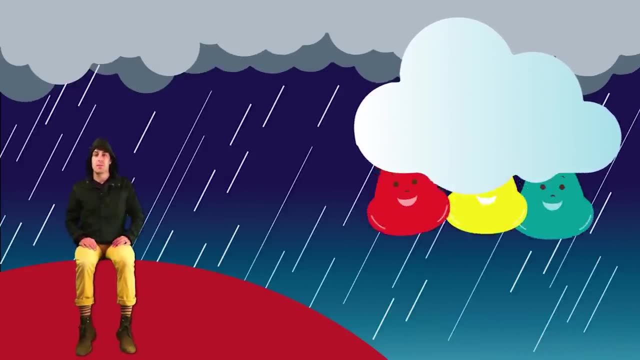 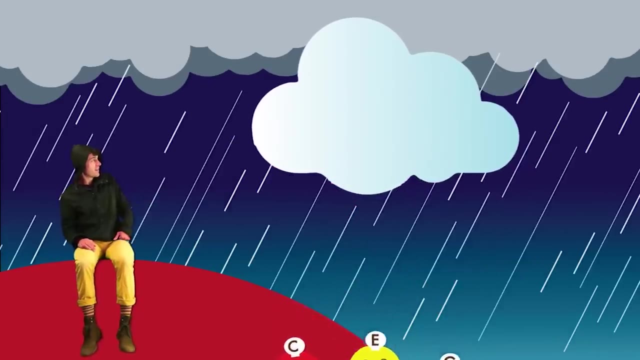 So the musical notes in today's chord watching adventure are C, E and G, And these three notes together make up the C chord. Did you hear it? That's our C chord. Yeah, here it comes. So when you hear that sound, you guys know it's going to be a C chord. 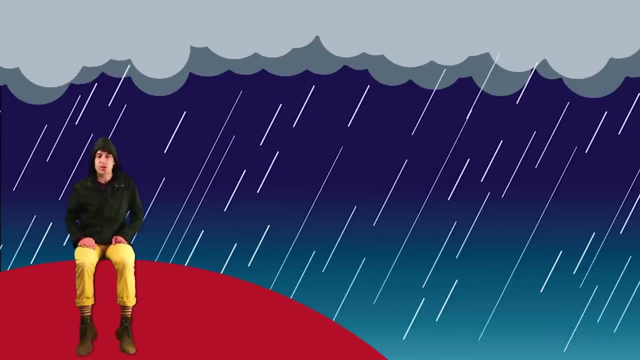 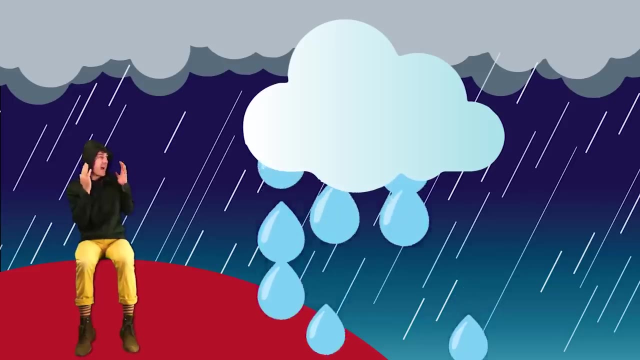 okay, When each cloud comes by, try to figure out which one it's going to be and then shout it out. okay, Do you hear it? Are those musical notes? No, that's some thunder and some lightning and some rain. That's not a chord cloud, That's a rain cloud. Yeah, you got it, That's a rain. 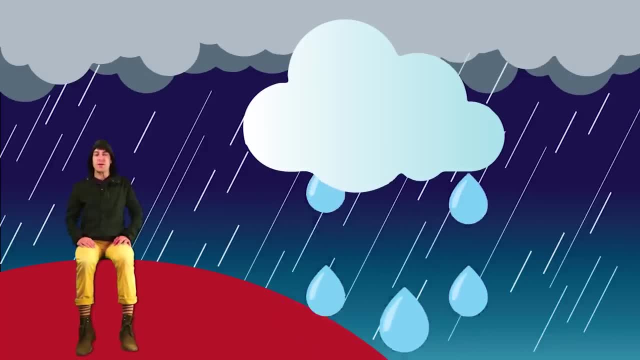 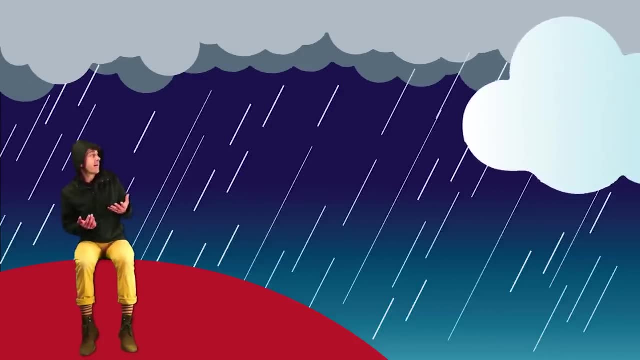 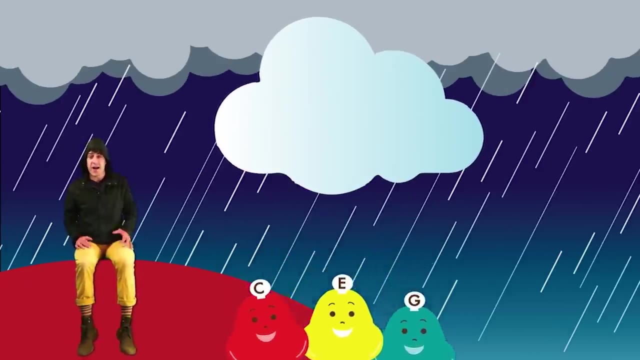 cloud. So just call it out when you're figuring it out. okay, I wonder what our next cloud's going to be. Do you hear it? I think I know what it is. Yeah, it's a chord cloud. It's a C? chord. Sometimes, when I hear a C chord, I like to put my hands on my heart, because 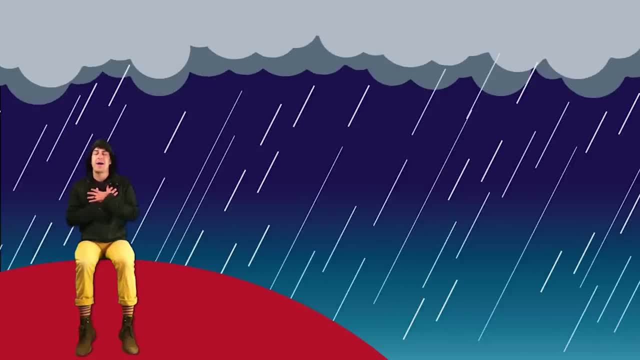 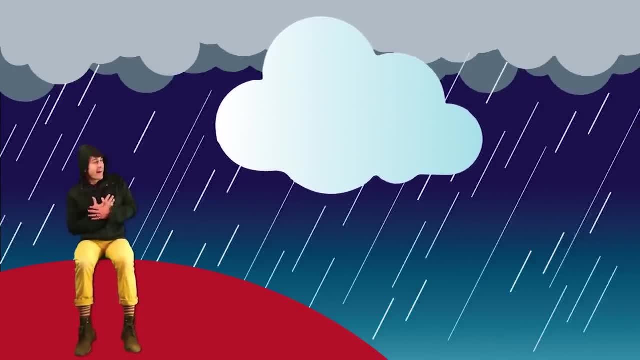 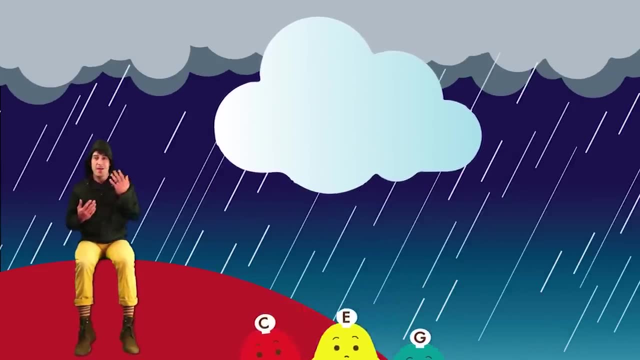 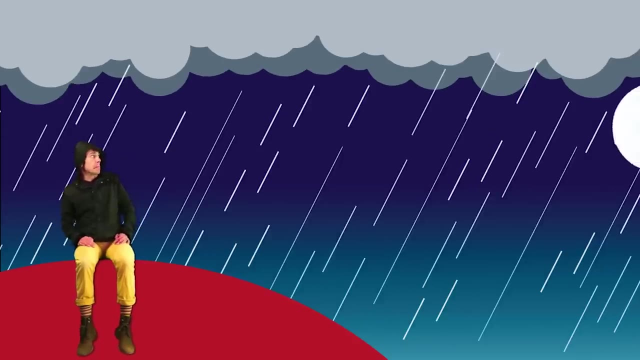 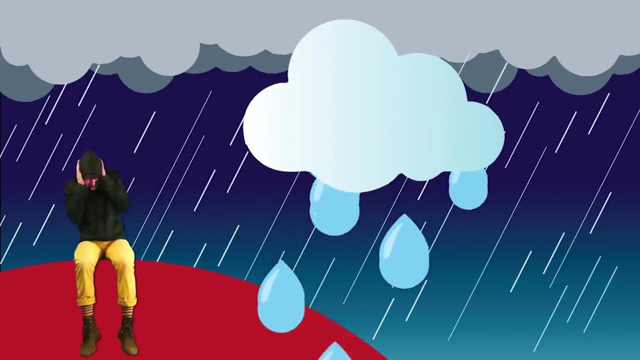 that C chord. And here they come. That's a great chord cloud. I wonder what the next cloud is going to be. What is that? Yeah, it's more thunder and lightning and more rain coming our way. That's not a chord, Oh man Woo. 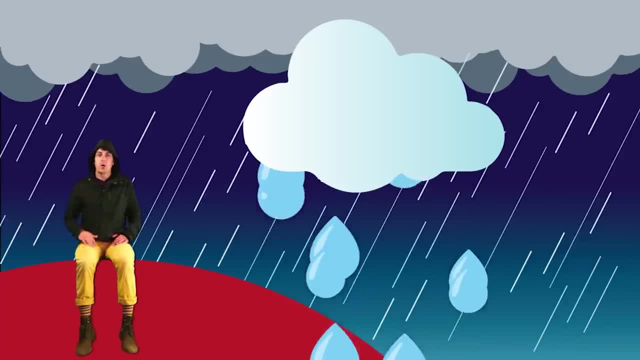 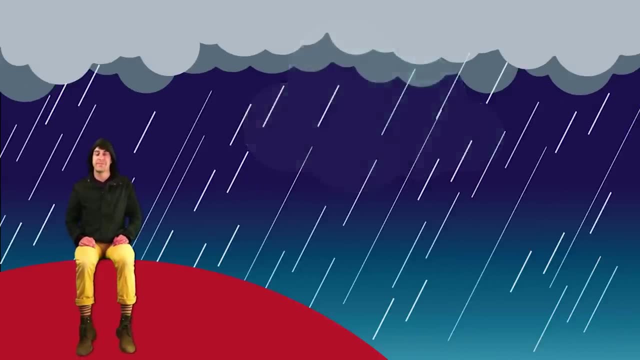 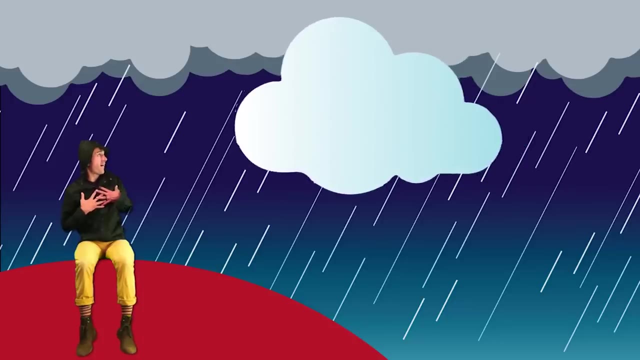 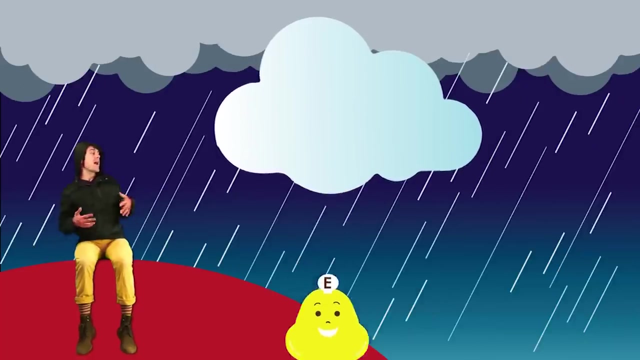 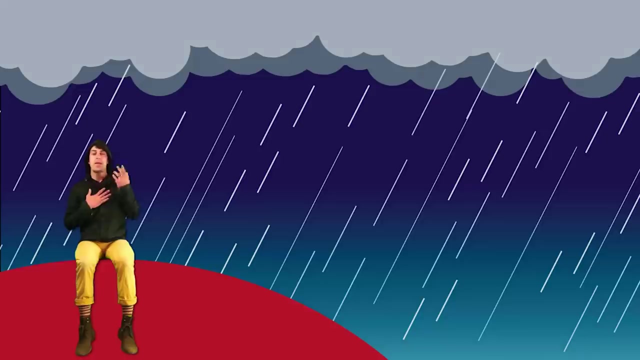 Yeah, that's a C chord. Yeah, Wonder what our next one is gonna be. I hope it's something a little bit prettier than that last cloud. What is it? Yeah, That's our C chord. Here they come: C, E and G. I Love that C chord. 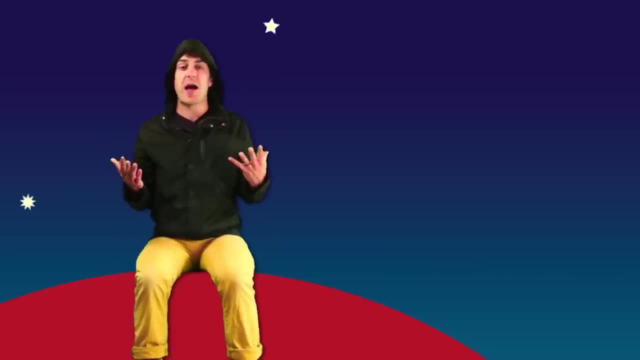 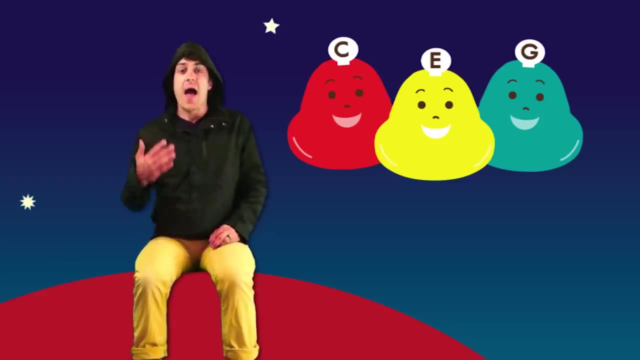 So I guess we're all out of chord clouds to watch for today. You guys can always go back and watch this one again. Put those listening ears on and try to figure out whether you hear a C chord or that thunder cloud, And then just shout it out right away. the faster you can get at identifying a C chord, the better. 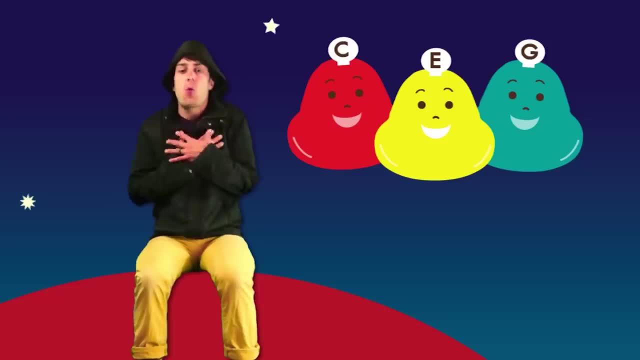 Listening for C chords is really important. This chord is sort of like our home base. It sort of serves as the background for almost All of the music here at the playground. so it's really important that you guys start to recognize this C chord. We'll try adding some new chords in future episodes. 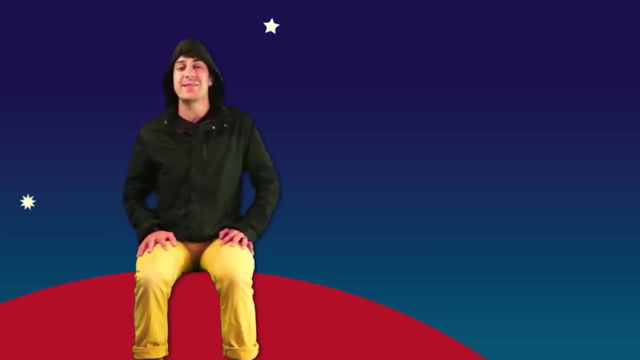 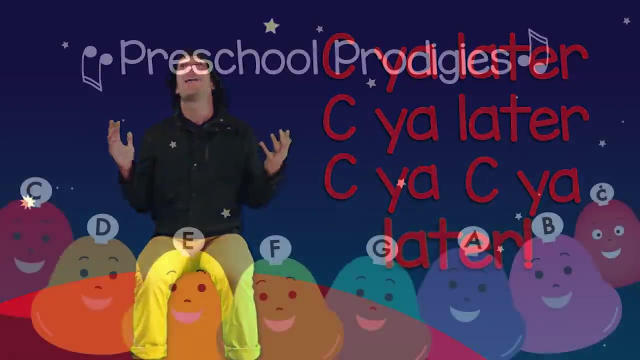 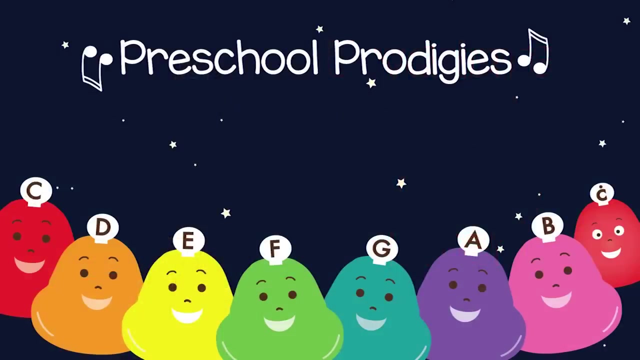 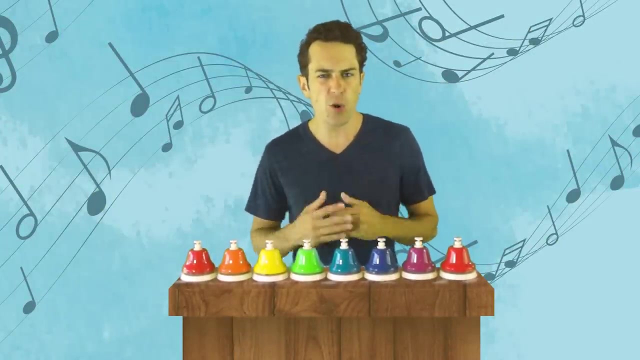 So that's pretty much it for today. I hope you had fun and until next time I will See you later, See you later, See ya, See ya. Nice job with the chord listening. everyone in that chord listening. We saw the notes C, E and G. doh me soul. and in the next listening game. 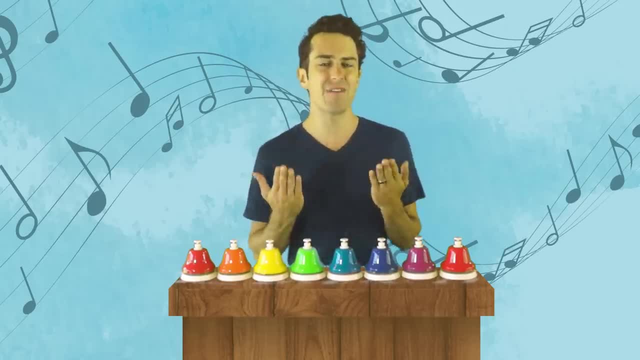 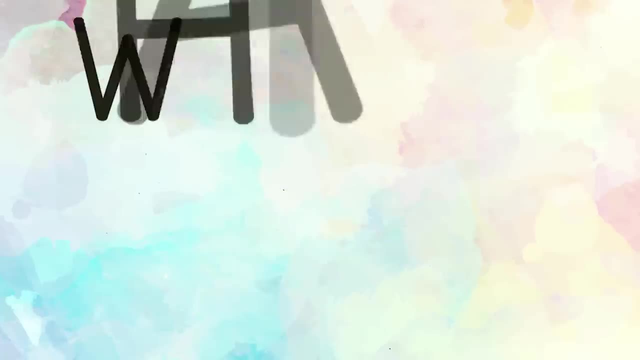 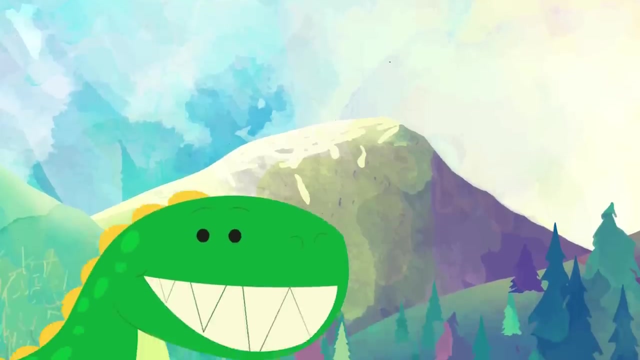 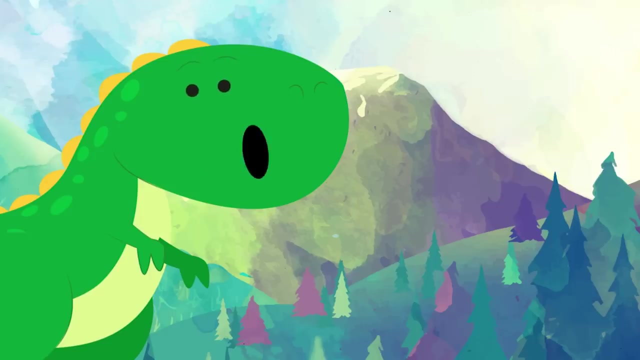 We're going to listen to the notes, one at a time, and see if you can guess what note is it. And now it's time for another episode of everyone's favorite game show. what note is it with your host, this Tyrannosaurus Rex? All right, kids, they're gonna play a note and we're gonna try and guess which one it is. Are you ready? 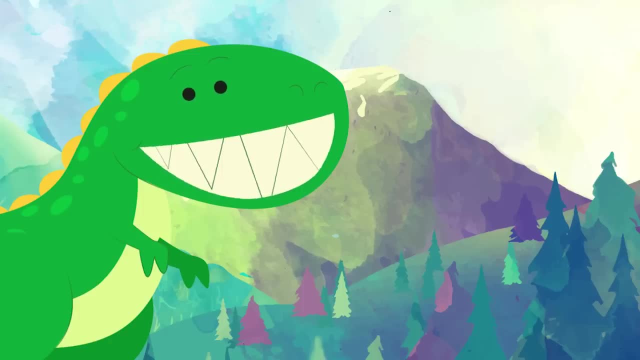 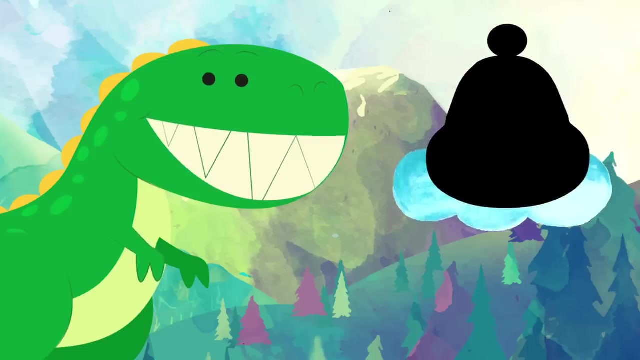 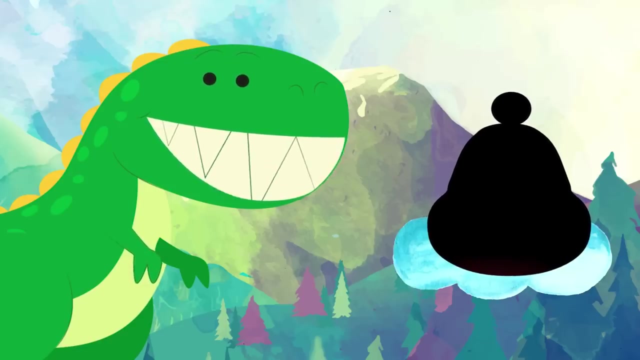 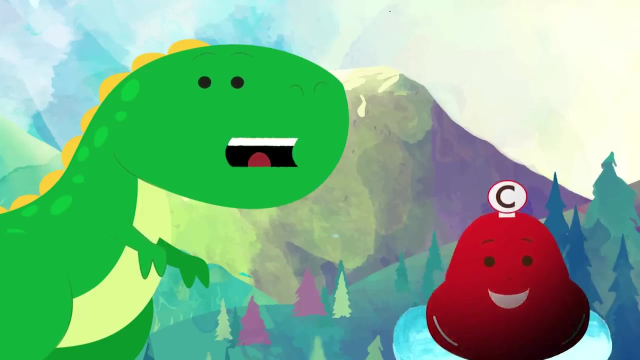 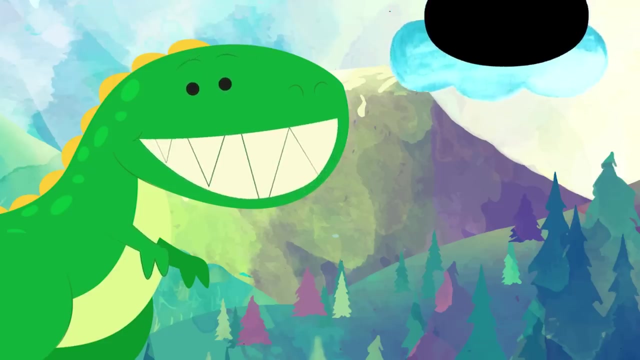 Today you were playing with C, E and G. All right, listen up. What note is it? I Think I've got it And the note is: that's right, It's C. Alright time for round two. let's see what it is. What could it be? 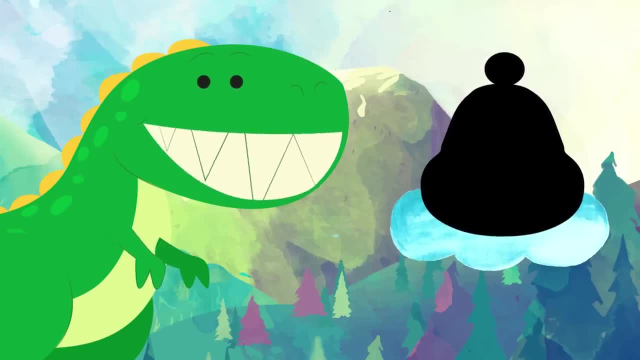 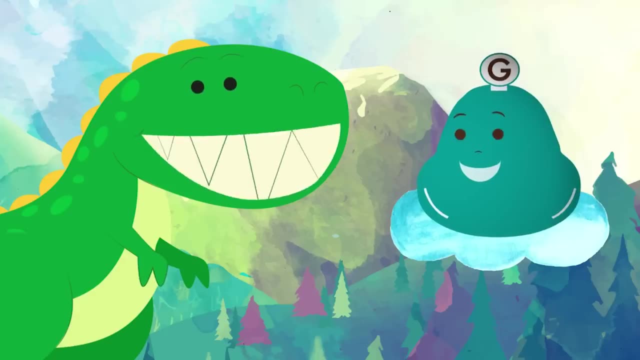 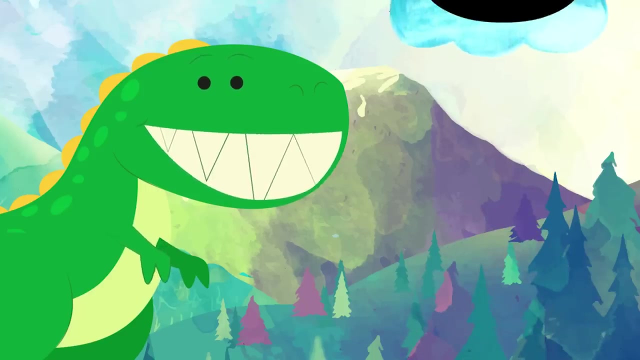 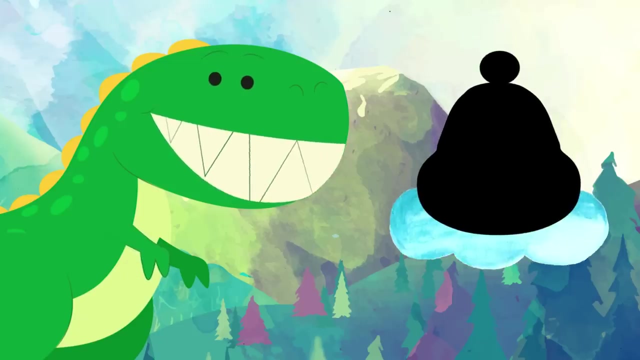 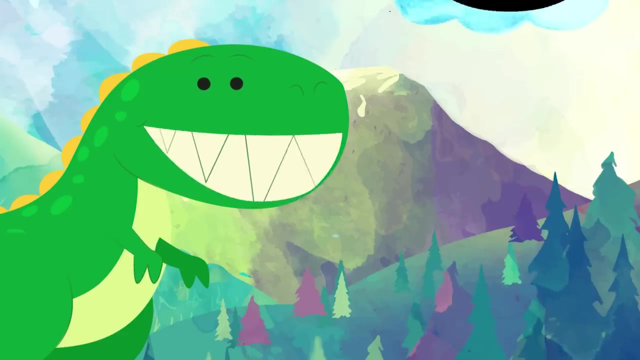 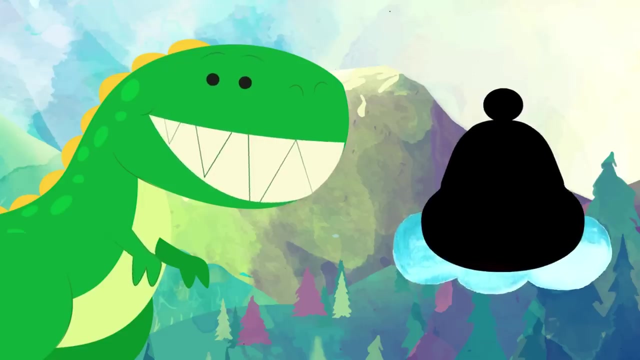 Can you guess? and the note is Good: guess it's G Time for another round. Hmm, I wonder. This one's an easy one and The note is: It was E or me. Here comes another one. Which one is it? I knew I should have practiced, And The note is: 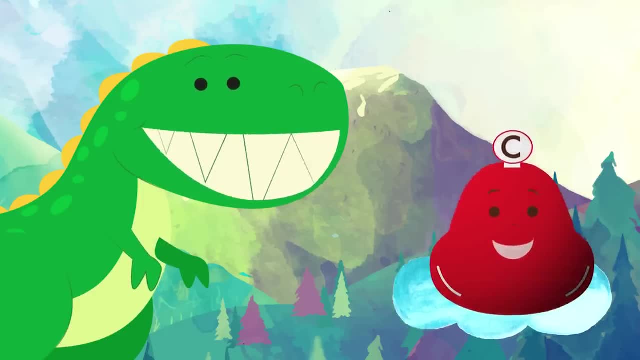 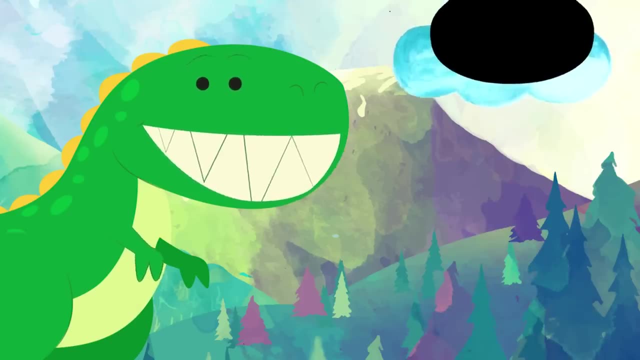 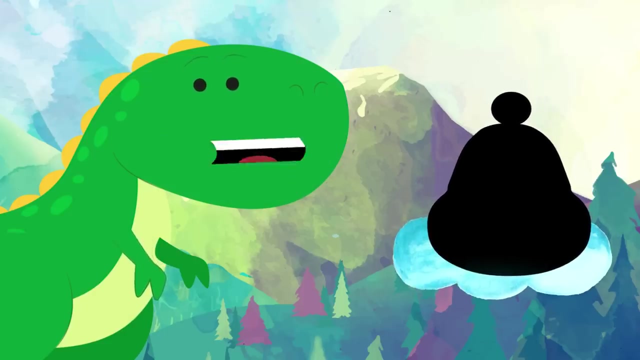 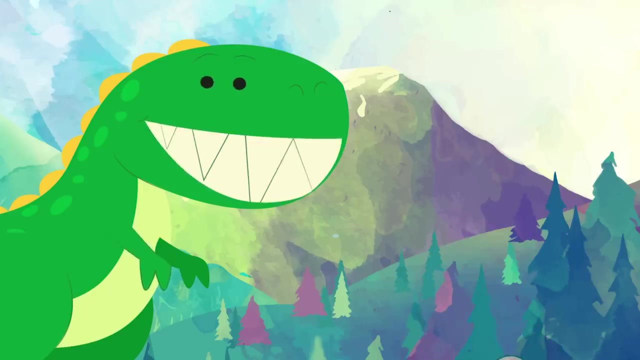 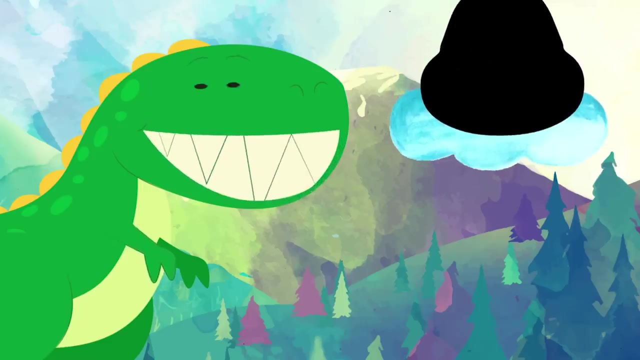 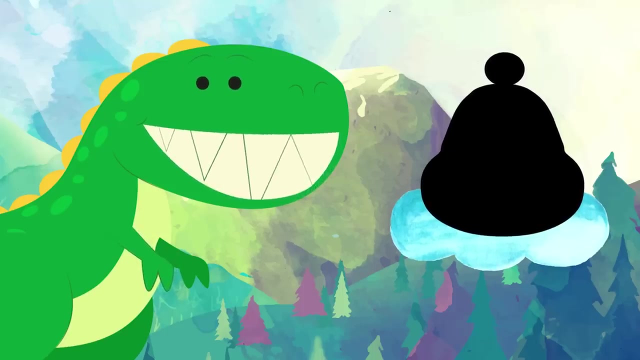 It was C or Doe. Alright, what note is it? This one's a tough one. What do you think it is? And the note is: It was G or so Now for the next round. What note is it, Can you guess? And the note is: 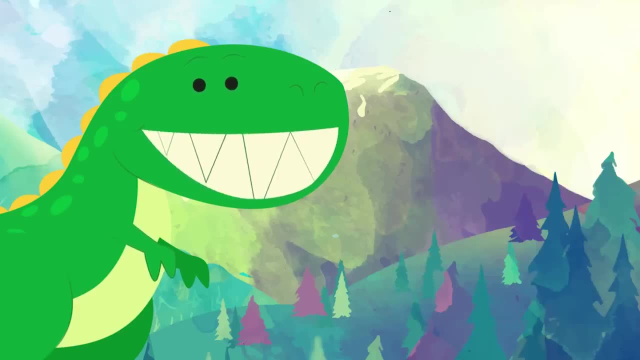 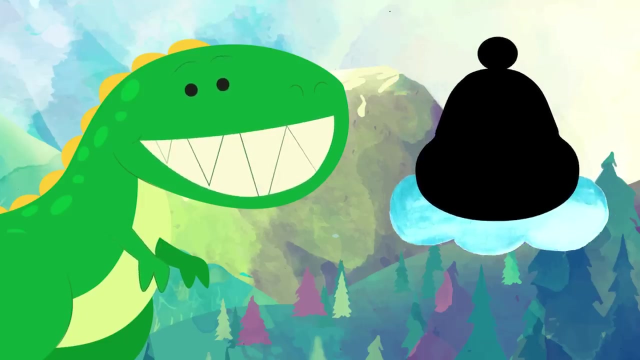 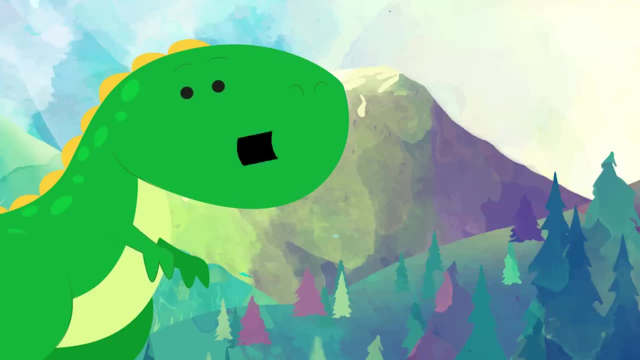 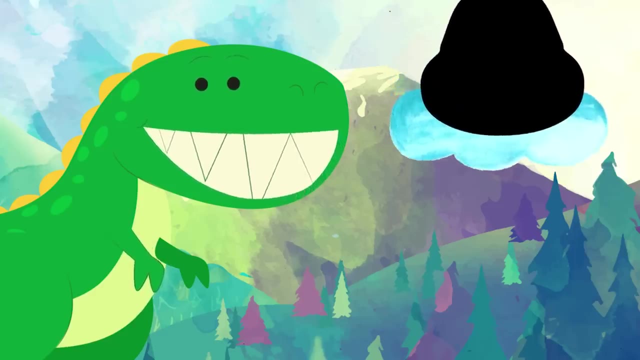 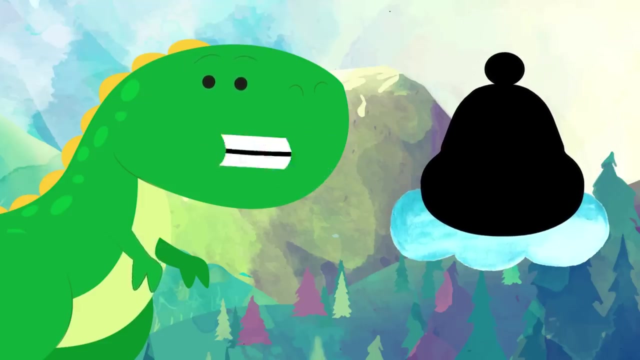 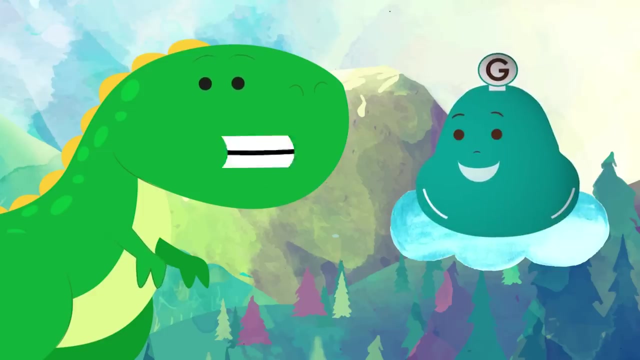 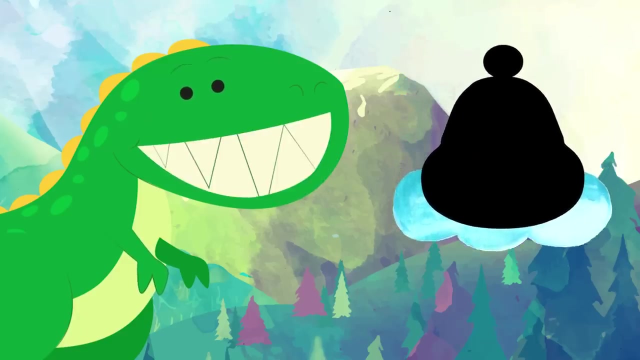 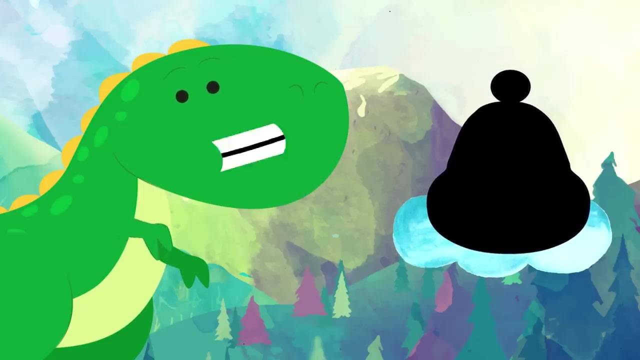 That's right, it's E. Great job, Let's try this next one. Any guess Which one is it? And the note is Good, guess G. Let's see what comes next. What do you think it is? This one's a tough one. 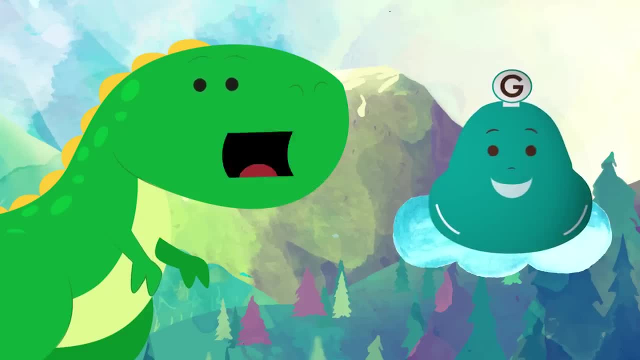 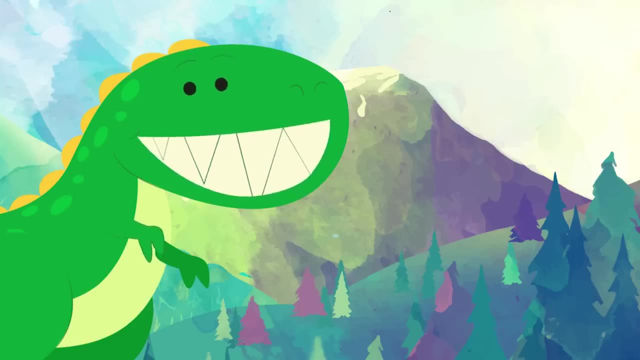 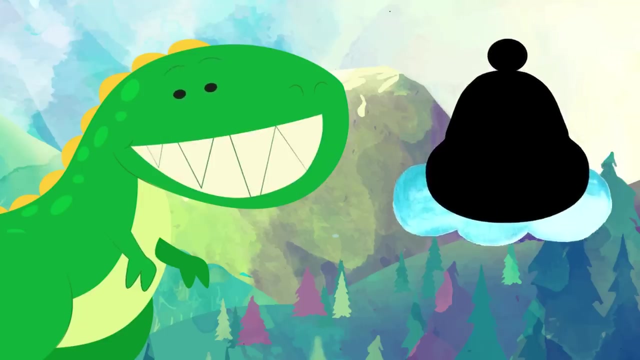 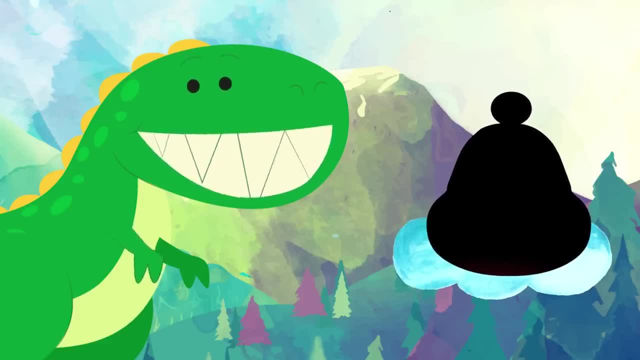 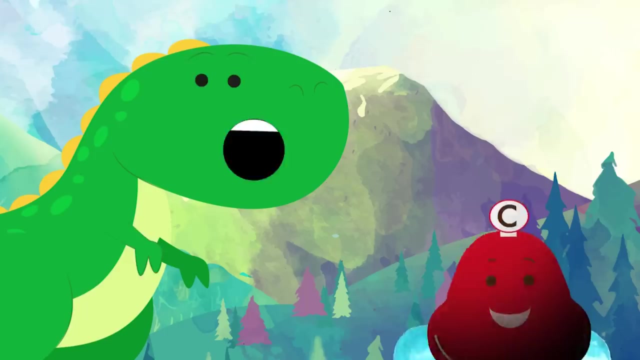 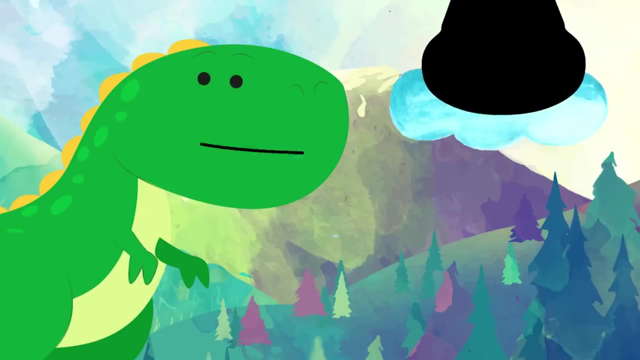 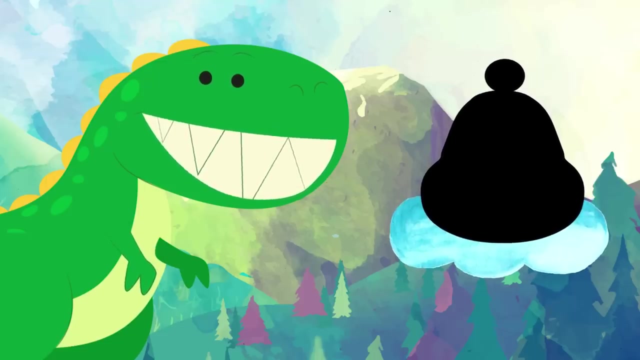 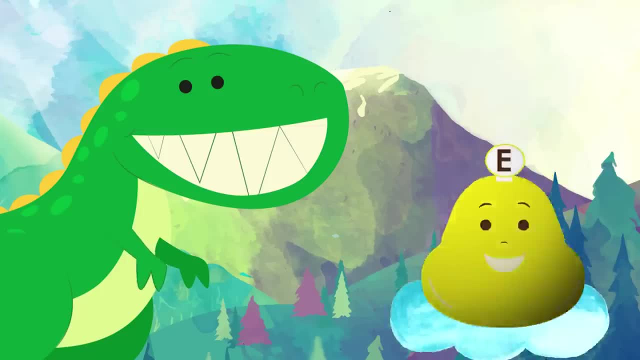 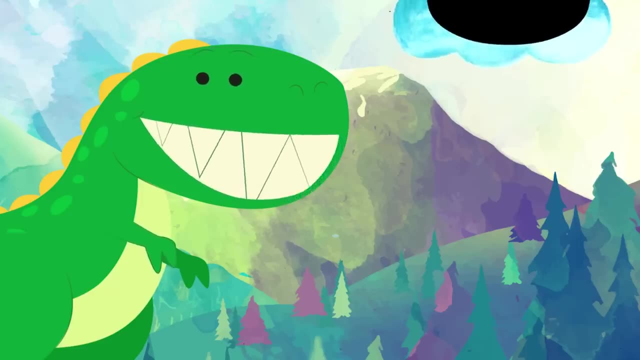 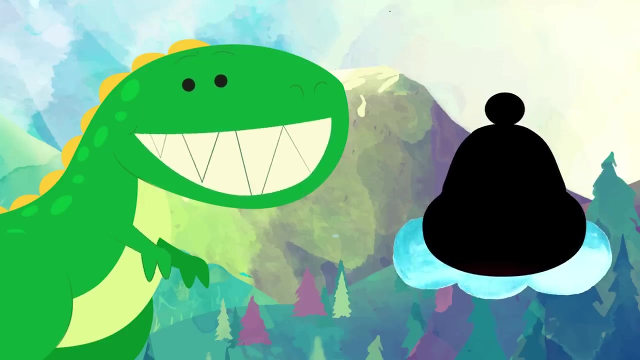 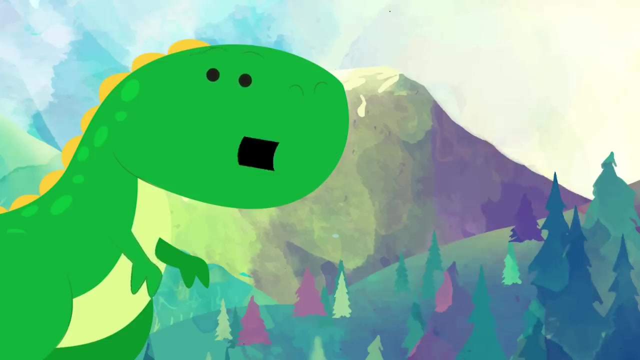 That's right, it's E. Here comes another one. Let's see what it is. This one's an easy one. Which one is it? And the note is Good? guess it's C. And now it's time for the lightning round. 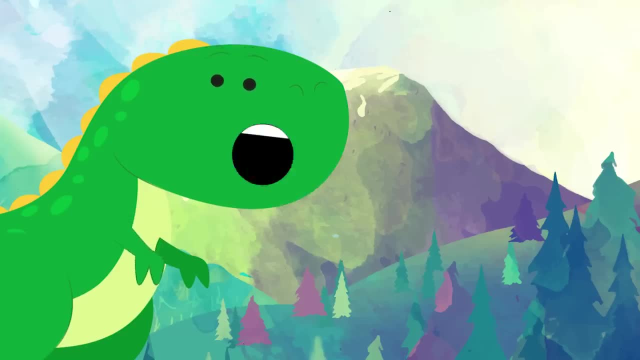 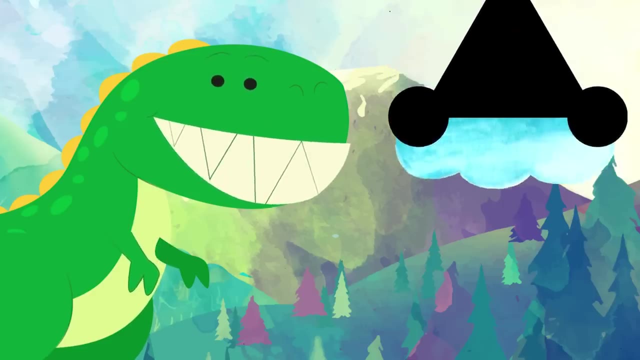 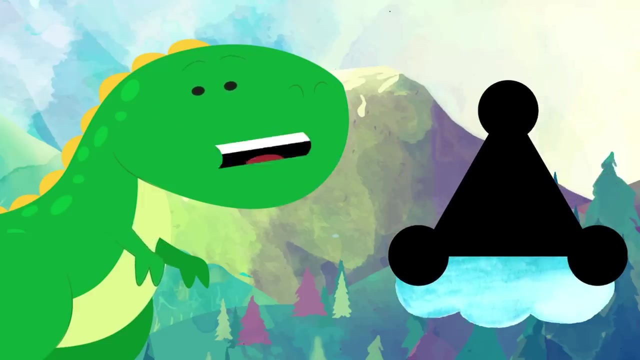 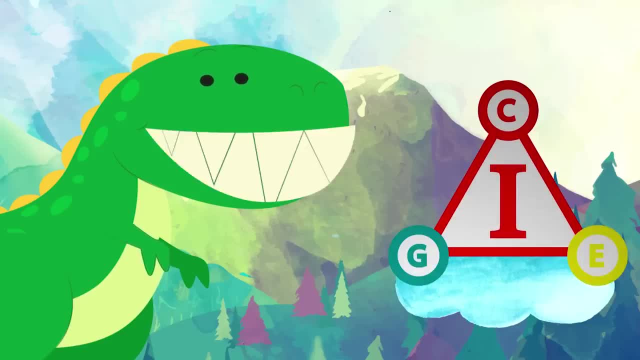 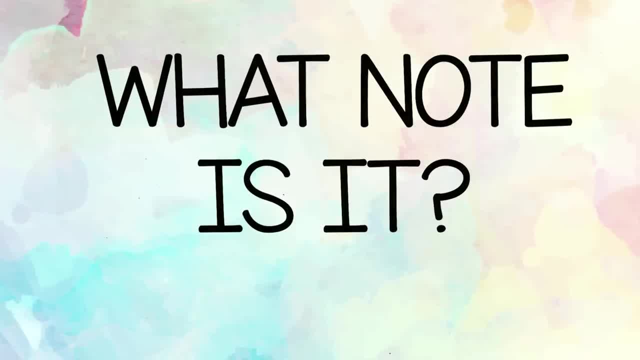 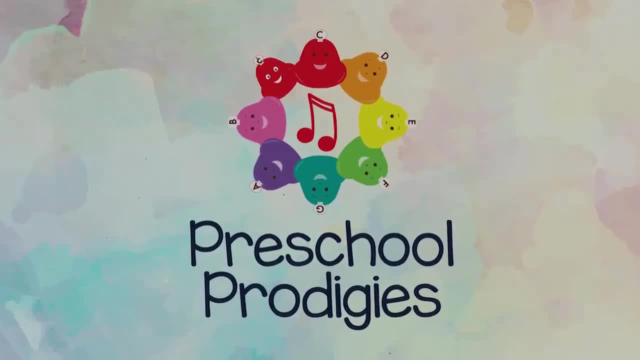 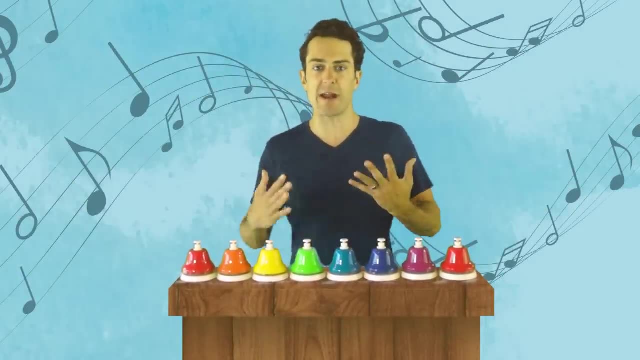 We had a lot of fun and we'll see you here next time. on What Note Is It? Welcome back and nice work. with What Note Is It? That game definitely takes a little bit of practice- practice- to get it right, and you can definitely go back and try it again Now. 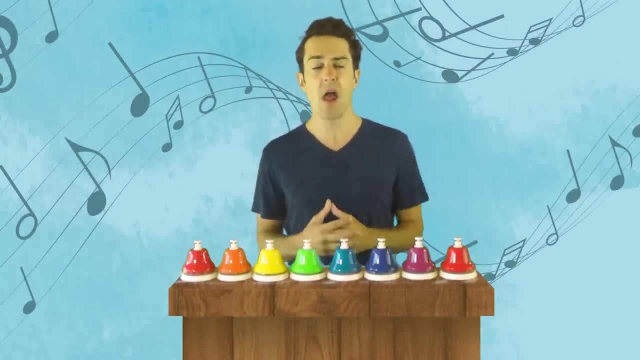 let's mix it up with a little bit more advanced of a rhythm lesson that's called Snow Day. This lesson is a lot like Sweet Beats, but with more complicated rhythms, Plus the bells in this video. have a lot of fun building a snowman. Let's head over to Snow Day for another awesome rhythm lesson from the. 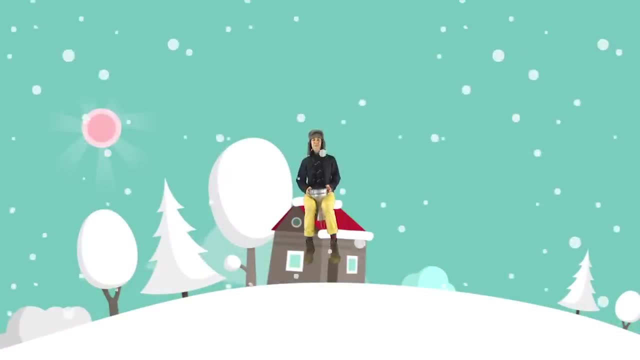 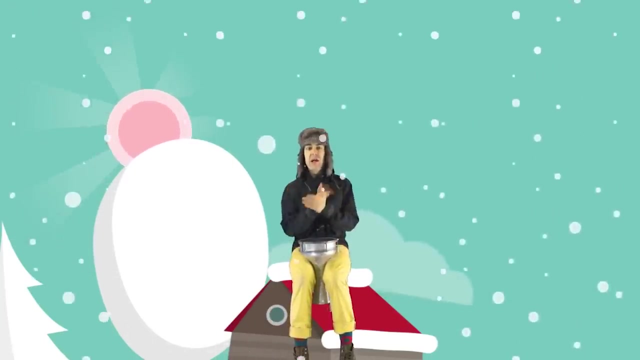 Prodigy's Playground. Hey everybody and welcome to another episode of Preschool Prodigies. My name is Mr Rob and today we're playing a rhythm song about a snow day. If you have a drum, get out your drum. If you don't have a drum, you can follow along by tapping on your legs and clapping your hands. I'm playing on this small drum called a Doonbeck today and you guys can follow along. Let's start out with some nice simple tapping and clapping. So follow me Ready, Tap, clap, tap clap. 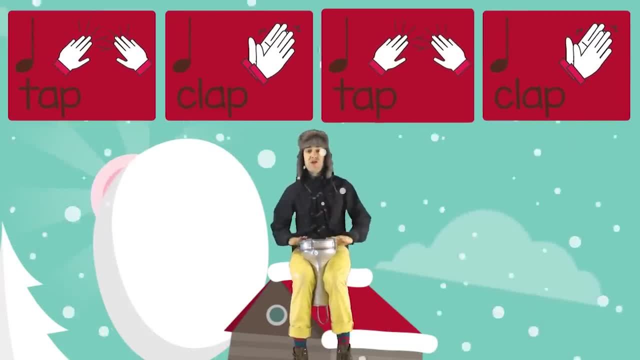 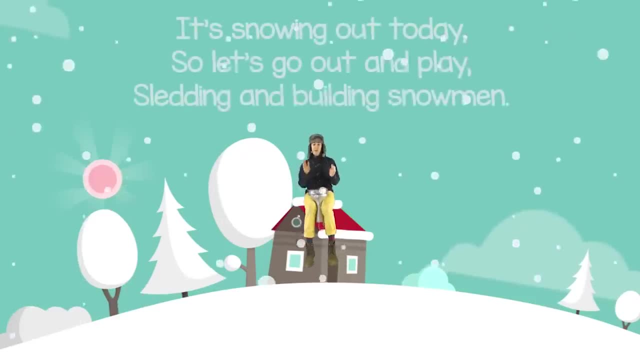 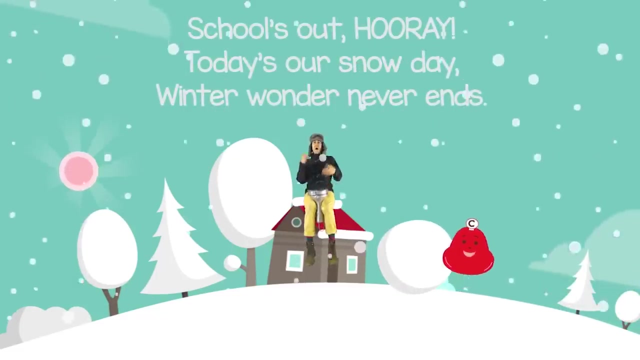 Nice. So we're going to sing a little song about the snow day and then we're going to jump in playing some rhythm And you'll repeat after me. okay, Keep on tapping and clapping. Here's the song part. It's snowing out today, so let's go out and play Steady and building snowmen School's out, Hooray. 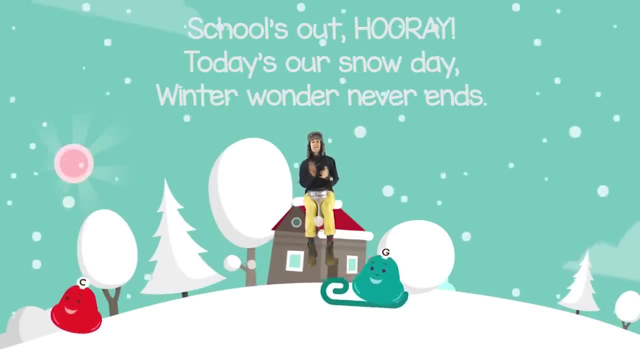 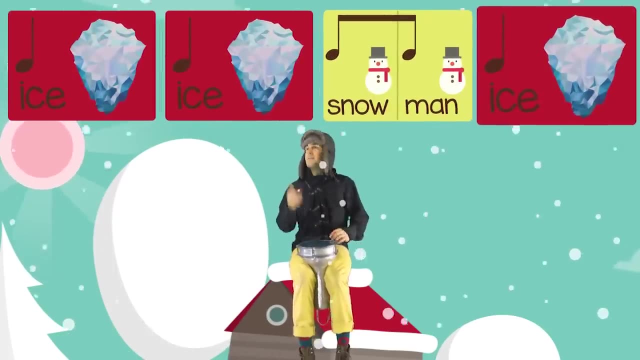 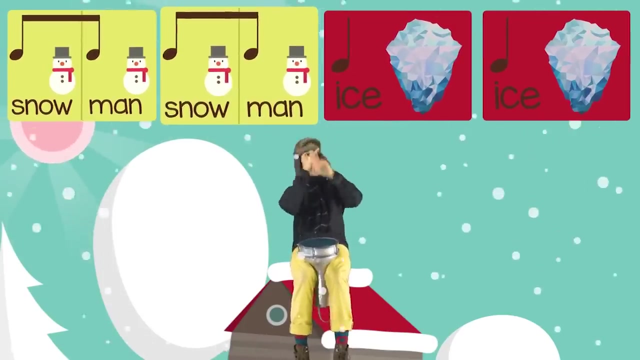 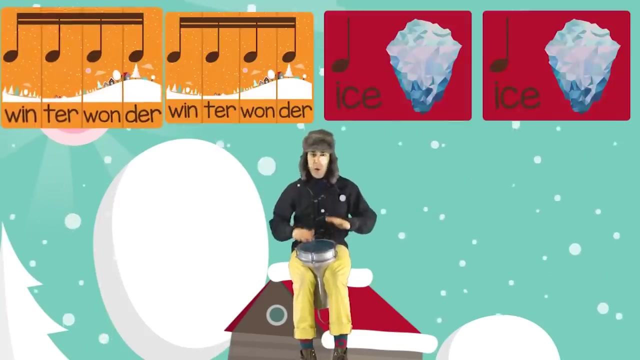 Today's our snow day, Winter one day, Winter never ends. So repeat after me We'll play Ice, ice, snowman, ice, Snowman, snowman, ice, ice, Ice, ice, snowman, ice. A winter wonder, winter wonder, ice ice. 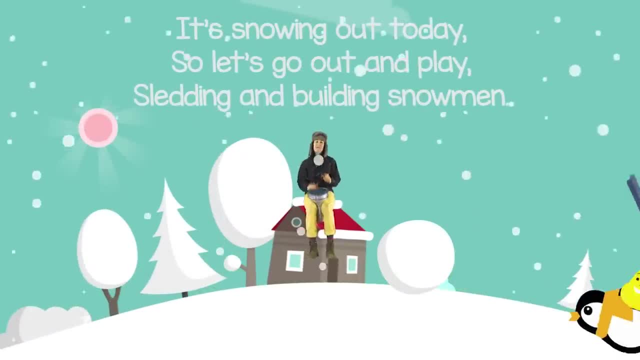 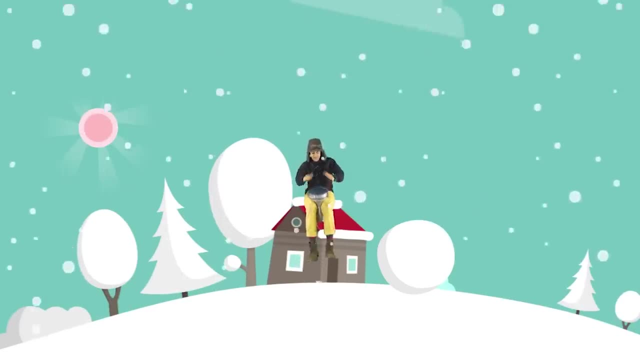 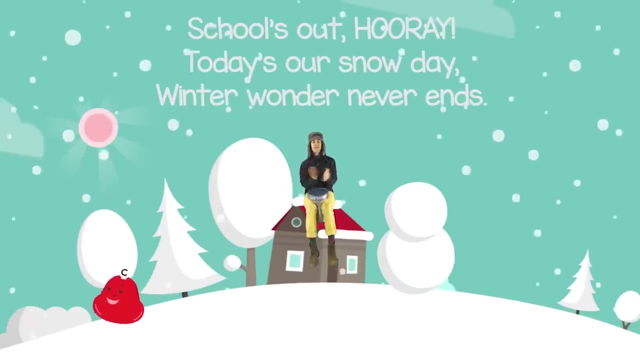 It's snowing out today, so let's go out and play, Steady and building snowmen. Study and building snowmen. School's out, Hooray, Today's our snow day, Winter one day. The winter wonder never ends. Repeat after me. 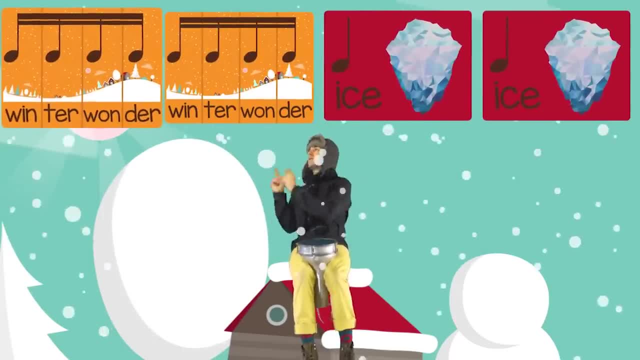 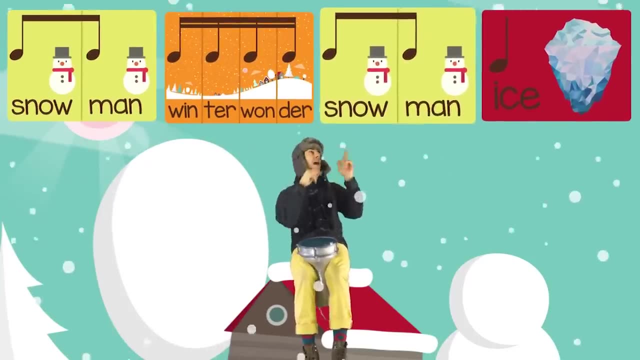 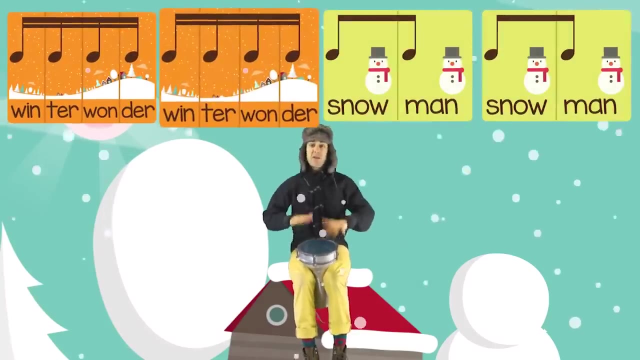 A winter wonder, winter wonder, ice ice. winter wonder, wonder Ice ice snowman. winter wonder, snowman ice, snowman, ice ice. Winter wonder, winter wonder, winter wonder, snowman snowman. winter wonder, winter wonder snowman. 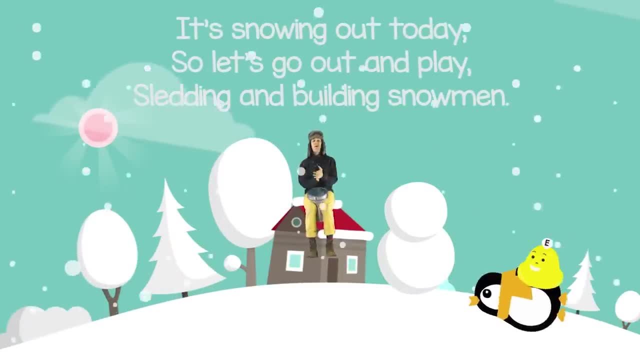 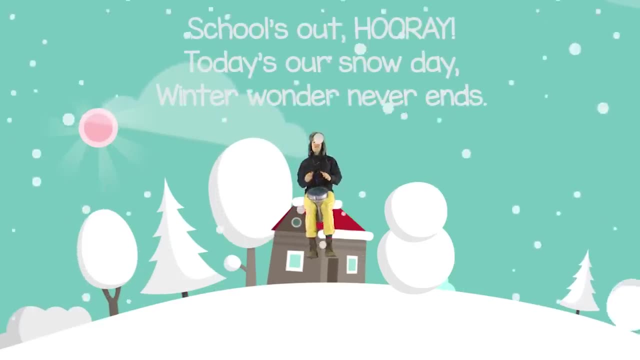 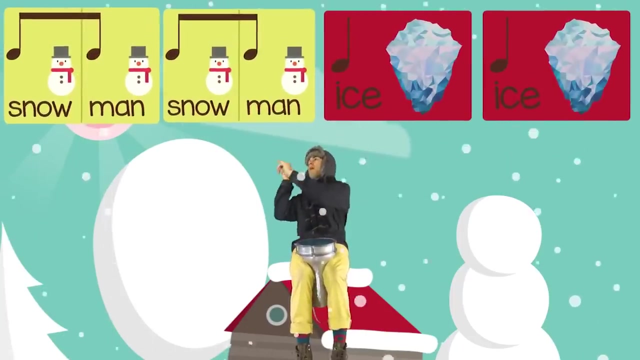 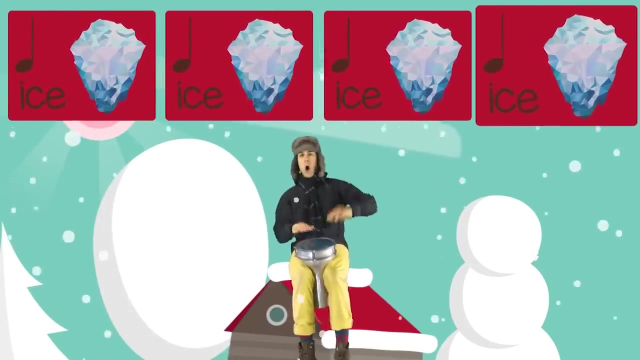 It's snowing out today, so let's go out and play sledding and building snowmen. School's out. hooray, today's our snow day. the winter wonder never ends. Repeat after me: snowman, snowman, ice, ice, ice, ice, ice, ice, snowman, snowman, snowman, snowman. 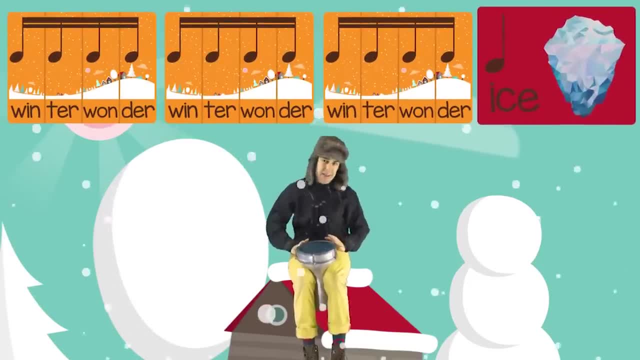 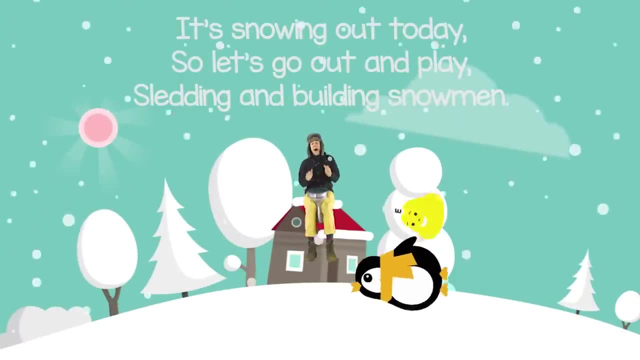 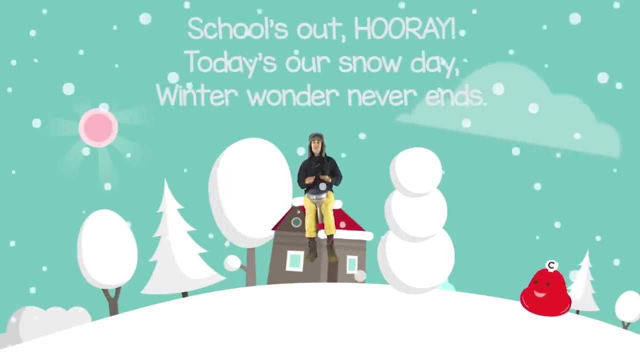 Nice and fast. winter wonder. winter wonder. winter wonder. ice Last time. it's snowing out today, so let's go out and play sledding and building snowmen. See if you can tap a little faster School's out. hooray, today's our snow day. the winter wonder never ends. 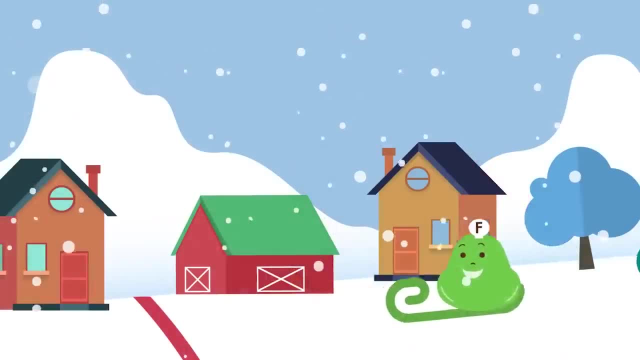 Nice job, everybody. give yourselves a huge round of applause. Great job playing with all these different rhythms here on our snow day, Alright, so welcome back. So far, a lot of the music has been great. So far, a lot of the music has been great. 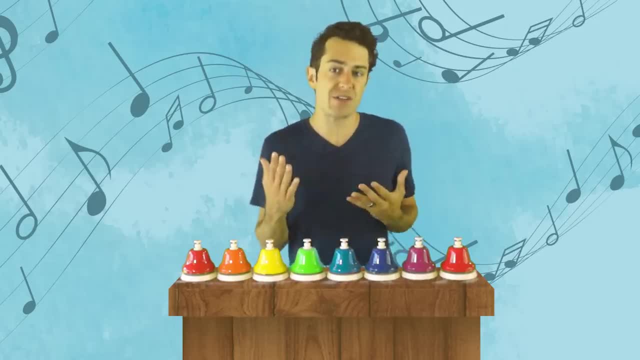 All the music that we've been reading has been pretty simplified or uses images like the beat or the cherry or the snowman, And now we're going to look at some real sheet music, some real scrolling sheet music inside of PSP, Melodies Number Nine and Ten. 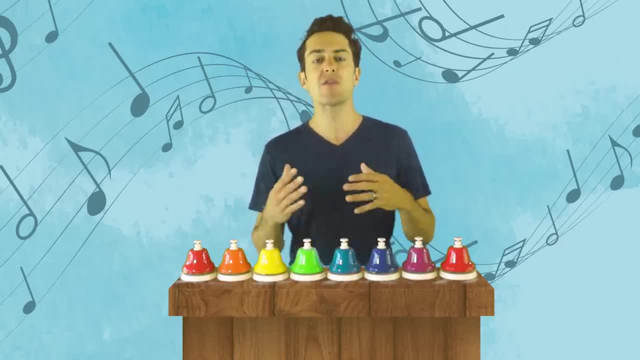 Both of these lessons feature the more advanced scrolling sheet music that we use inside of level two of the Playground, Primary Prodigies. Primary Prodigies is designed for the elementary school learner kids between 5, 6,, 7,, 8,, 9,. 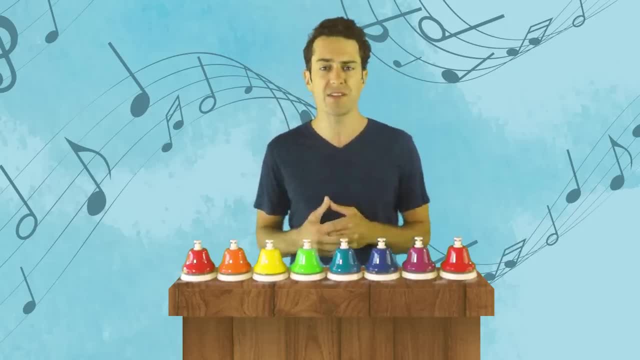 10. awesome, awesome follow-up to Preschool Prodigies, and it's also sort of a program that you can do all on its own, because it starts out with a lot of review of the concepts that we did inside of Preschool Prodigies. Alright, 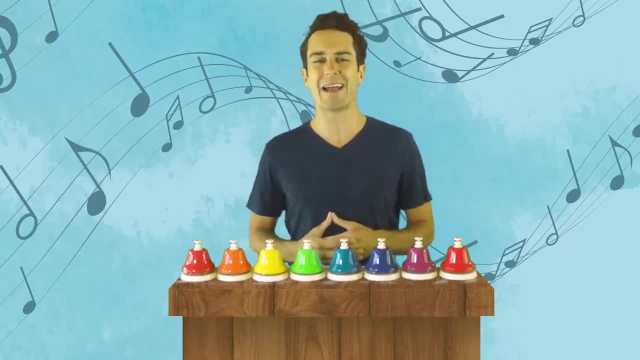 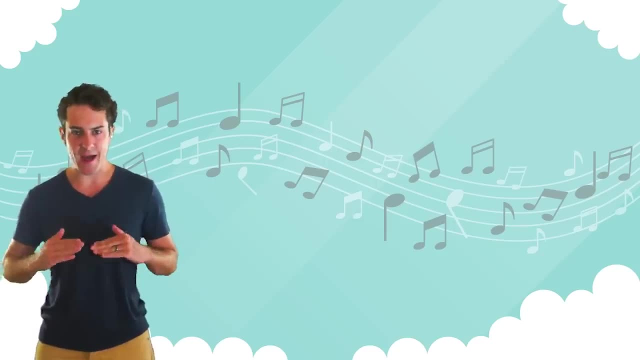 well, without any further delay, let's check out PSP Melodies number 9 and 10.. Hey everybody, and welcome to PSP Melodies number 9.. Today we're gonna be singing and hand signing with some whole notes, half notes and quarter notes on. 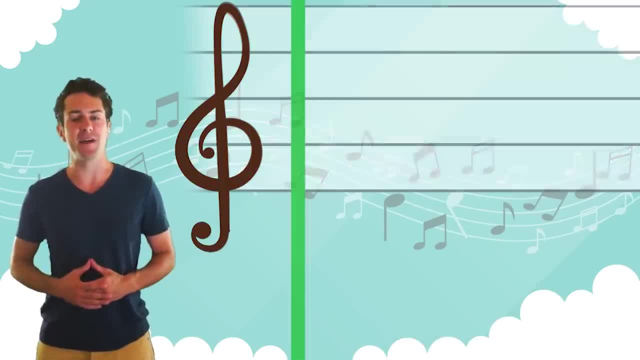 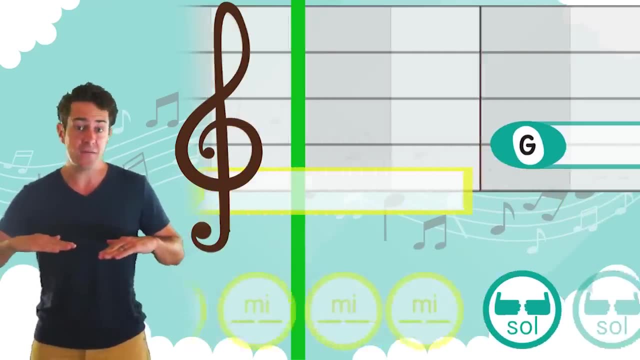 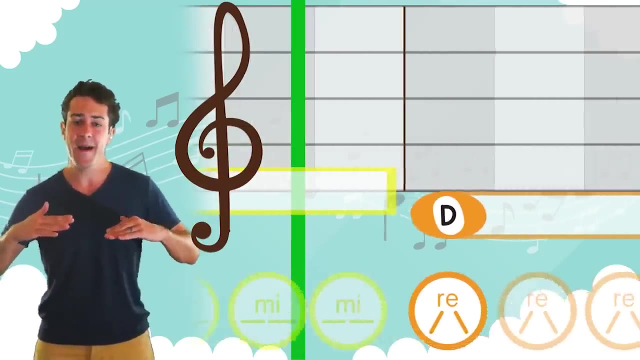 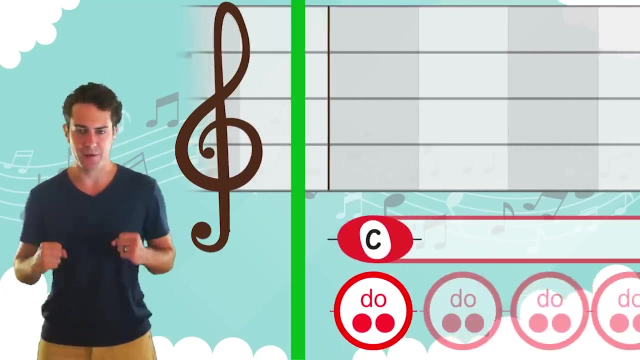 the treble clef. This is gonna be reading some real sheet music and we'll start out with a nice low do to start. Do for the whole measure Mi for the whole measure Sol. Nice, Ba back down to mi, Re down to do Nice. Let's try that again together. Ready set do. 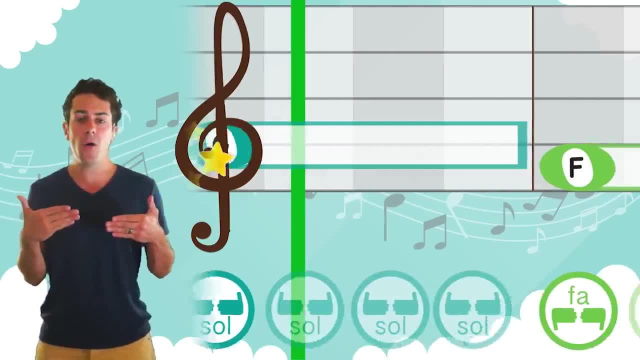 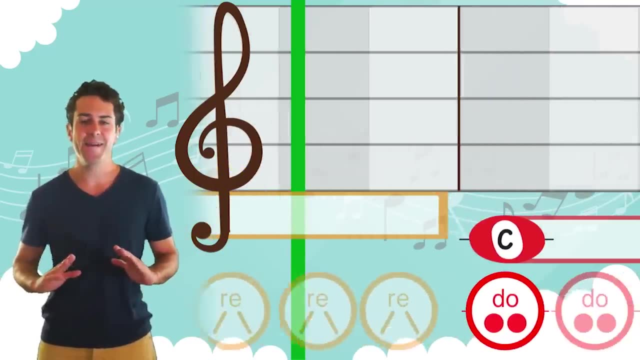 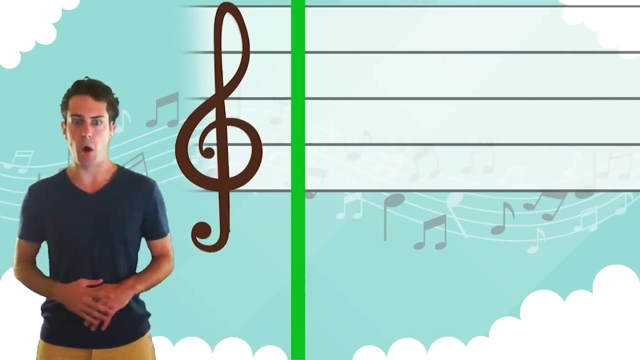 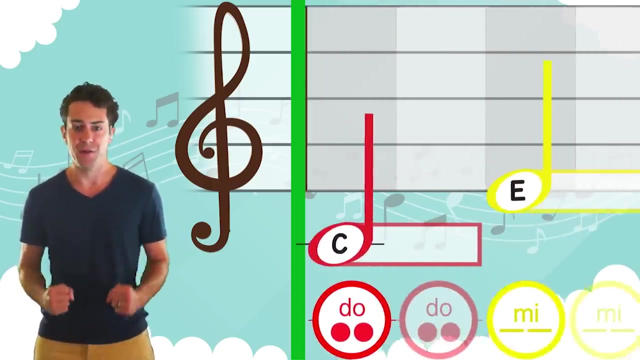 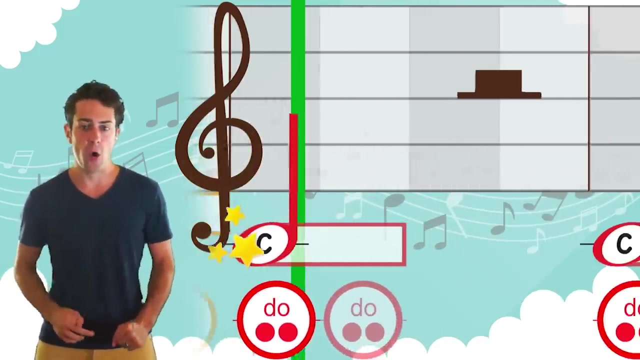 Mi Sol Fa Mi Re Do. Hey, nice job with that. So those are the whole notes that take up the whole measure. We're gonna play a little bit faster with some half notes Ready. Do Mi Sol Fa Mi Re, Do You do it? 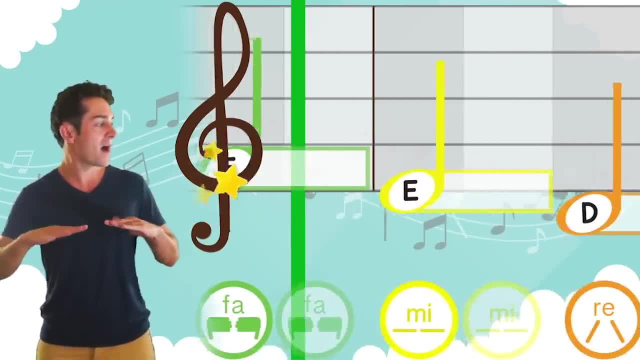 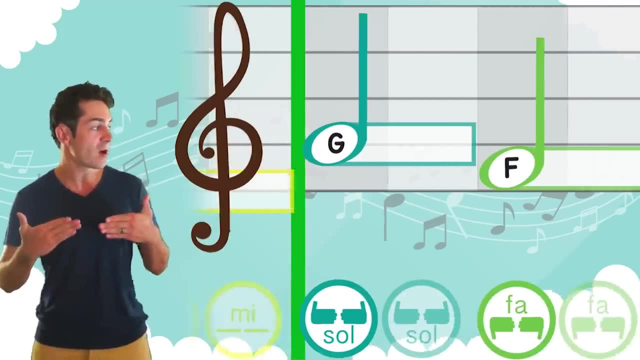 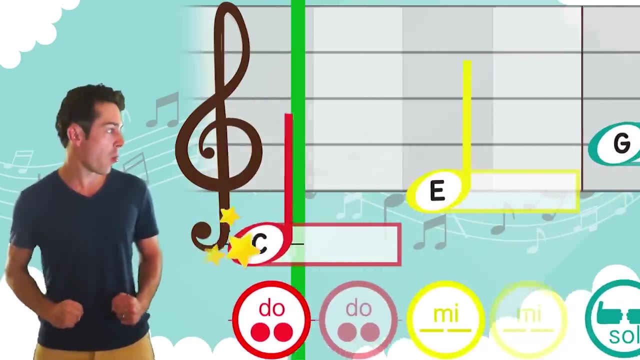 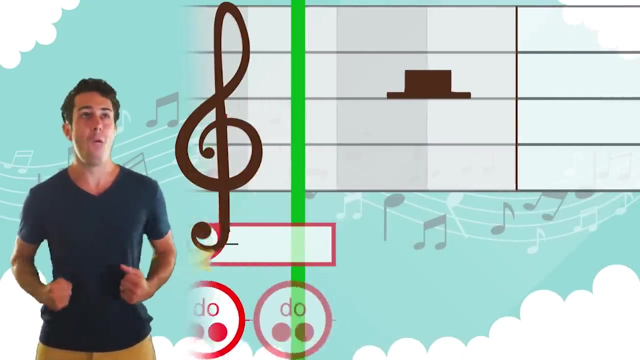 Altogether nice and loud. Do Mi Sol Fa, Mi Re Do One more time, just like that. Do Mi Sol Fa, Mi Re Do. Alright, we're gonna try it even faster using some quarter notes. 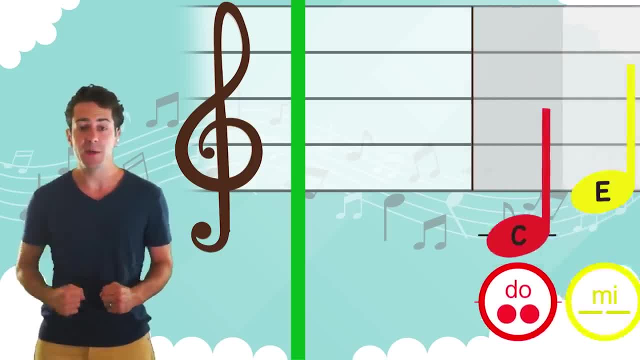 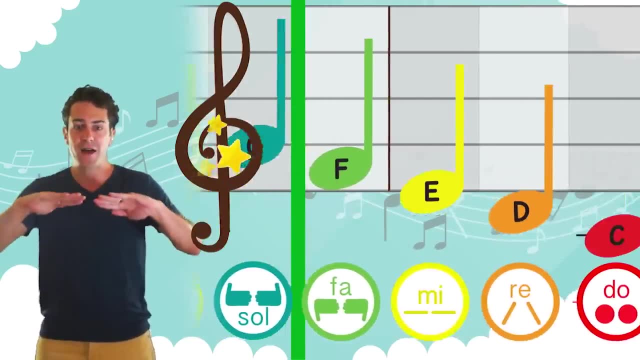 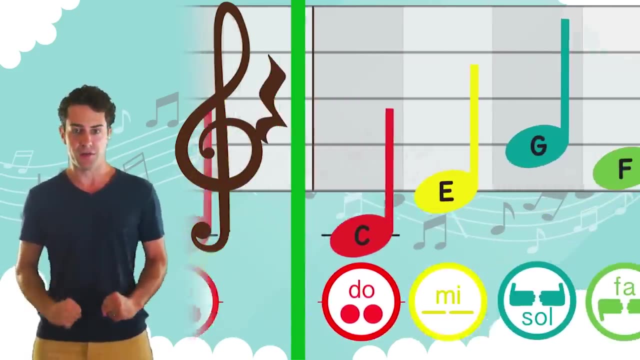 It's gonna be pretty quick. okay, One, two, here we go. Do Mi Sol Fa Mi Re Do Again. Do Mi Sol Fa Mi Re Do Two more. Do Mi Sol Fa Mi Re Do Last one. Do Mi Sol Fa Mi Re Do. 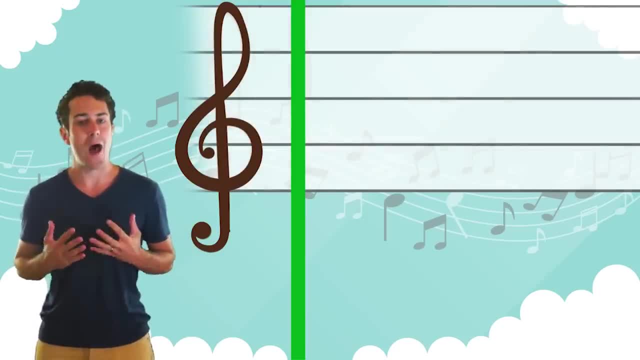 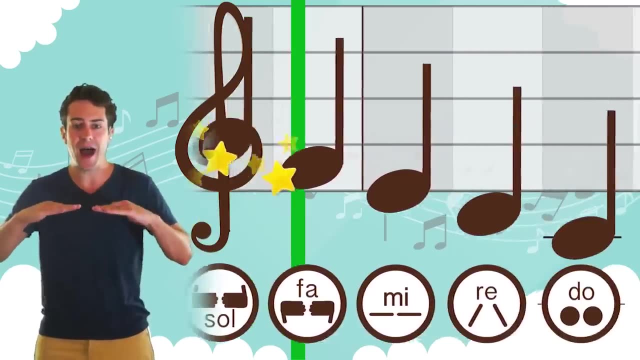 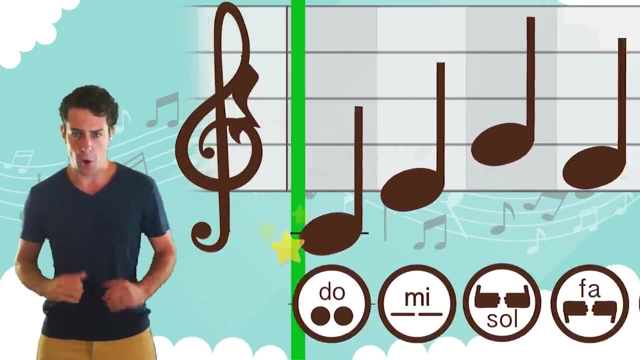 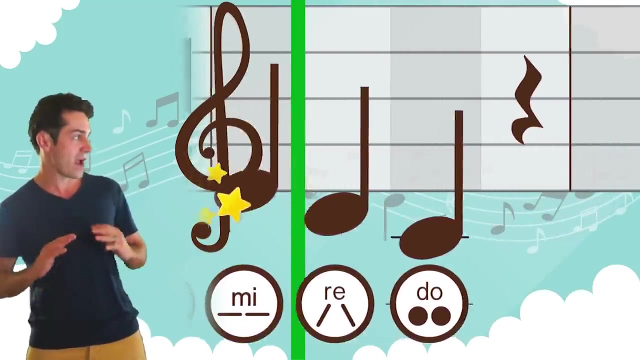 Now we're gonna do it one more time today, without the color-coded music Ready. Here we go. Do Mi Sol Fa Mi Re Do. Do Mi Sol Fa Mi Re Do. Do Mi Sol Fa Mi Re Do. Last time. Do Mi Sol Fa Mi Re Do. 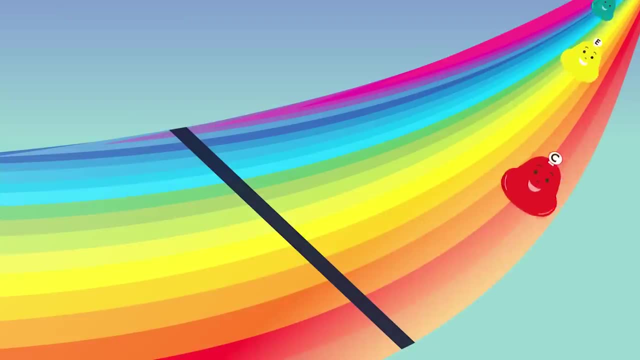 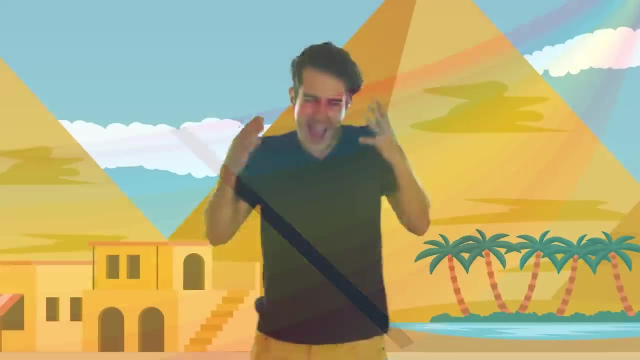 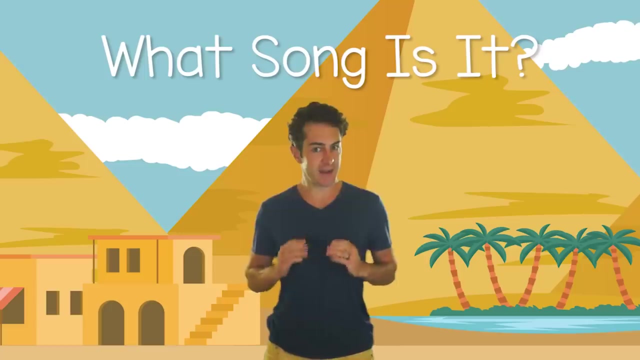 Give yourself a huge round of applause. Nice job with PSP Melodies 9: everybody, Hey, everyone, and welcome to PSP Melodies number ten. Today we're playing a round of What Song Is It We're gonna sing and hand sign some melodies and you have to tell me what song we're singing. So we're gonna start out. 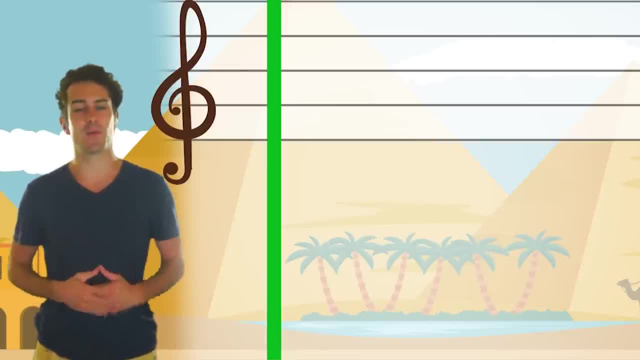 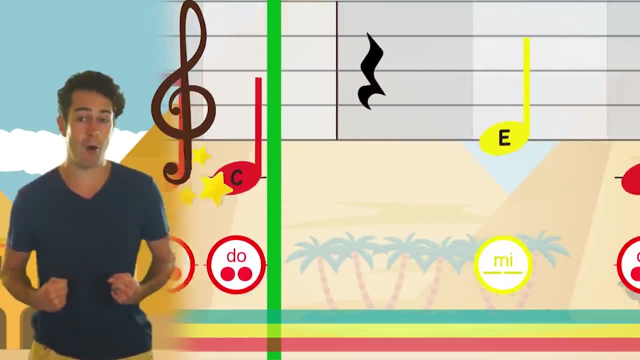 with this one today. Put on those listening ears, get out those hand signs and we'll start on a nice low-do You ready? Here we go, Do, do, do, do, do, do, do Mi do, Re re rererere Mi do. 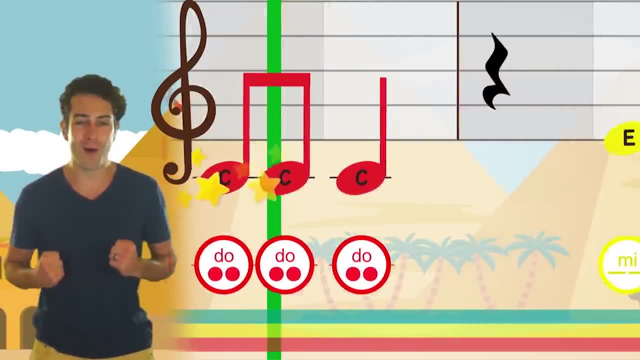 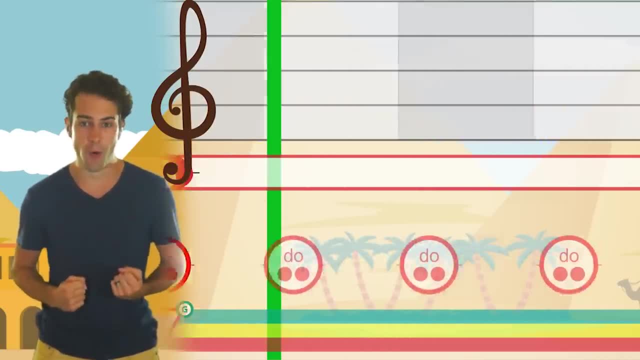 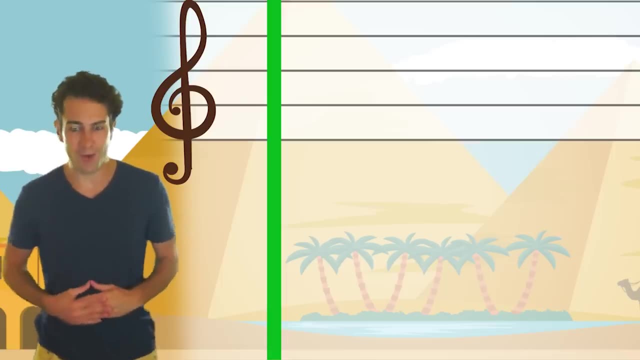 Doe, doe, doe, doe, doe, doe, doe me, doe, doe me, ray, ray, doe. Do you know what song it is, Do you? It's about a camel. The words are going to come this way: 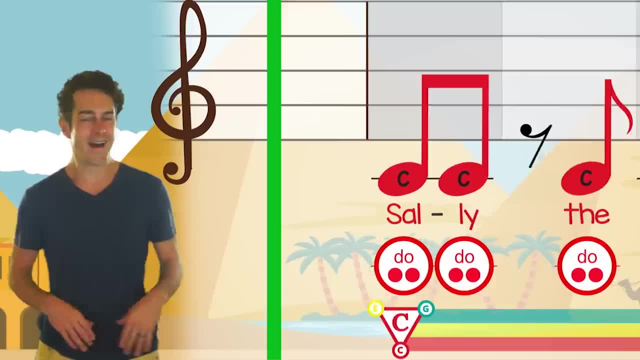 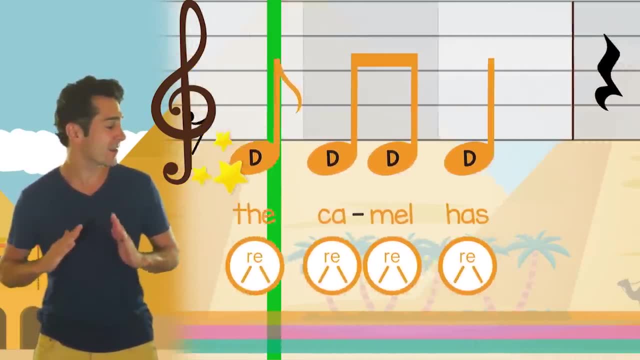 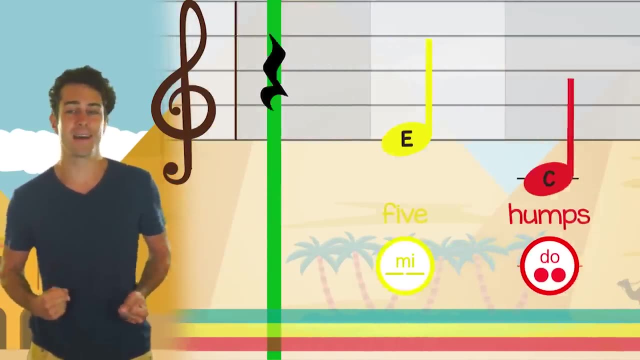 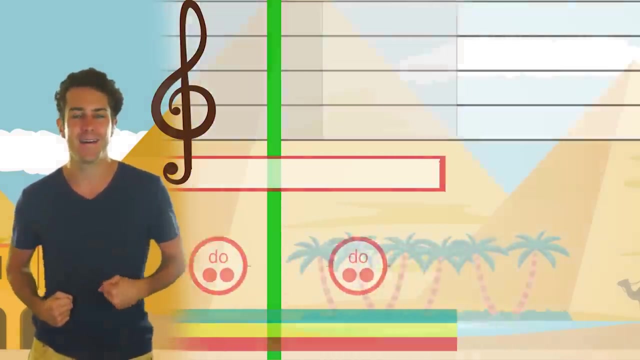 We can sing the words and it will tell you what song it is Ready. Sally the camel has five humps. Nice, Sally the camel has five humps. Sally the camel has five humps. So ride, Sally, ride. Hey, nice job with that song everybody. 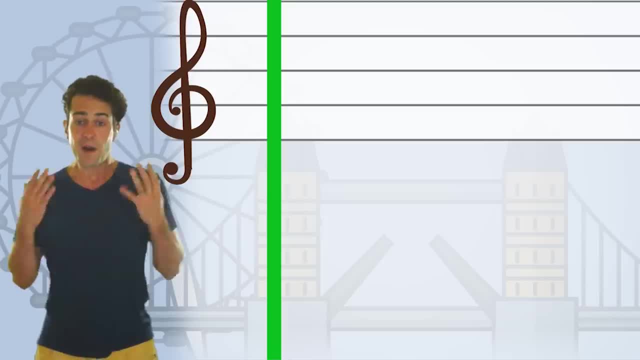 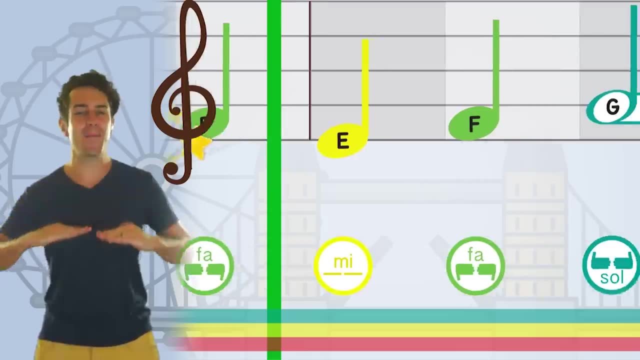 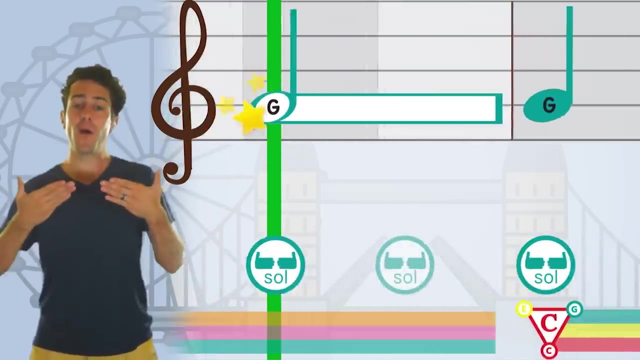 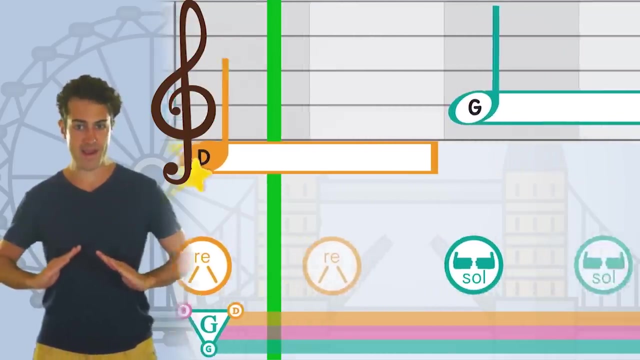 Let's head over to the next one. All right, we're here in the next song. I wonder what it's going to be Ready set. Sol la sol fa mi Fa, sol re mi fa mi fa sol. sol la sol fa mi fa sol re sol mi do. 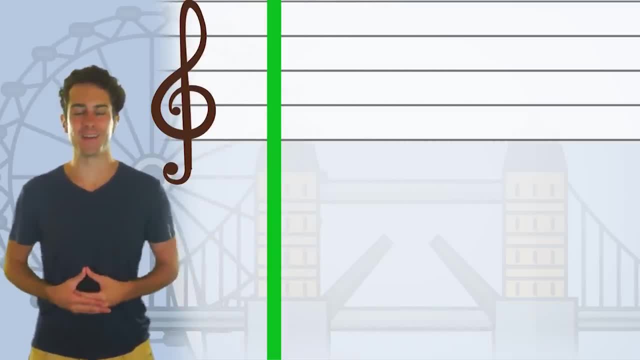 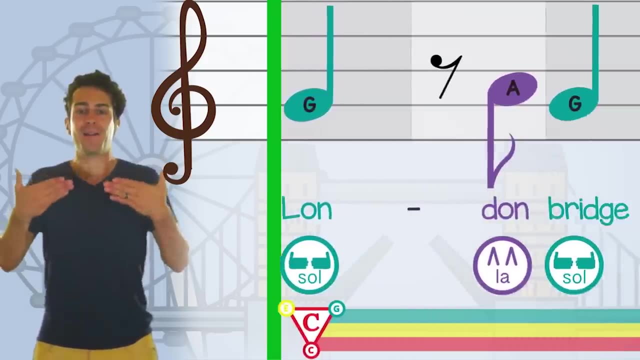 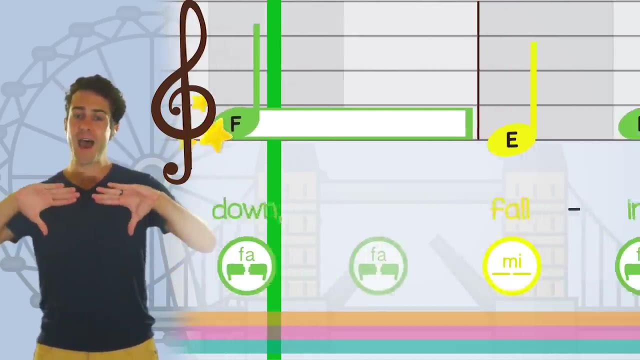 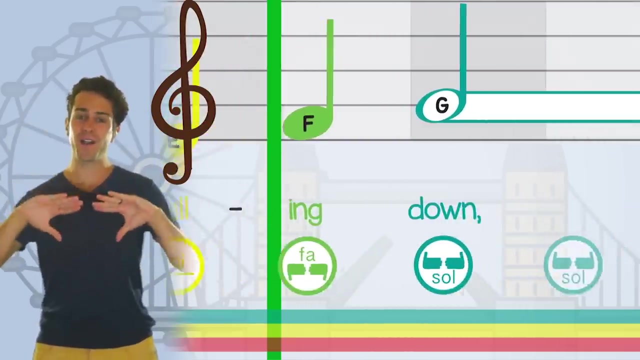 Do you know what song that one is? Yeah, you do. That's an easier one. That's a London Bridge. It's falling down. Let's try singing and hand signing with the actual lyrics: London Bridge is falling down, falling down, falling down. London Bridge is falling down, my fair lady. 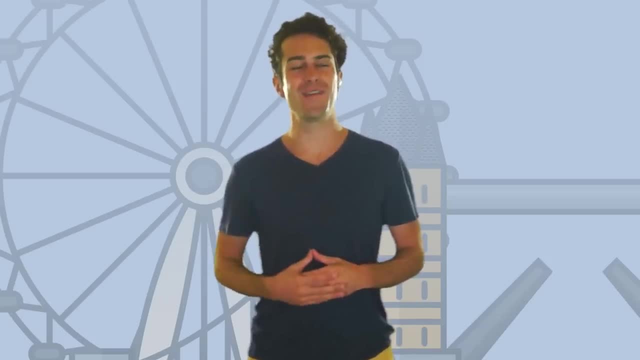 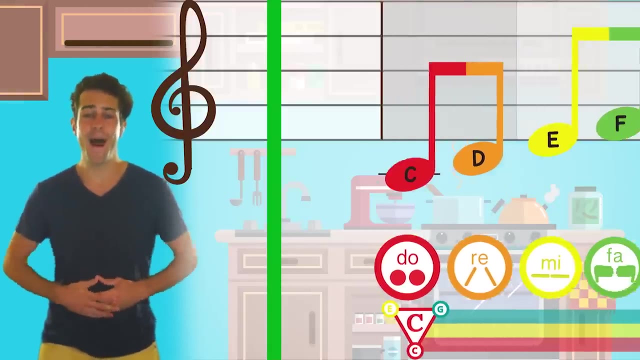 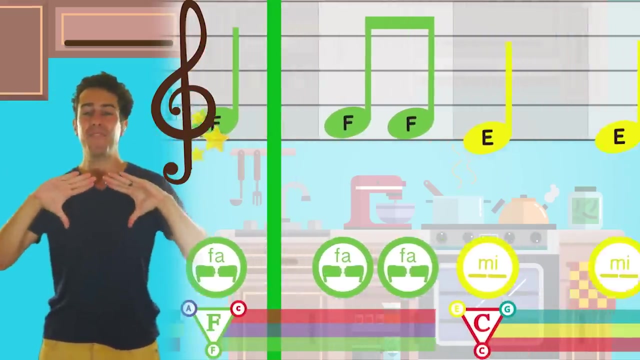 Hey, nice job with London Bridge, everybody. Let's head over to the next song. All right, we're ready for the next song. One, two Ready. Do re mi fa sol do la do sol, fa, fa fa mi mi re re re do. 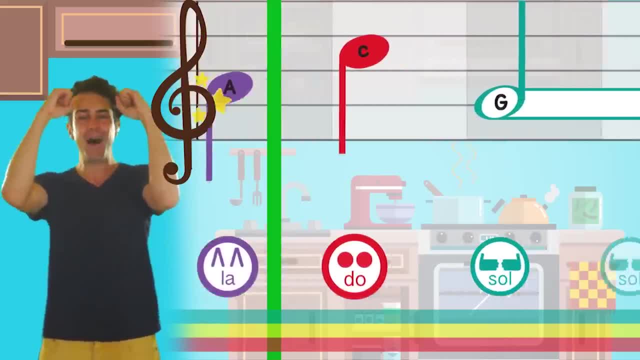 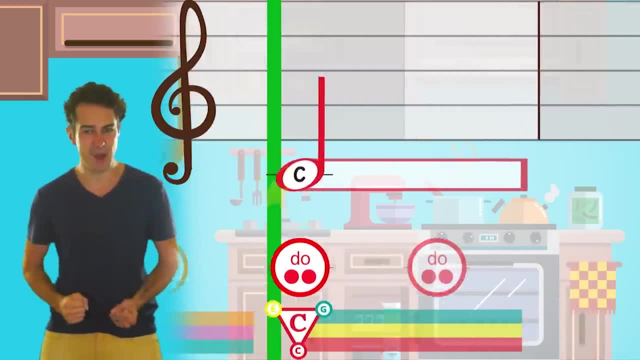 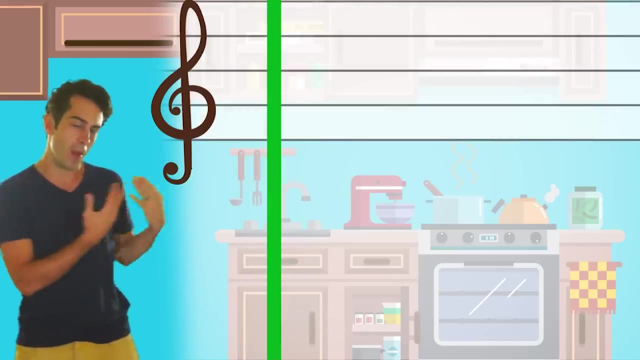 Do re mi fa sol, do la do sol. do la sol sol fa mi re do. Do you know what song it is? It's another pretty distinct melody. When the lyrics come this way and scroll by, we're going to sing and hand sign. 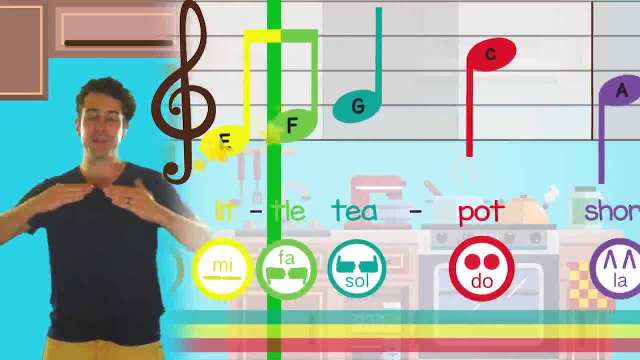 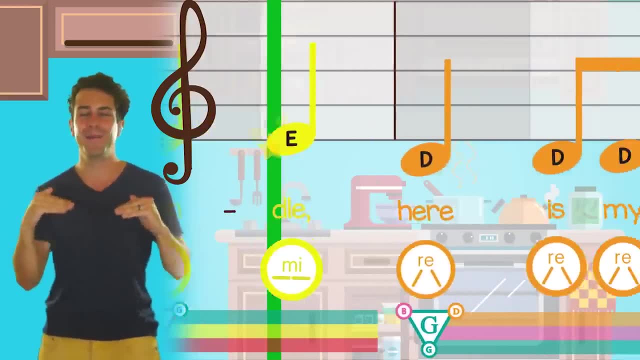 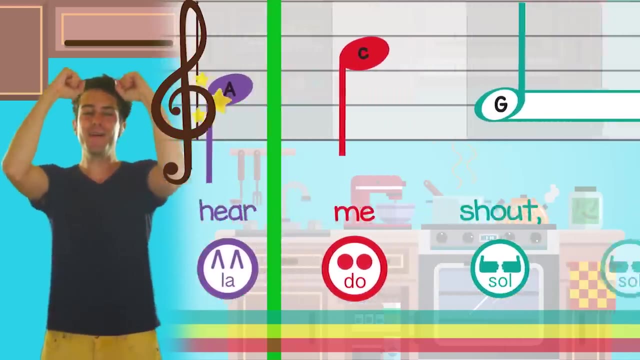 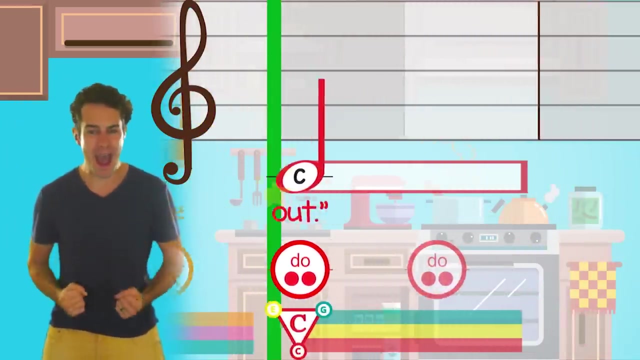 Ready, Here we go. I'm a little teapot, short and stout. Here is my handle, here is my spout. When I get all steamed up, hear me shout, Tip me over and pour me out. Yeah, that was, I'm a little teapot. 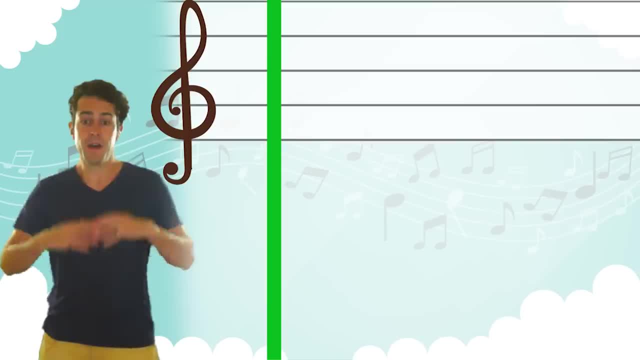 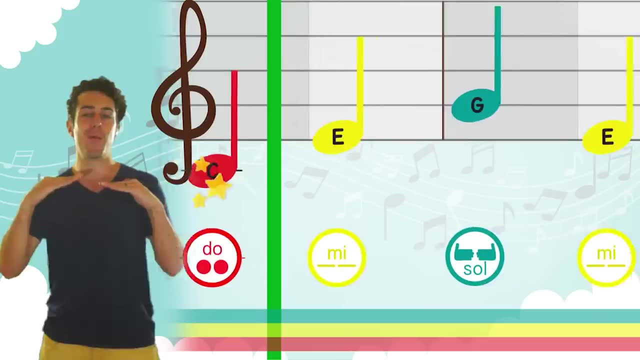 Nice job with that, everybody. Let's jump to the next song. All right, so we're going to finish up today, nice and strong, Ready Sol, do, do, do, do, mi sol, mi do Louder. 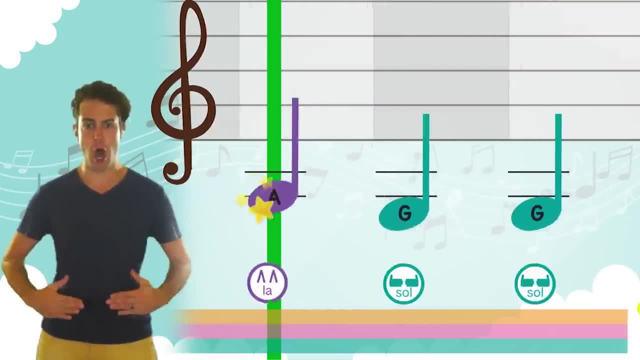 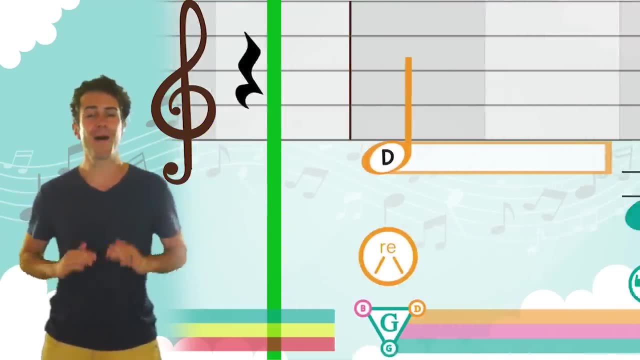 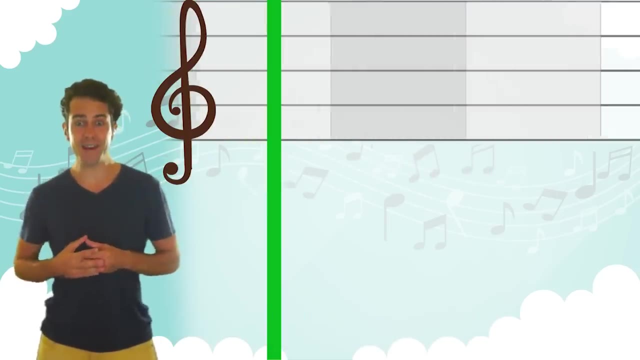 Re re re ti la sol sol do do do do mi sol mi do Re sol ti do Do. you know what song it is? It's another really distinct melody that's a little bit harder to hand sign. 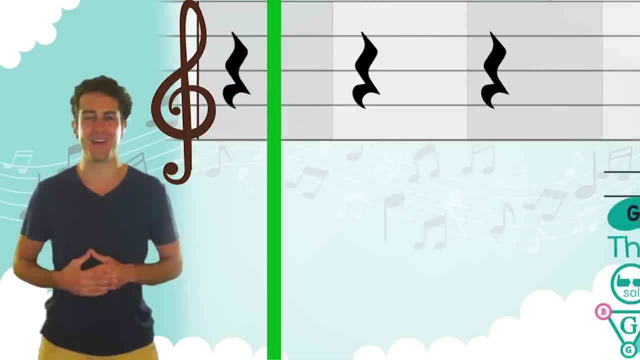 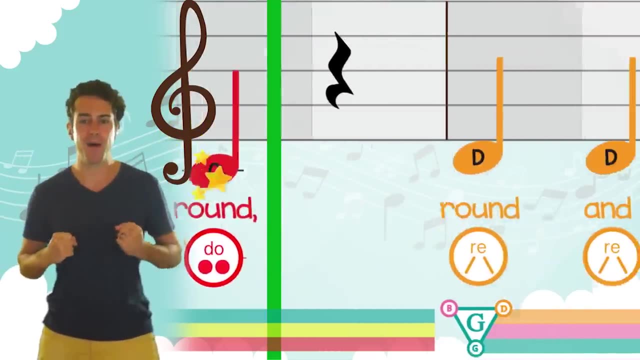 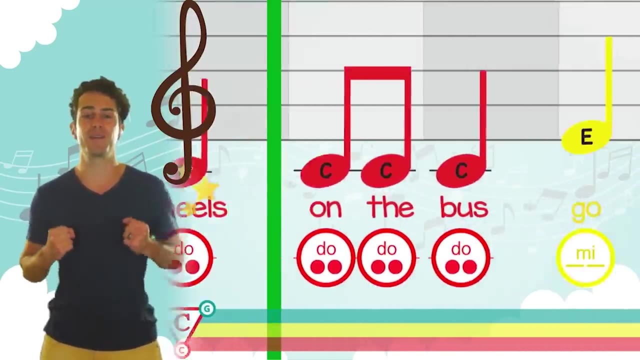 Let's add the lyrics to the wheels on the bus to finish it up. The wheels on the bus go round and round, Round and round, round and round. The wheels on the bus go round and round. The wheels on the bus go round and round. 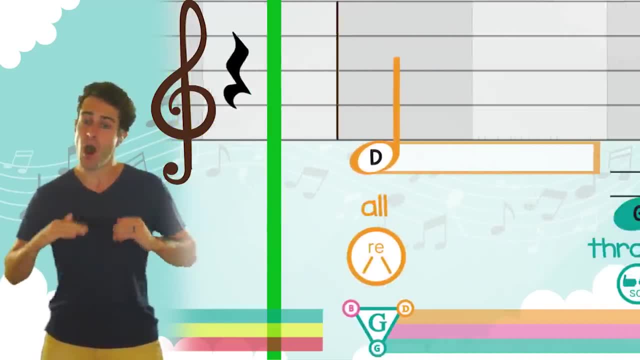 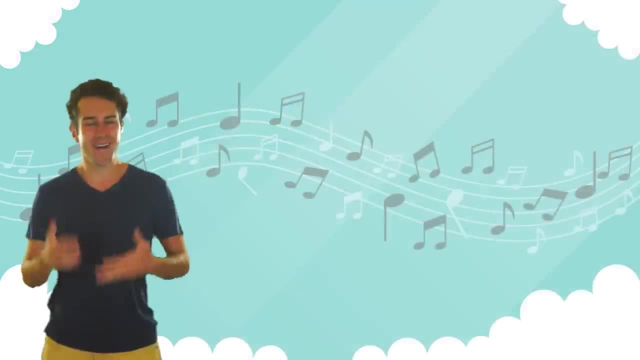 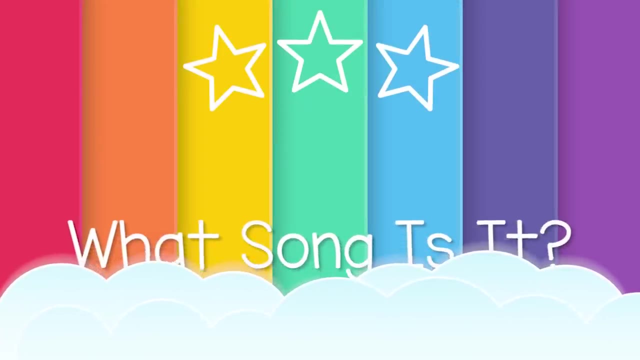 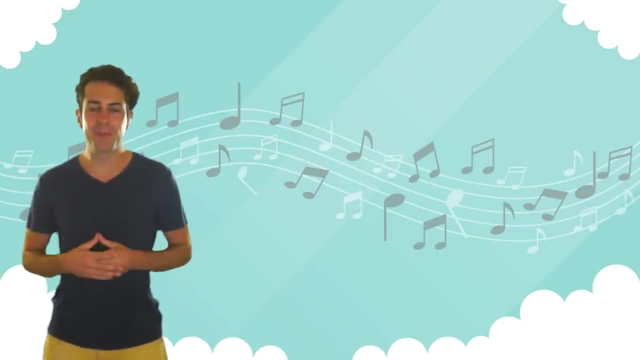 The wheels on the bus go round and round all through the town. Hey, give yourself a huge round of applause, everybody. Nice job with PSU Melodies 10, this awesomely long version of What Song Is It? We hope you had a lot of fun playing this version of What Song Is It? 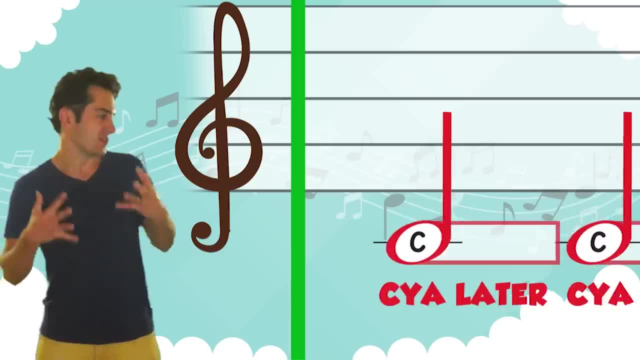 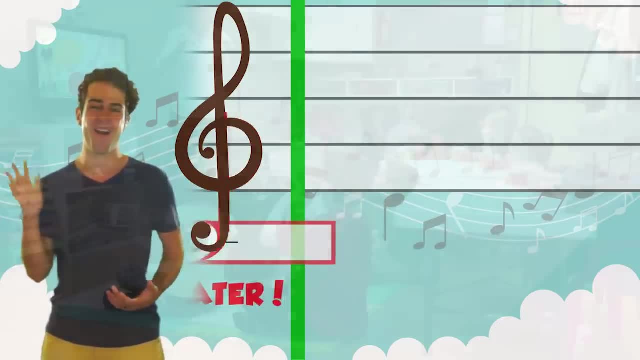 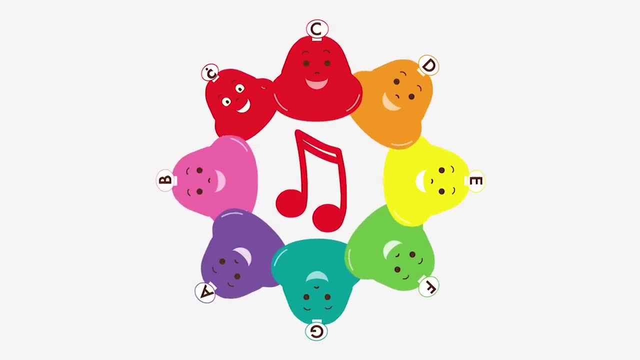 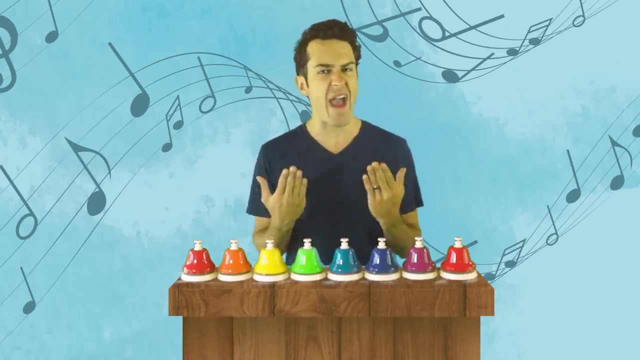 And until the next lesson, I will See you later. see you later. See ya, see ya later. The last two videos we have today are actually shorter clips from some of the more advanced rhythms that we have inside of Primary Prodigies. 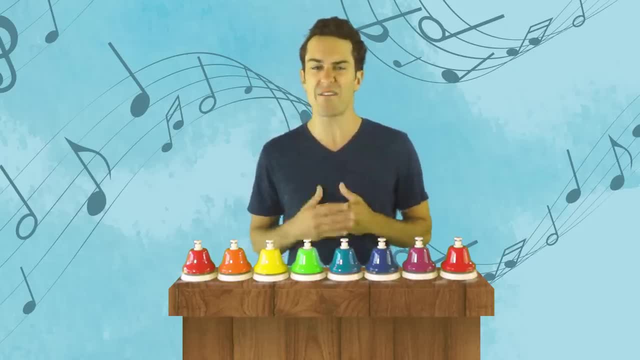 First we'll get a taste for some pizza rhythms inside of a short clip from ZaTime, and then we'll bring it on home with a final look at a more advanced version of Sweet Beats. I hope you enjoyed this little compilation. I hope you enjoy these next two little clips. 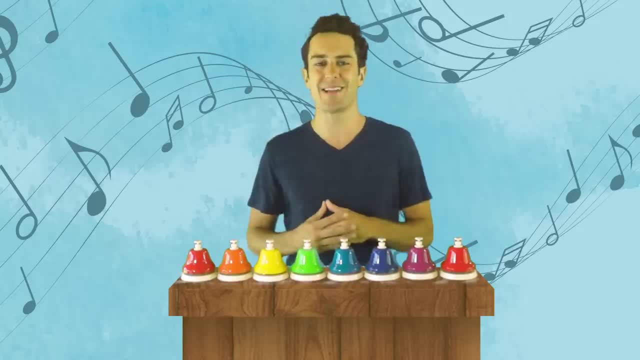 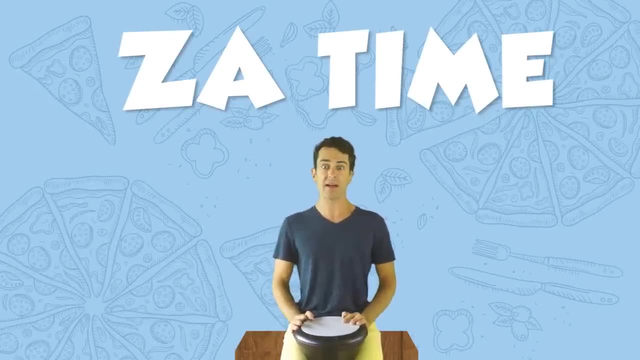 and we'll be back in a couple minutes to sing one final big see ya later. Hey everybody and welcome to Za Time. Today we're going to be playing lots of call and response rhythms using our Za's and Zee Zee's- our pizza music. 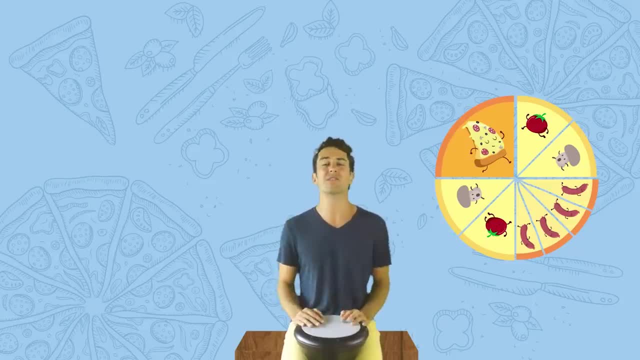 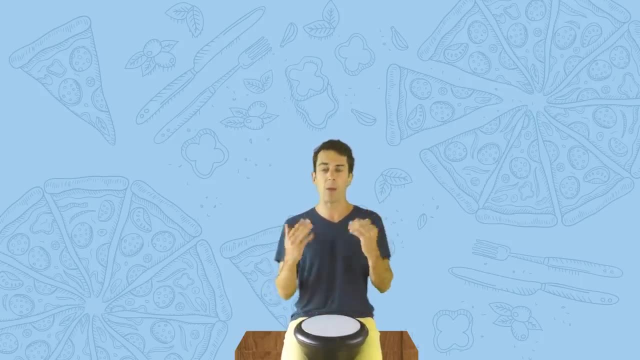 We'll also use some toppings for the pizza and we'll of course use our numbers like one and two, and to sing about our rhythms. We'll do a little tapping and clapping for the choruses and then we'll do repeating after me for the verses. 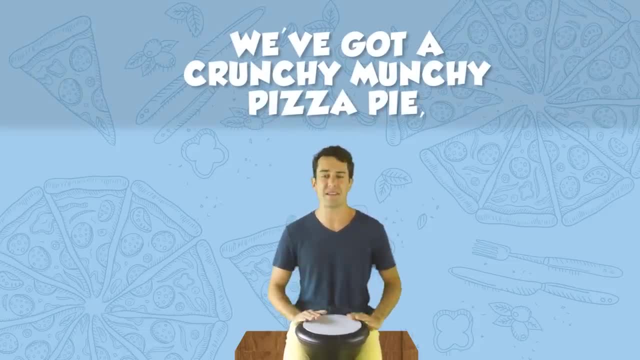 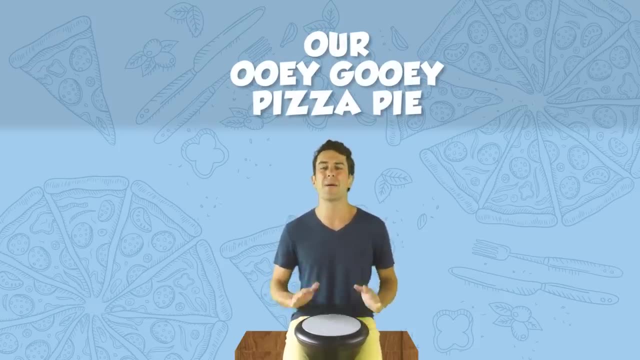 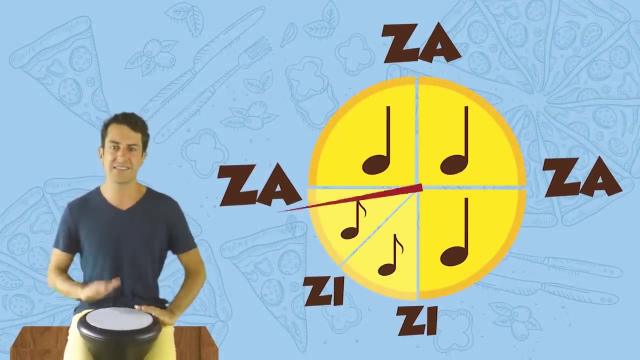 Ready. We've got a crunchy, munchy pizza pie. We'll cut it up to make a slice, Our ooey gooey pizza pie. Let's see how it divides You ready. We've got Za Za, Zee, Zee Za. 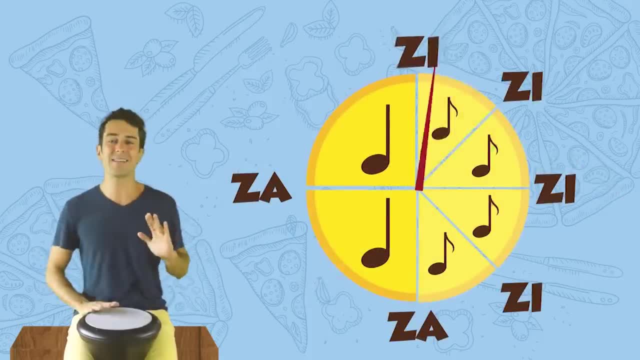 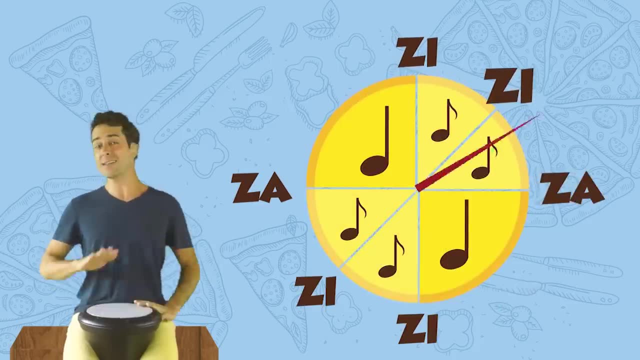 Za Za Zee. Zee Za Zee Zee Zee Za Za Zee Zee Zee Zee Za Za Zee: Zee Za Zee Zee Za. 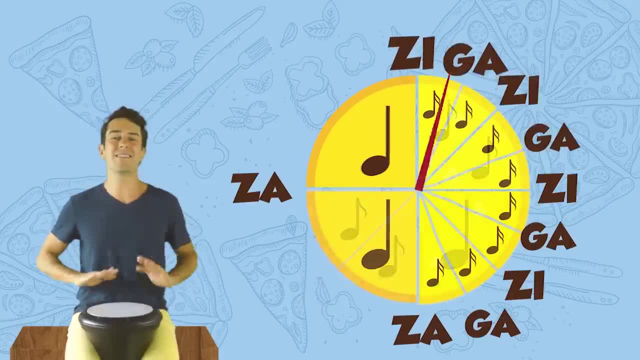 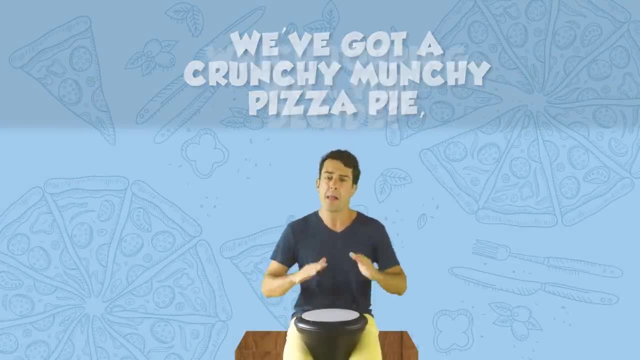 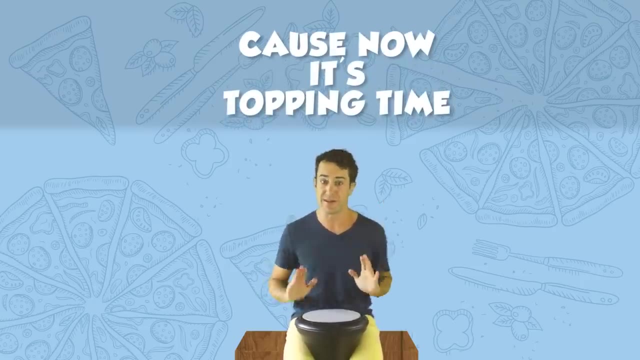 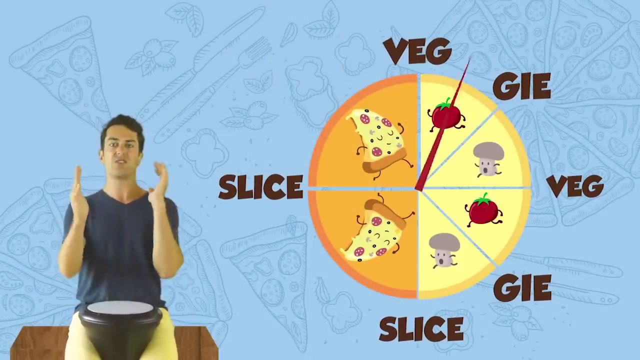 We've got a crunchy munchy pizza pie. Which toppings will you decide for our ooey gooey pizza pie? Because now it's toppings time. We've got veggie veggie slice slice. veggie veggie slice slice. 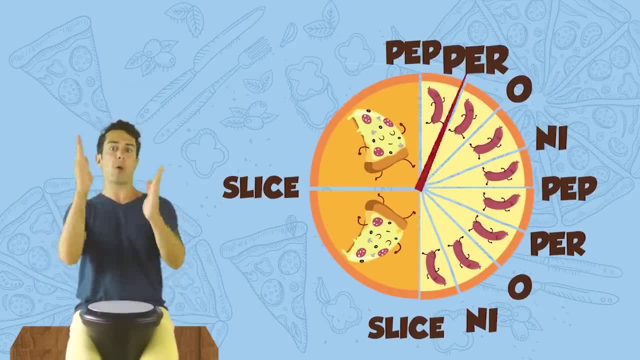 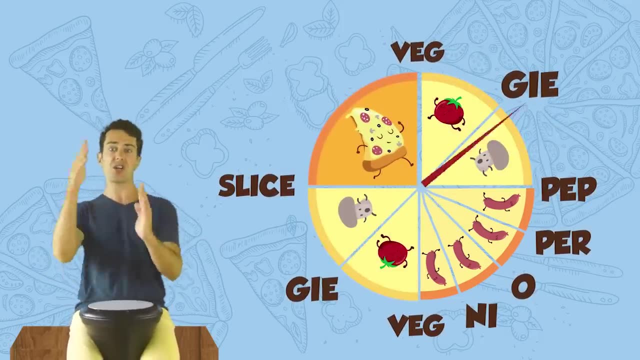 Pepperoni pepperoni slice slice. pepperoni pepperoni slice slice. Veggie pepperoni veggie slice. veggie pepperoni veggie slice. Pepperoni veggie- pepperoni slice. 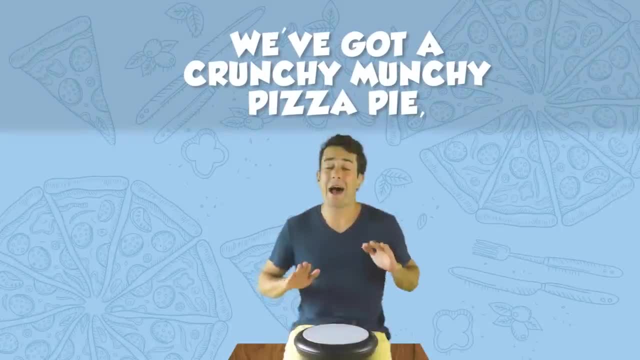 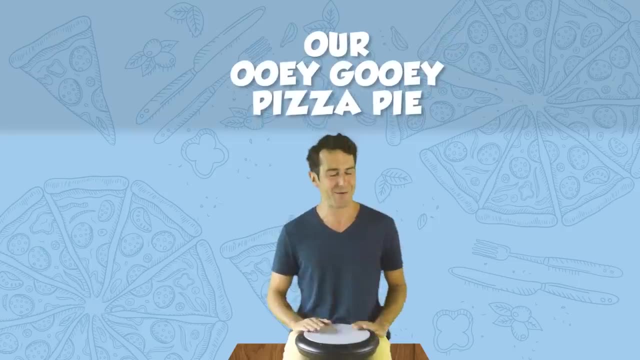 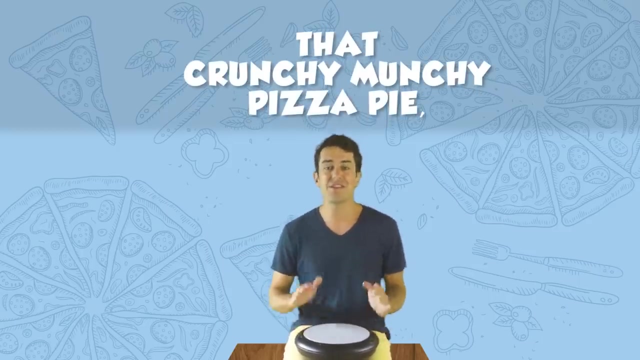 Pepperoni veggie slice, slice, slice. We've got a crunchy munchy pizza pie. We cut it up to make a slice, Our ooey gooey pizza pie. Let's see how it divides That crunchy munchy pizza pie. 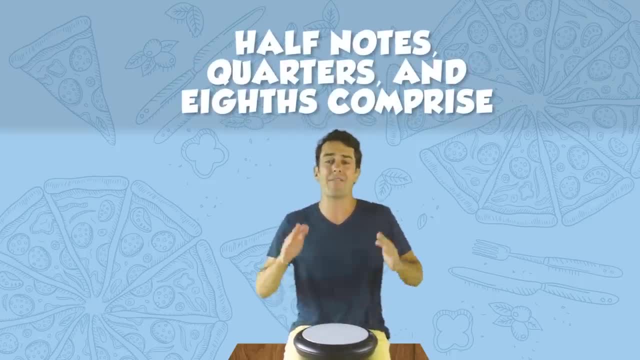 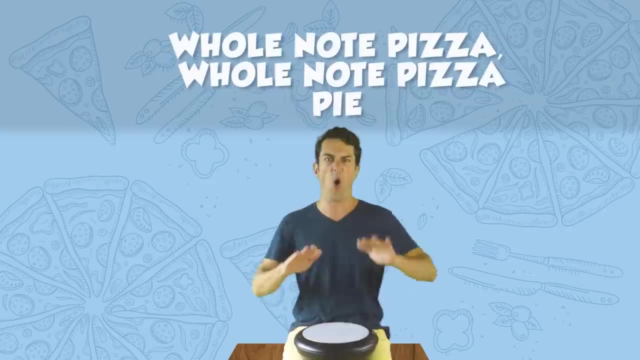 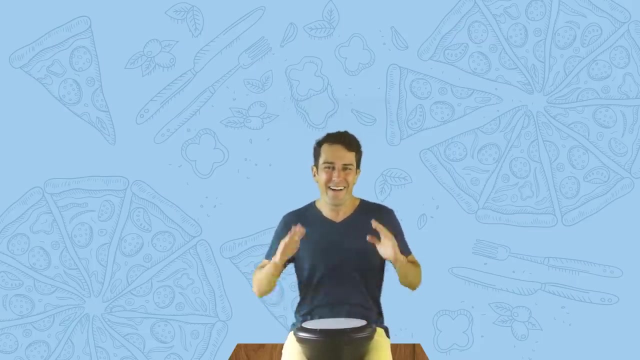 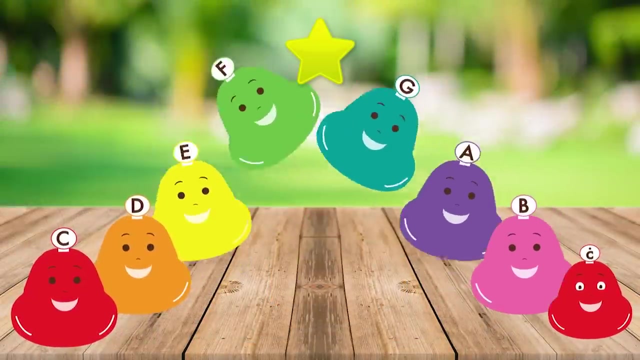 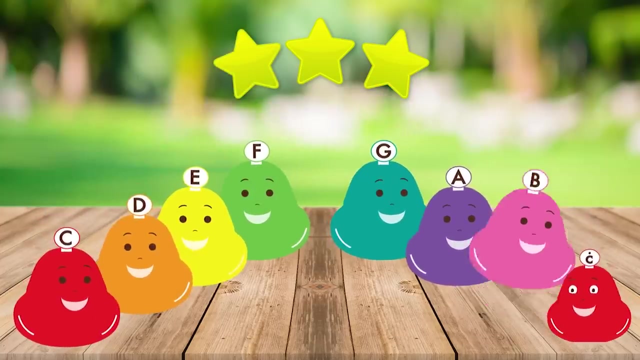 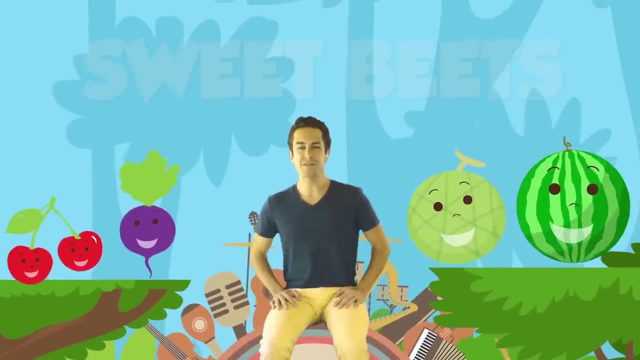 Now we know how it divides: Half notes, quarters and eighths comprise Our whole note Za whole note Za whole note pizza pie. Give yourself a huge round of applause. Excellent work with the pizza rhythms. everybody, Hey everybody, and welcome to Sweet Beats. 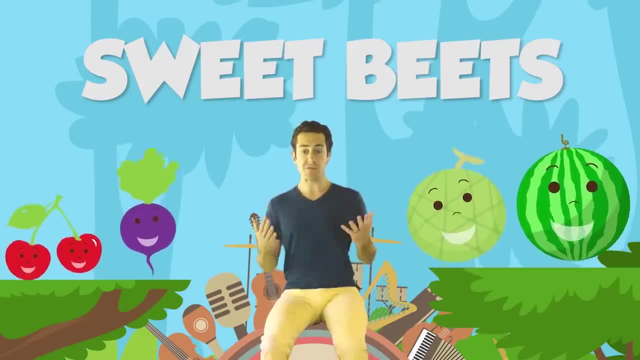 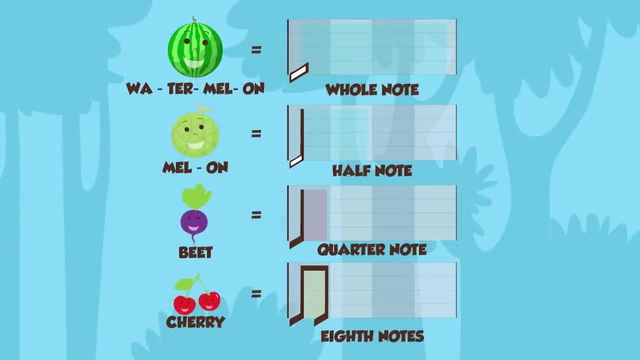 Sweet Beats is a call and response rhythm game and we're going to use some fun fruits and vegetables to talk about our whole note, our half note, our quarter notes and our eighth notes. We're going to play some call and response, so you'll do a lot of repeating after me. 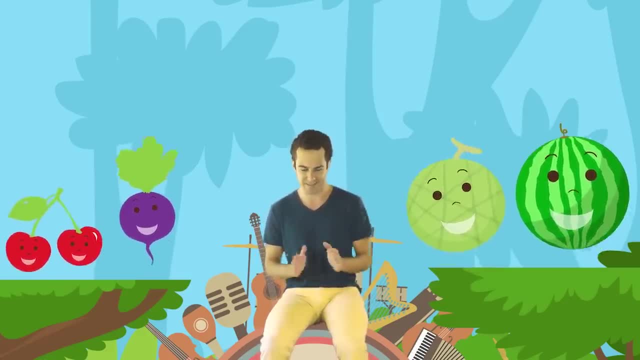 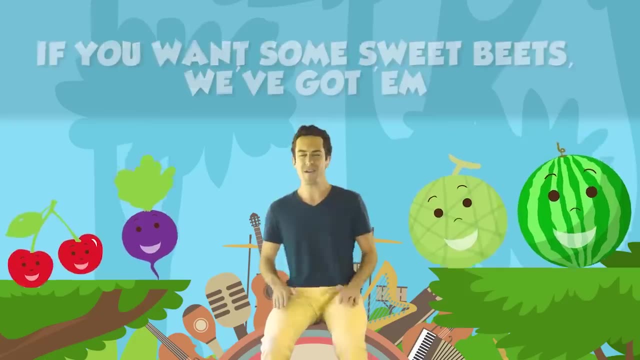 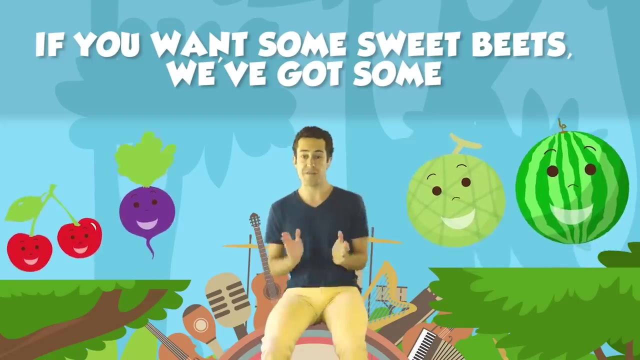 and we'll start out by tapping and clapping, just like this. The song goes like this: If you want sweet beats, we've got some. If you want some sweet beats, we've got them. And if you want some sweet beats, we've got some. 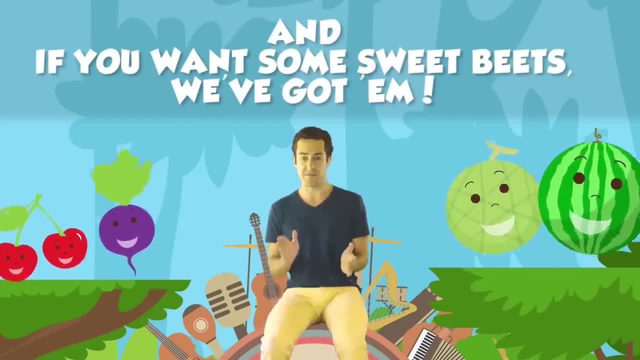 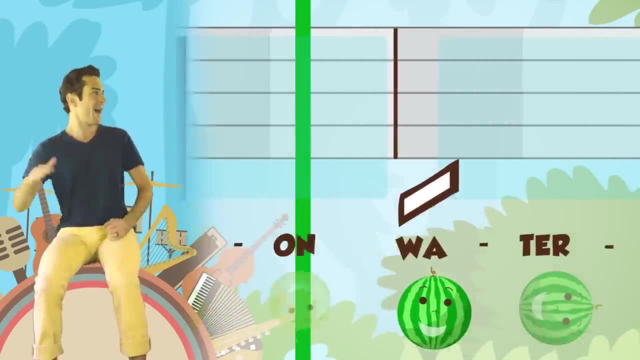 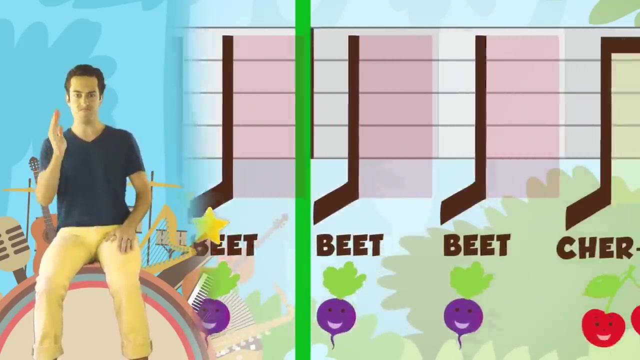 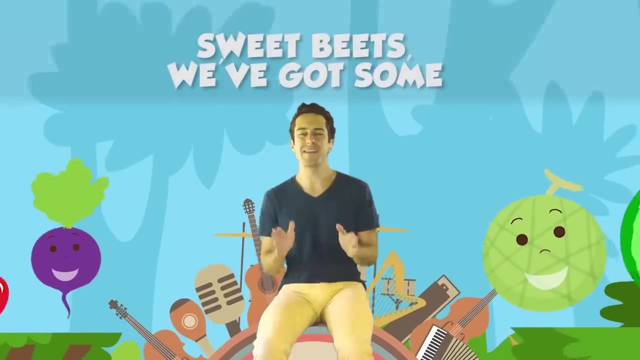 And if you want some sweet beats, we've got them All right, so repeat after me: Beet beet melon, Watermelon, Nice Beet beet, cherry, beet, Melon, beet beet, Sweet beats, We've got some. 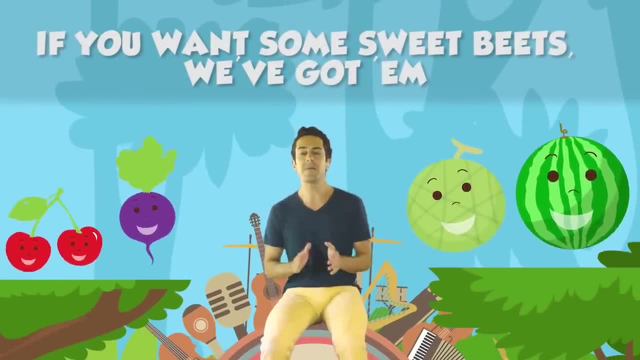 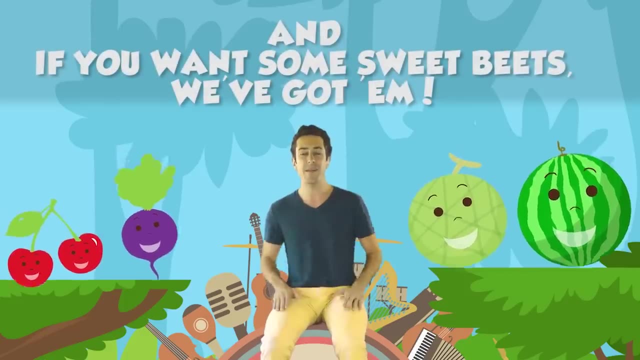 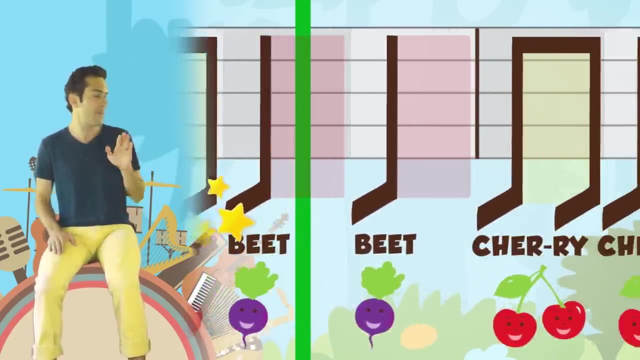 And if you want some sweet beats, we've got them, And if you want some sweet beats, we've got some, And if you want some sweet beats, we've got them. With those fruits again, we've got cherry, cherry, beet, beet. 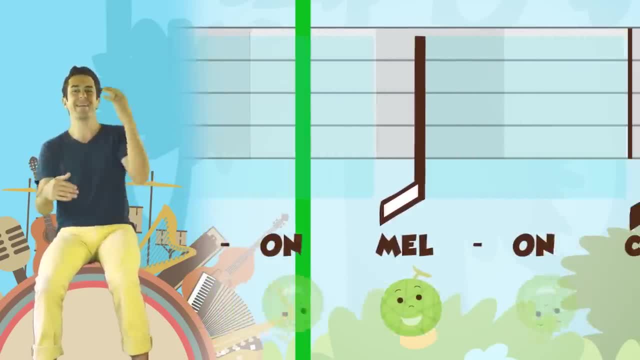 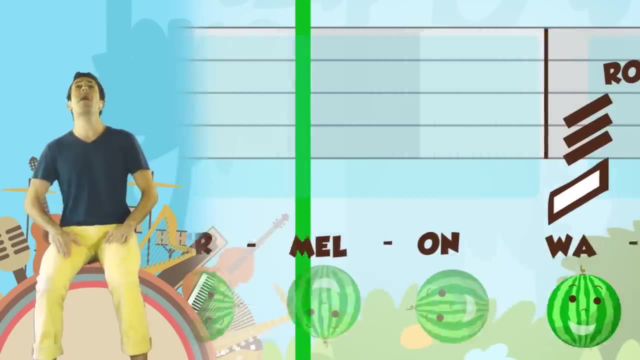 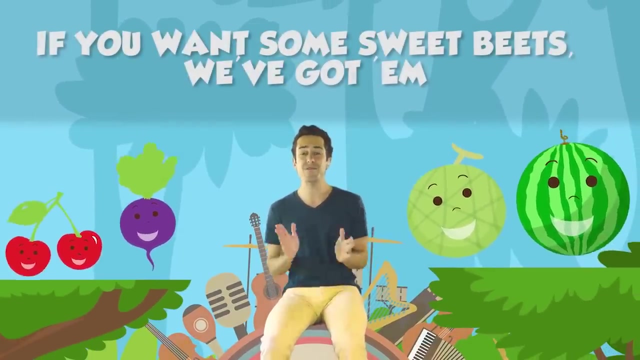 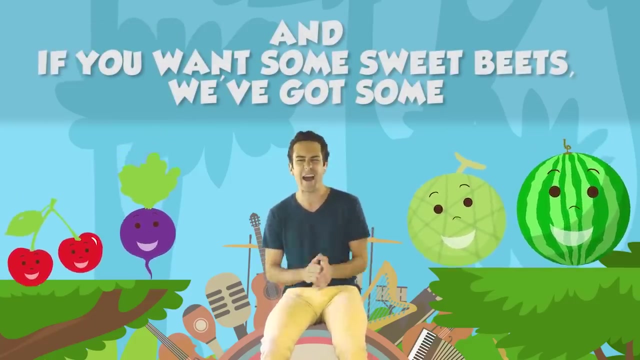 Yeah, melon, melon, Cherry beet, cherry beet, Watermelon, Sweet beats, we've got some. And if you want some sweet beats, we've got them. And if you want some sweet beats, we've got some. 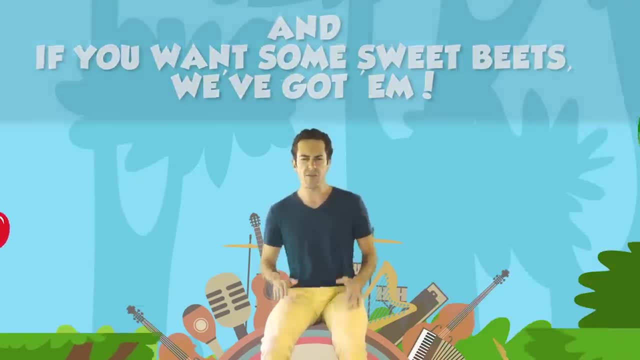 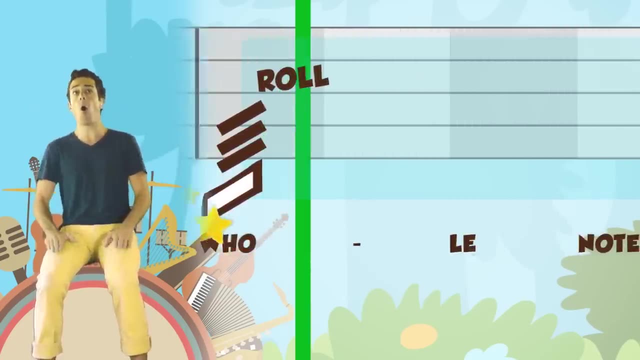 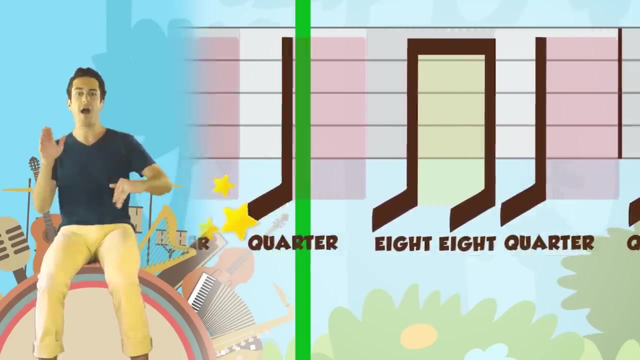 And if you want some sweet beats, we've got them With the names of the notes. quarter quarter: half note. Quarter quarter half note. Whole note Four: note four note Quarter quarter eight: eight quarter. 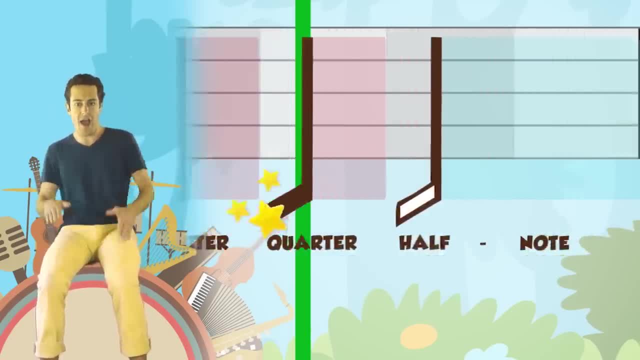 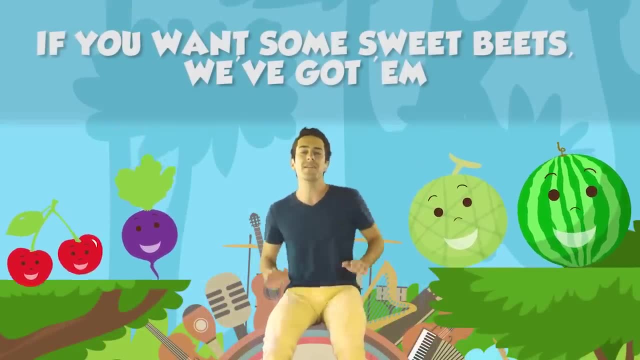 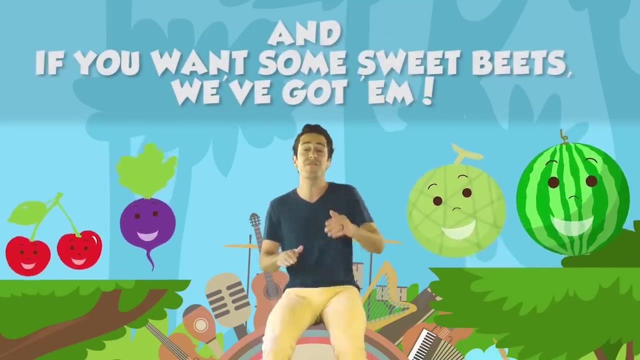 Yeah, quarter, quarter, half. note: Sweet beats, so we've got some. And if you want some sweet beats, so we've got them. And if you want some sweet beats, so we've got some. And if you want some sweet beats, we've got them. 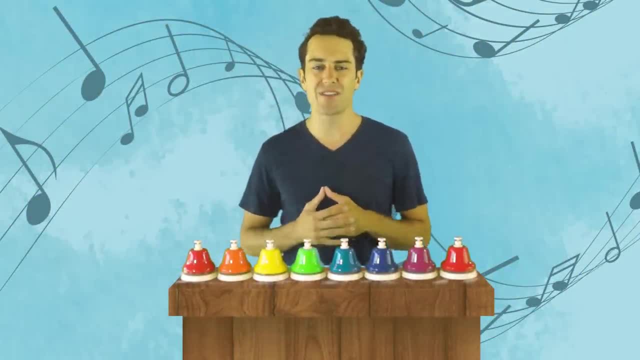 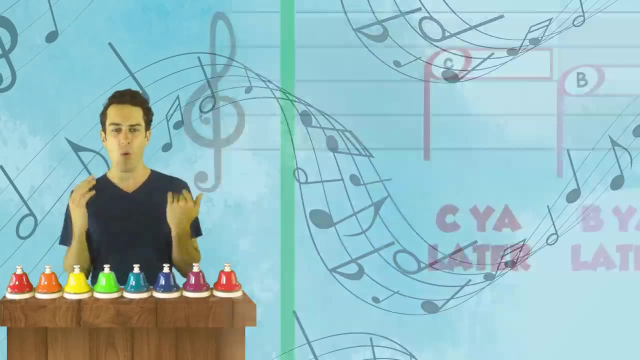 Hey, so nice work with all those different lessons from the Prodigy's Playground. We covered a lot of different things today. I hope you had a lot of fun. Until the next time I will see you later. be you later, A you later, D you later. 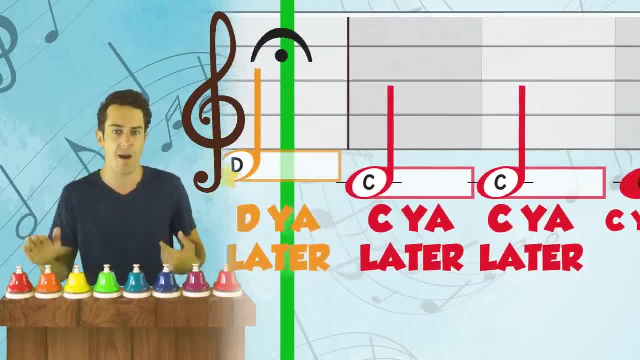 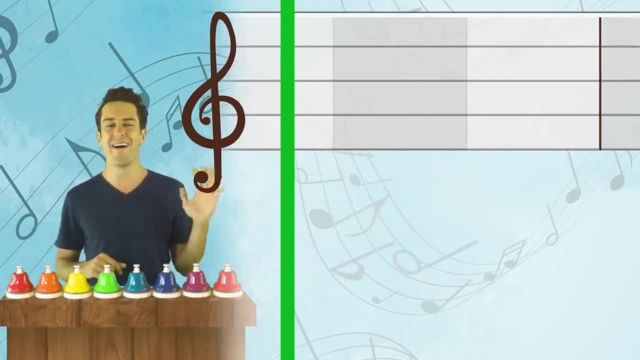 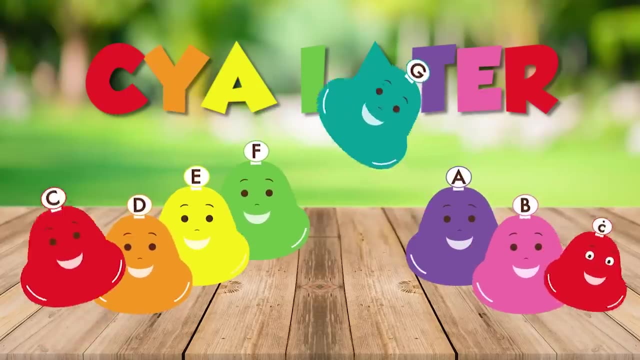